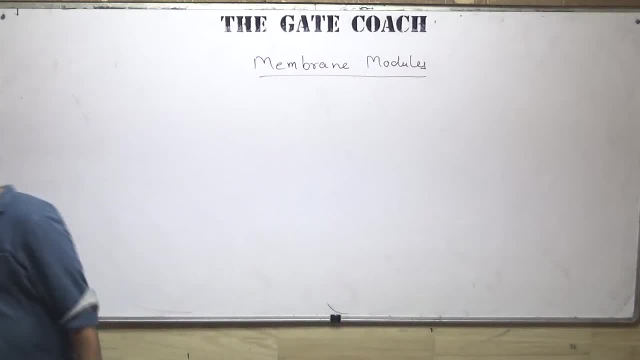 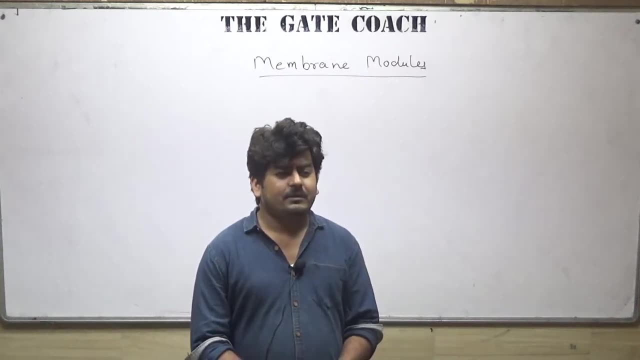 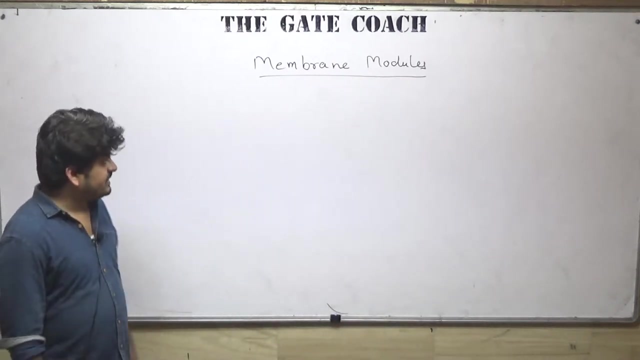 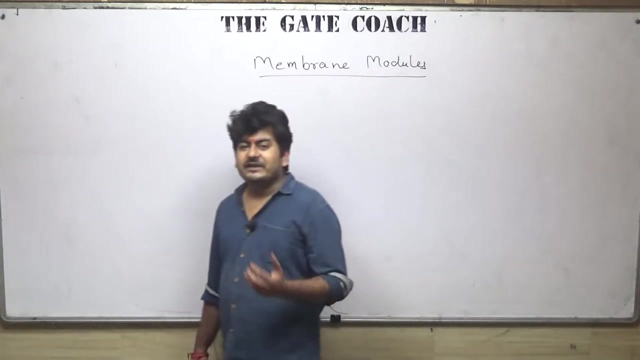 Okay, So that will be a surprise for all of you And surely we will go – that surprise you will get from the next lecture. Okay, And here today we are in third lecture. We will discuss the membrane. If you remember, in the last lecture we discussed about the materials used for the membrane. 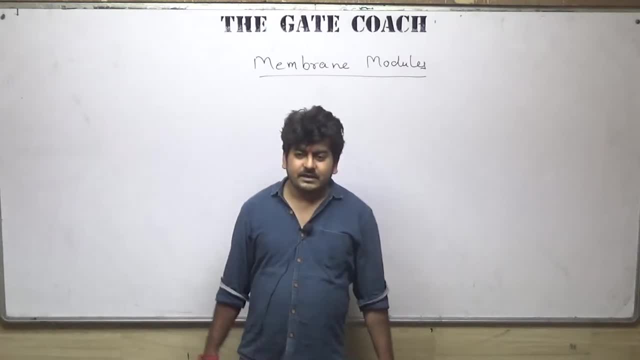 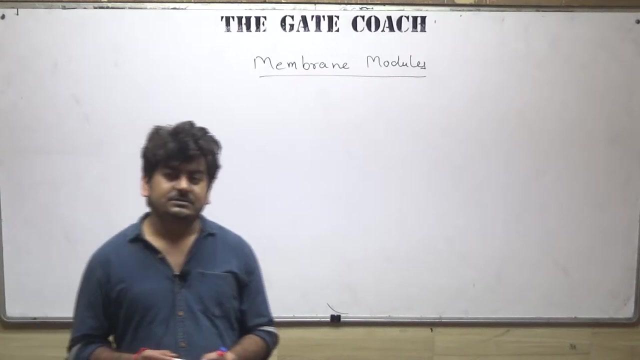 preparation, membrane manufacturing. like polymers, what kind of polymers we use? the natural and synthetic polymers, their characteristics, and I have shared the handout on our telegram group for that. You can join our telegram group to get the handouts on these lectures. 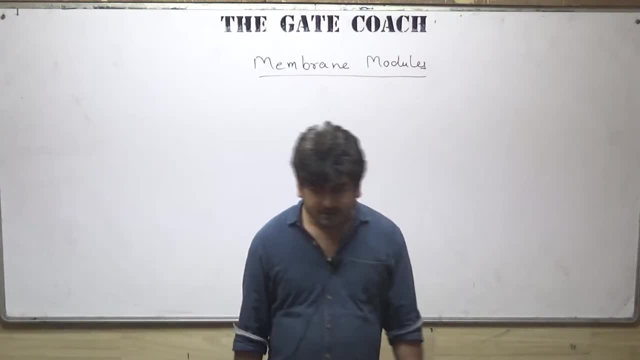 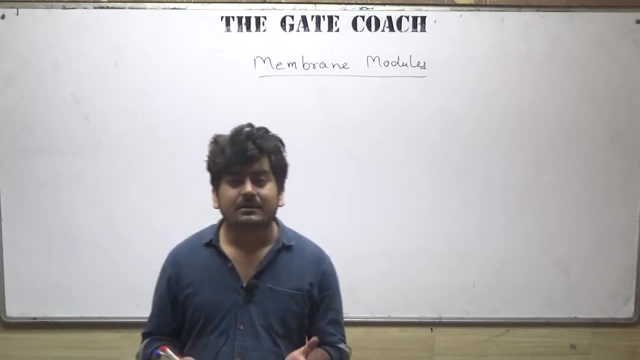 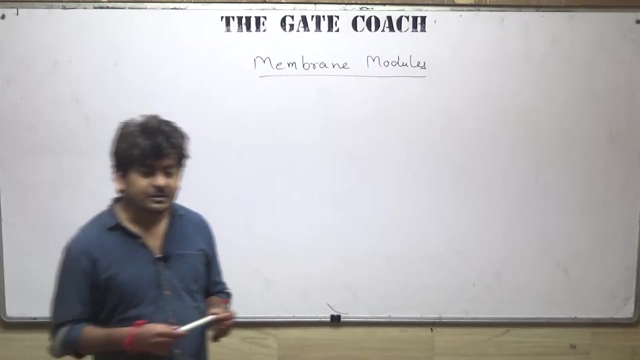 Today, in this third lecture, we will discuss about the membrane modules. So if I talk about the modules- modules, basically here we will talk about membrane- only the working, the mechanism in membrane means: how can we classify the membrane? what kind of membranes are used, the flow patterns, transportation of solutes. 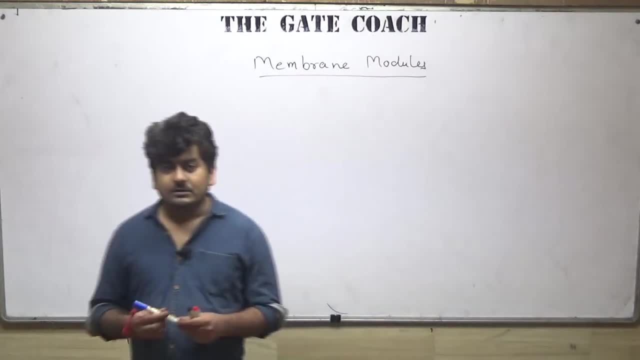 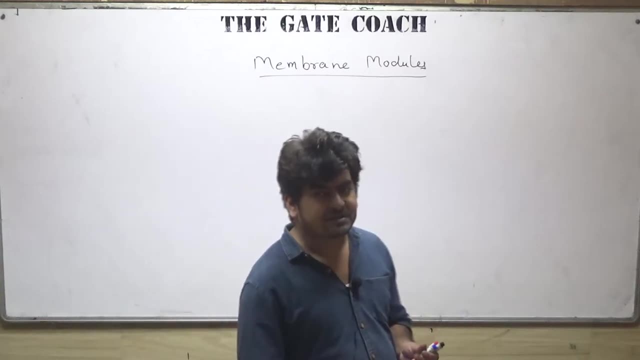 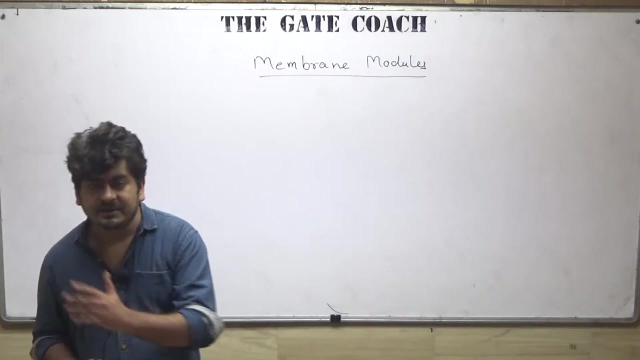 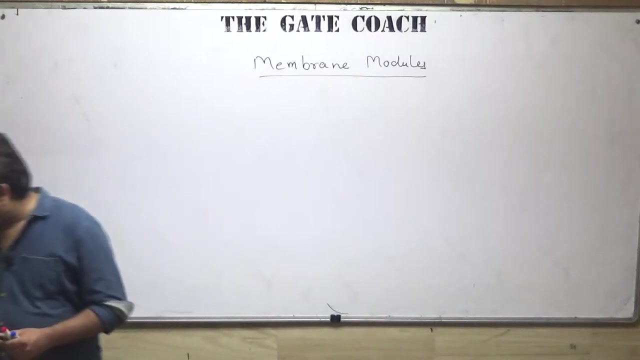 As we discussed, membranes are used to allow the selective transport to some of the constituents or one of the constituents present in the mixture. So how that constituent will move, will transport through the membrane in the permeate phase? all these things we will discuss in this lecture. 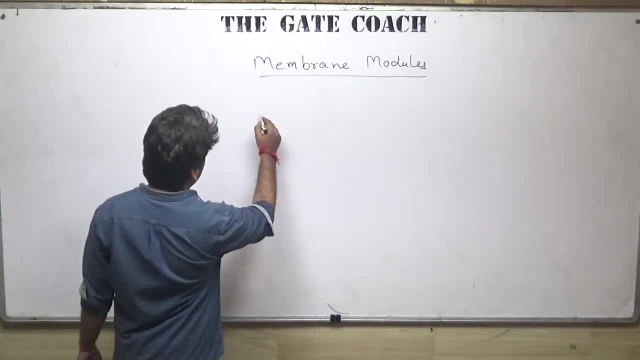 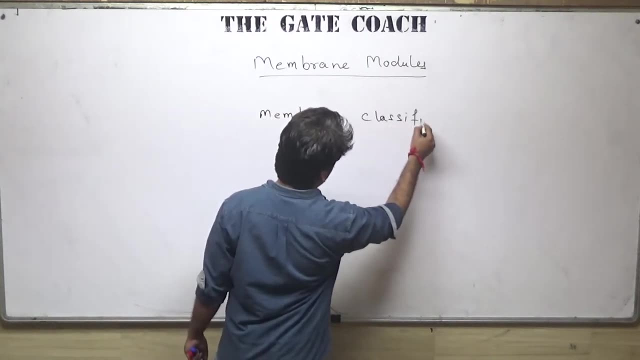 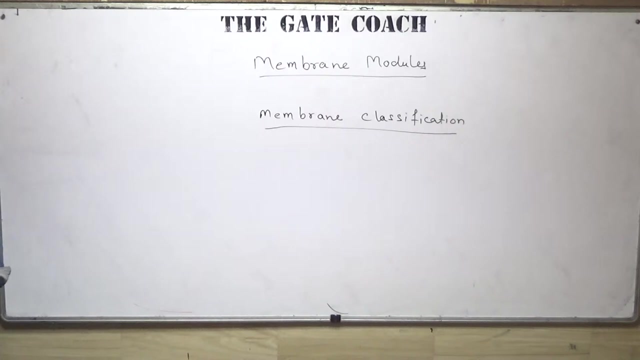 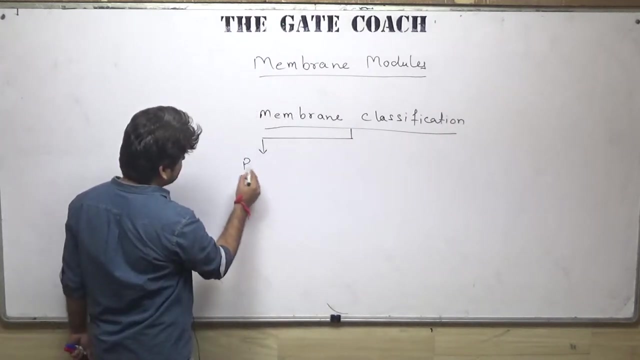 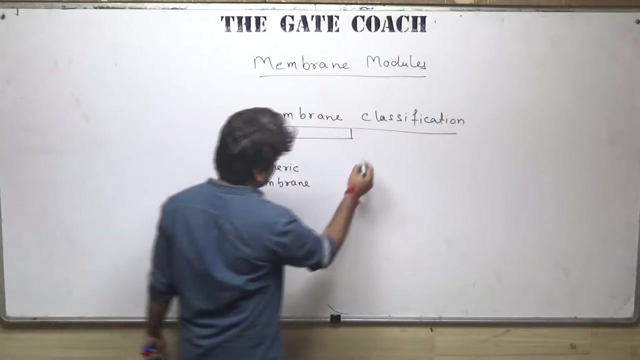 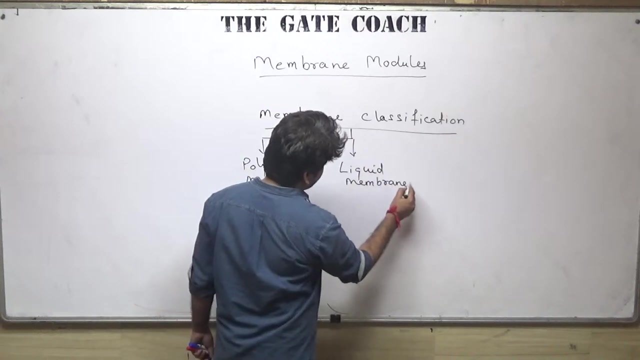 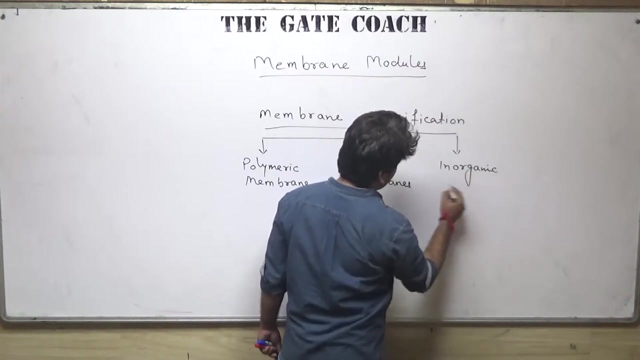 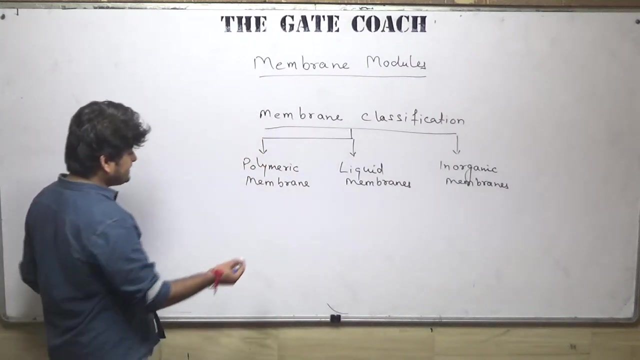 So, first thing, I am again repeating the membrane classification So that we can understand this in a better way. So here we can classify the membranes into three categories: Polymeric membranes, Liquid membranes And polymers And polymers- inorganic membranes- where we can classify these polymeric membrane into. 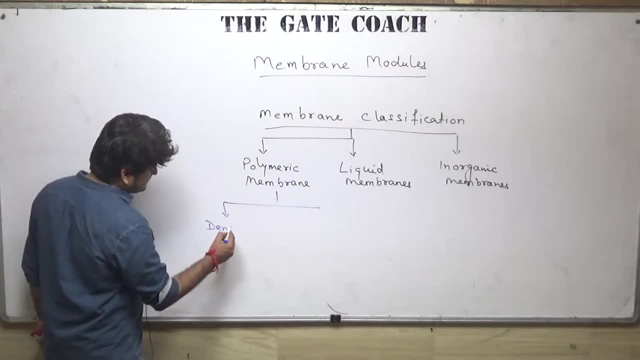 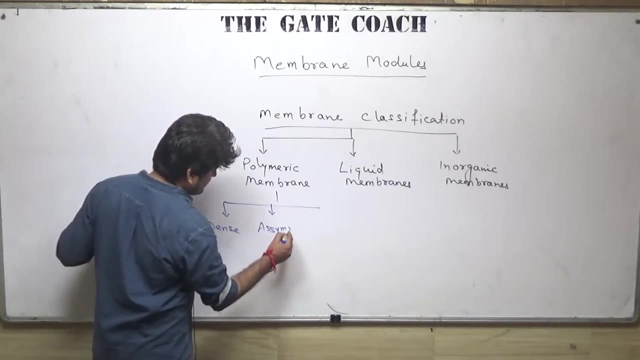 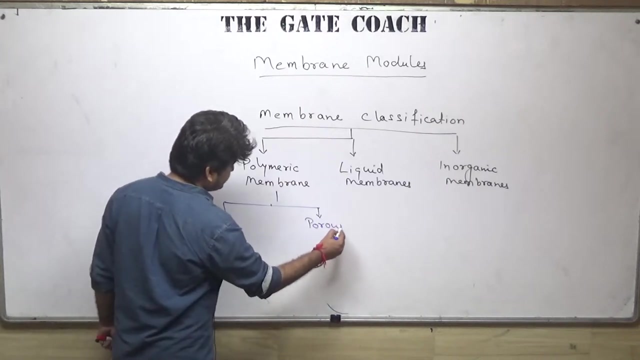 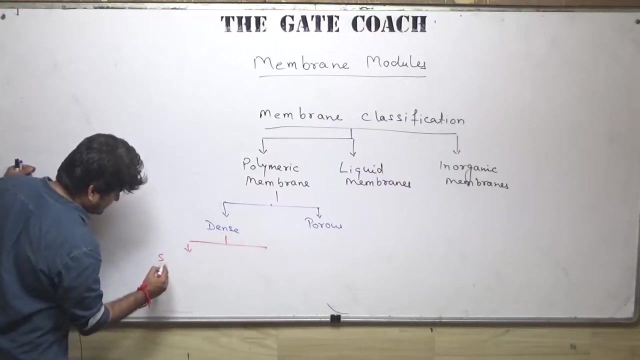 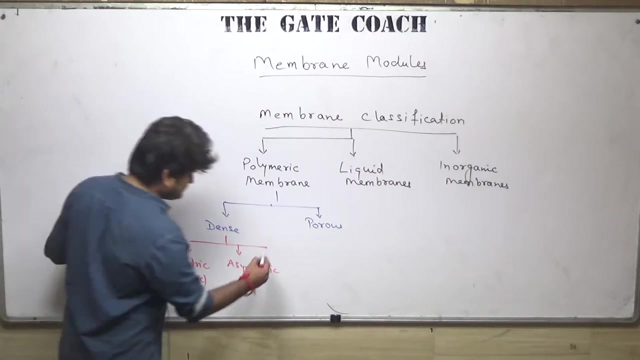 three categories. further, dense polymer membrane- asymmetric polymer membrane- asymmetric- comes in the dense category. actually, we can classify this into two parts only: dense and porous. okay, further, this dense membrane can be classified into three categories, where one is symmetric, also known as isotropic. second is asymmetric, also known as anisotropic. 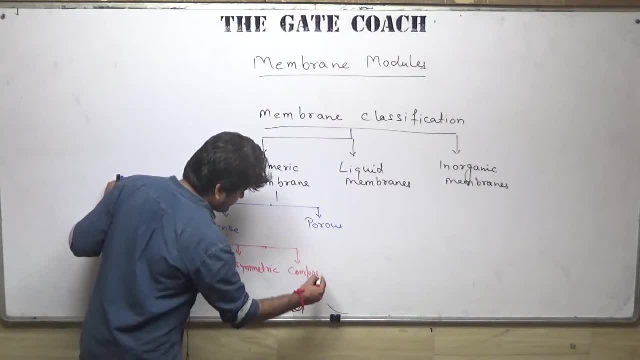 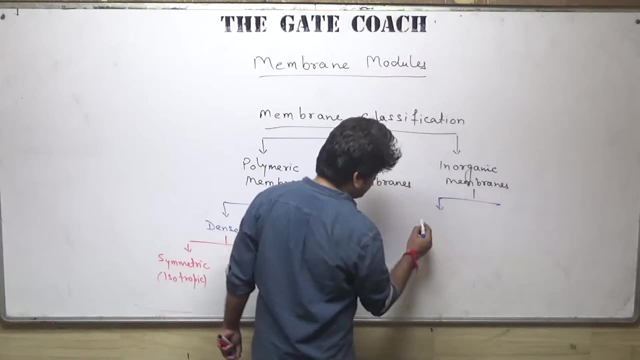 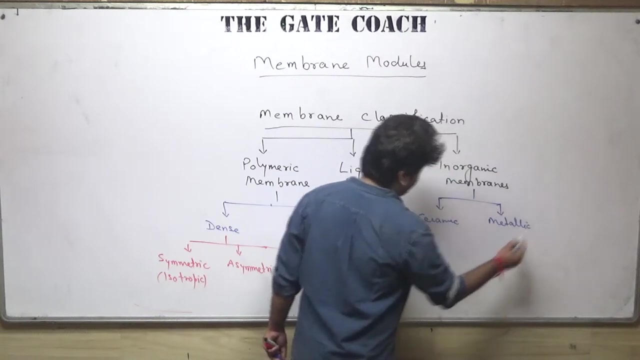 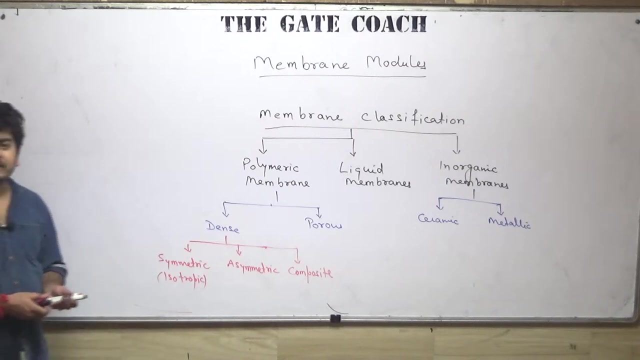 and the third one is composite membrane, where these inorganic membranes can be classified into two categories: ceramic and metallic. okay, so we will talk about each of them, their function, they are working, their application and then that how the transportation takes place in each of the following membrane. so first we will talk about the dense membrane. 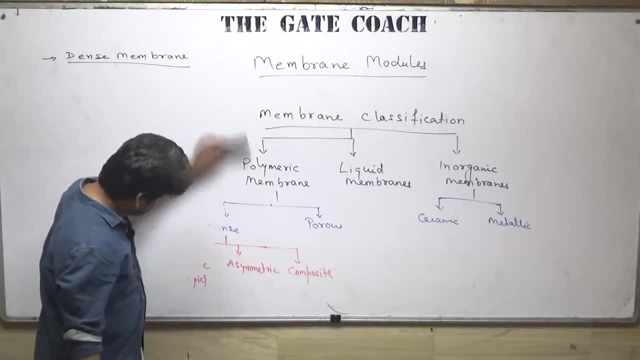 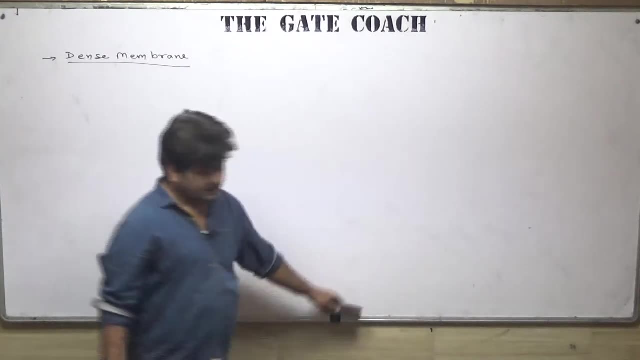 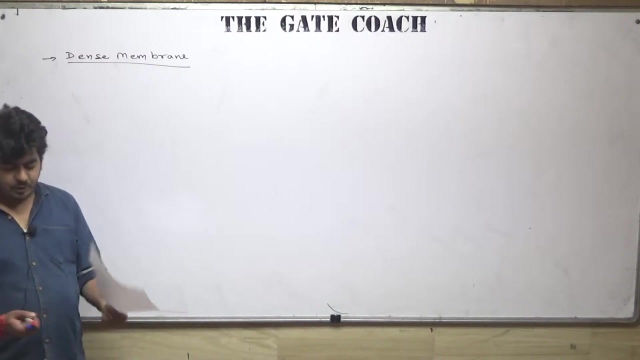 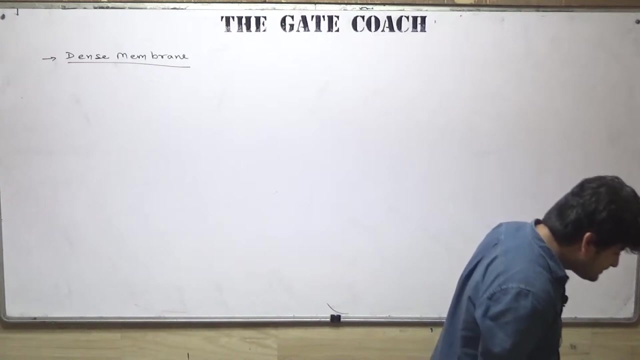 we discussed the same thing in the first lecture as well. So, guys, if we talk about the dense membrane, I have prepared some important key points for all of you. okay, so that we can understand this. What surprise, sir Swarup Kumar. the link of the telegram group will be available in. 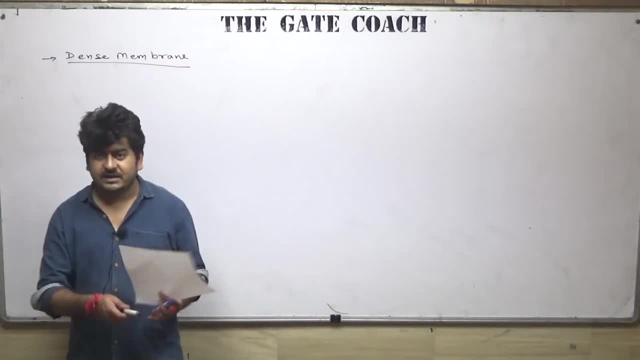 the description and in the comment section of the same video after this lecture will end. So, guys, you can see that link in the previous lectures, lecture 1 and 2,. okay, The surprise. I am sure you will like that surprise okay. 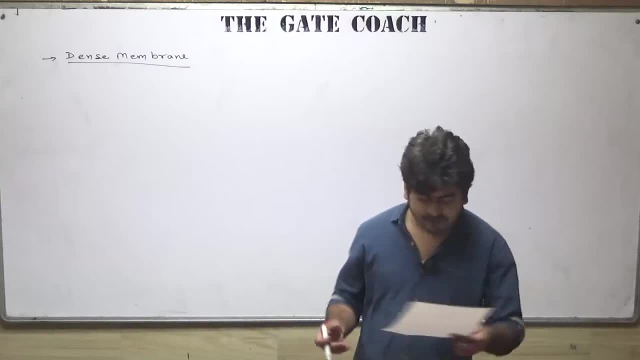 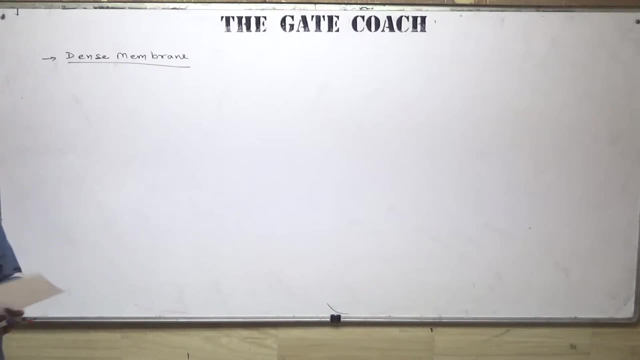 We were busy in that thing as well. that's why we were not able to be live. So, if I talk about the dense membrane, so, guys, there are few points which you should know, okay. Dense membrane, also known as non-porous membrane. 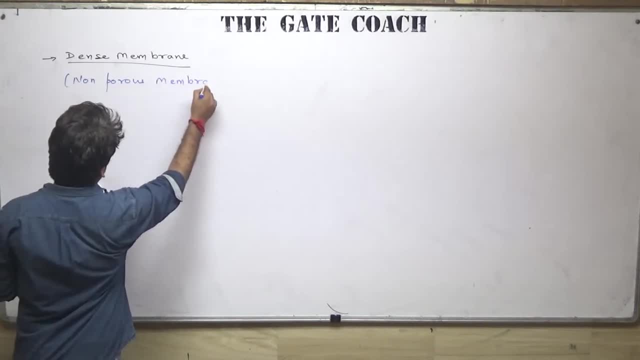 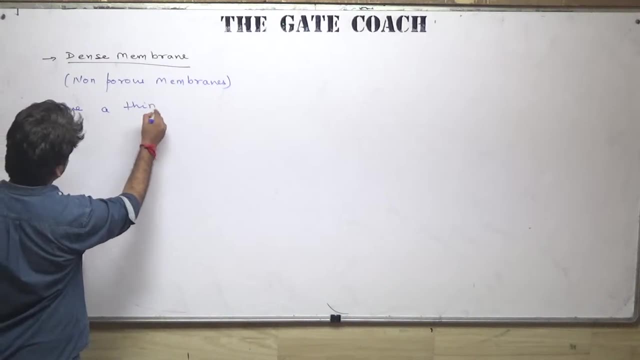 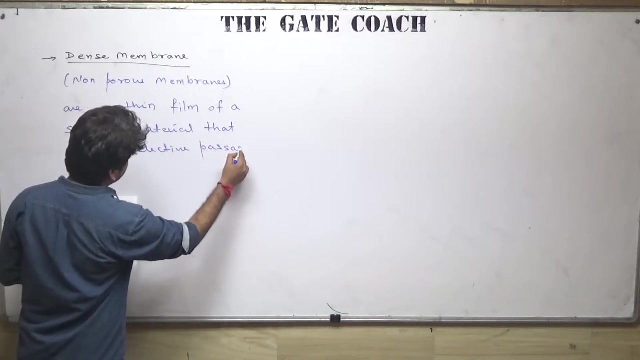 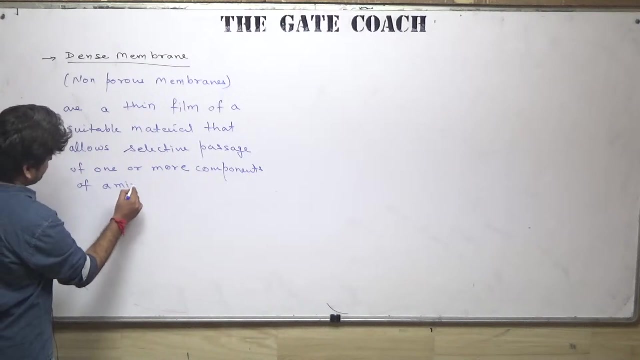 Are a thin film of a suitable material that allows a thin membrane to be able to stretch. Okay, Okay, Okay. selective passage of one or more components of a mixture. now the question is how it will allow the selective passage, what, how molecules will transport through the dense membrane. so just understand that in the dense 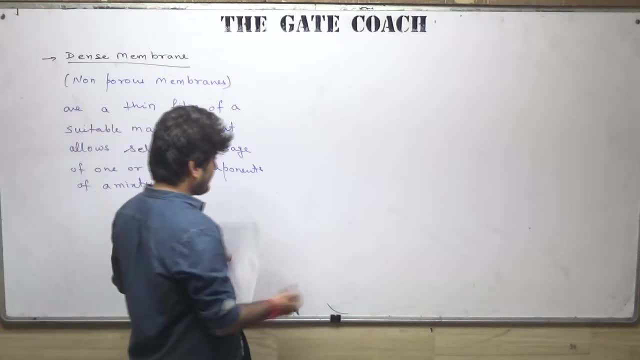 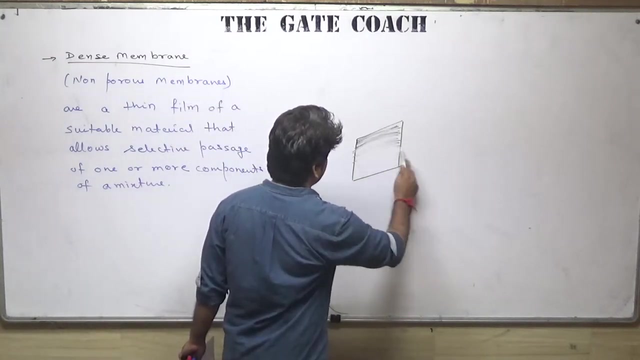 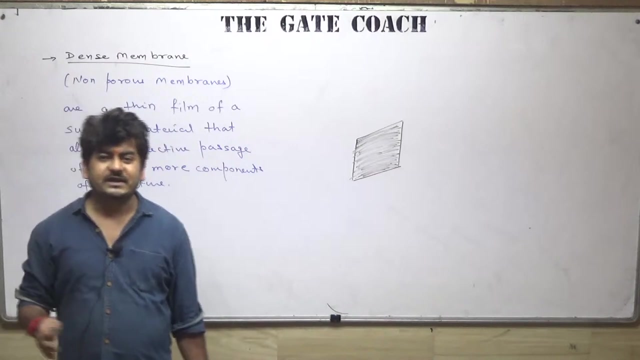 membrane. if I draw the diagram, suppose this is some dense membrane. it is almost non-porous. non-porous, I mean, you understand, there is no empty space inside the membrane. okay, just like a thick, solid. you can understand a solid plate. from one side we send the feed particles and from other side we are. 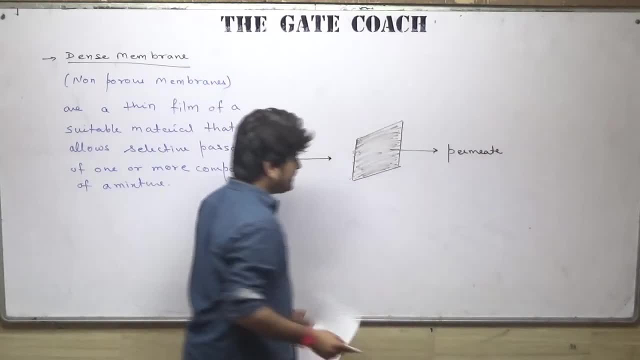 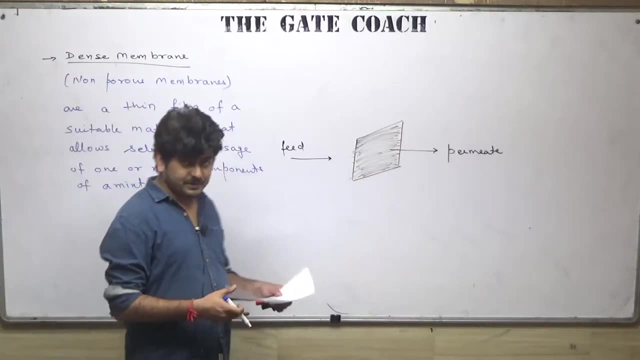 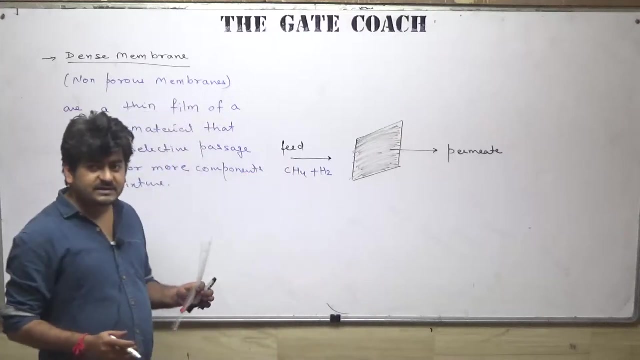 supposed to get the permeate? okay, so if I take one example, so suppose you have a membrane like this, and if you have a membrane like this and you have, that is one live example. okay, experimental example- if we pass a mixture of CH4 and H2 through this dense membrane, then what will happen? okay, 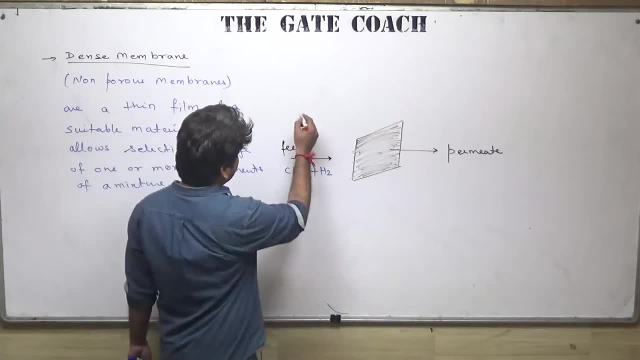 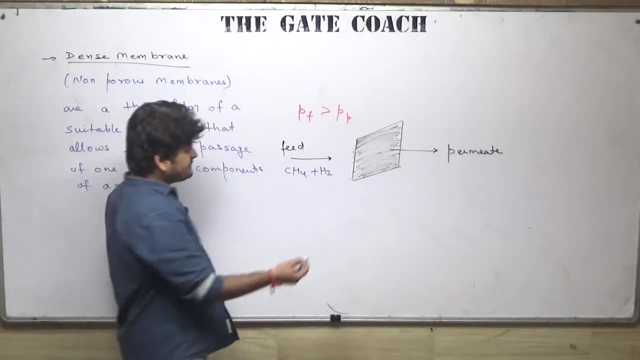 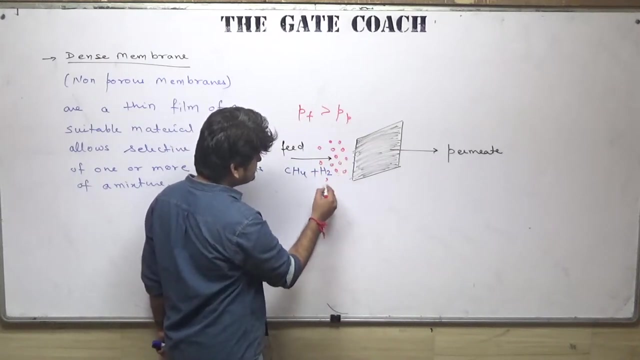 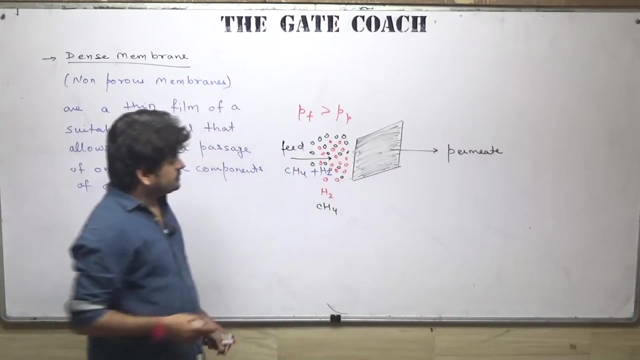 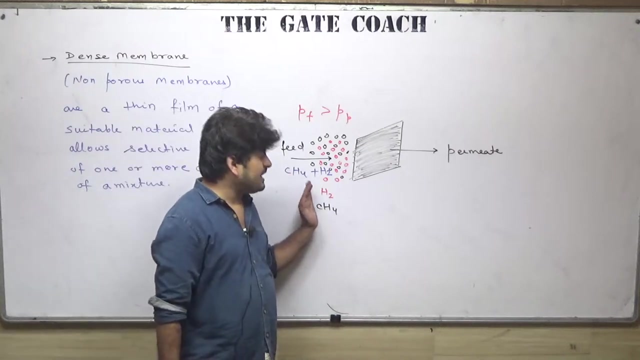 under the driving force of pressure. there the pressure of feed side is greater than the pressure that of an on the permeate side. so suppose we have hydrogen molecules in red color on this feed side and some methane molecules, suppose methane molecules are in black. so the size of this or that this dense membrane will be like these hydro it is, it will. 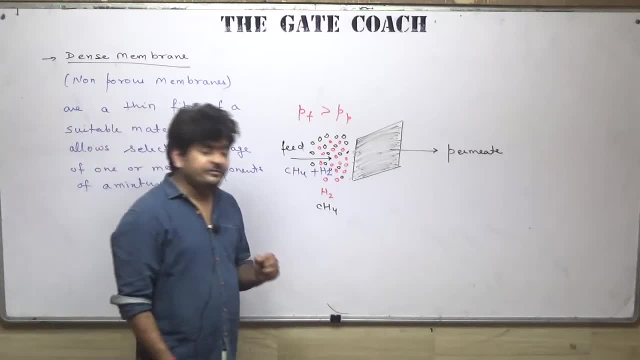 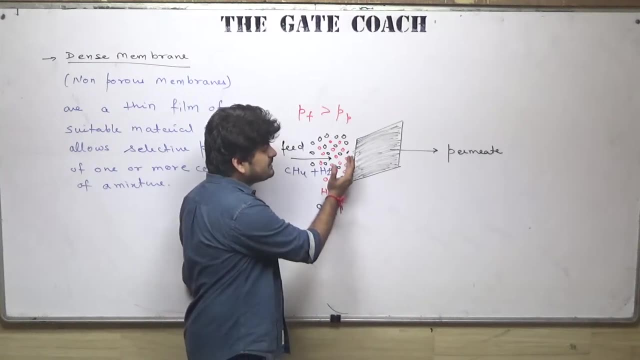 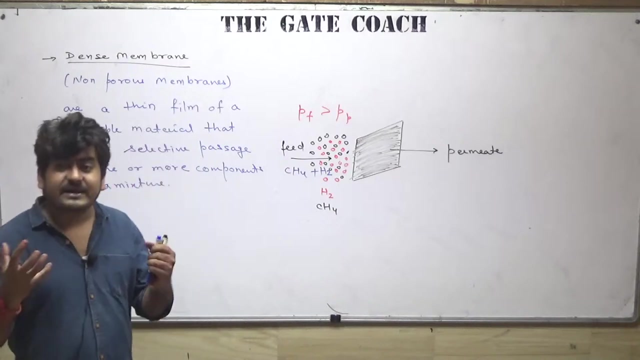 allow only the hydrogen molecules to pass. so what will happen? these hydrogen molecules? hydrogen molecules will pass through this membrane and this is the way that the hydrogen molecules will absorb in on this membrane. absorb means you can say, just like they are getting dissolved, okay, they are getting dissolved. 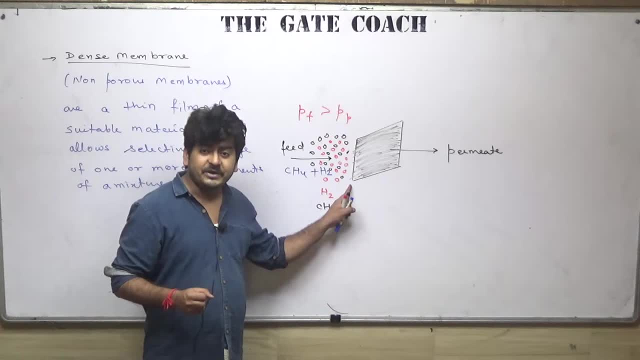 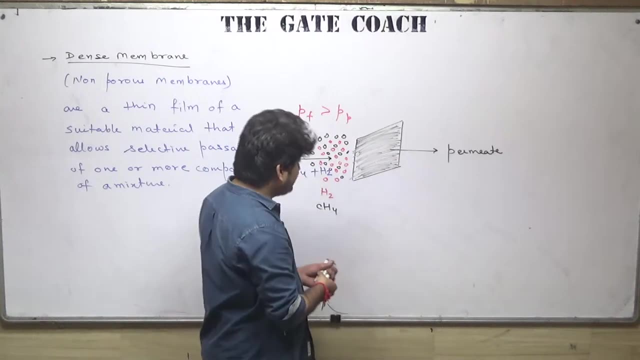 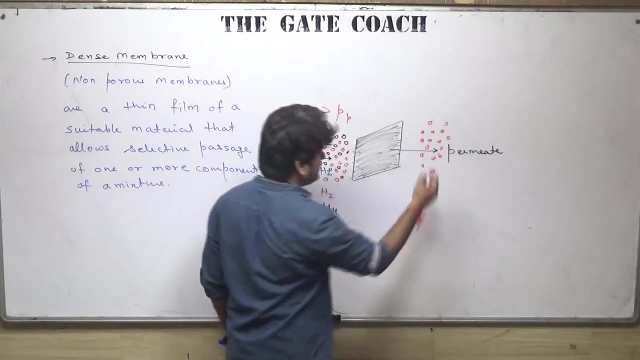 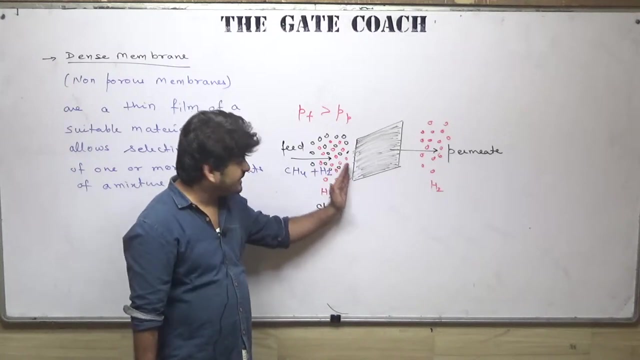 in the on this side of the membrane and they will diffuse through the membrane till this opposite side of the permeate side and then they will leave here. okay, that's not YNplnesmfbnfw. hey, hung into frjочкиde. hydrogen molecules are getting absorbed, getting dissolved on this side of the. 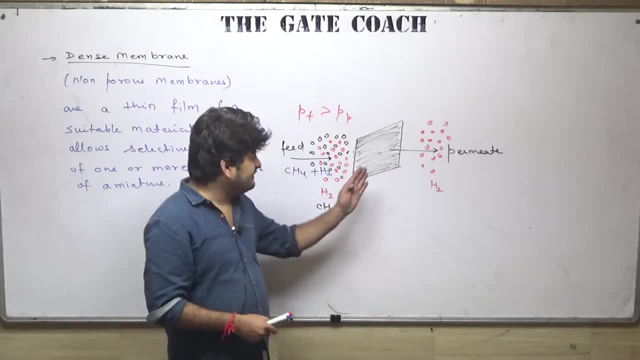 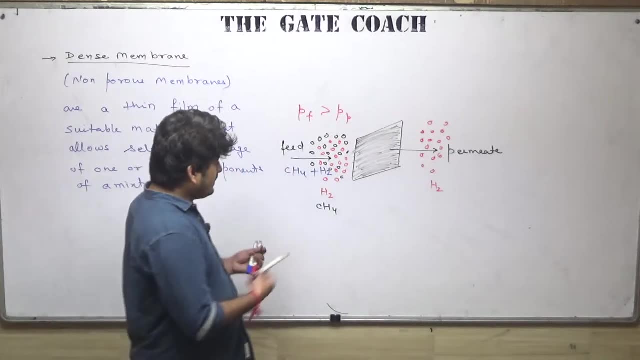 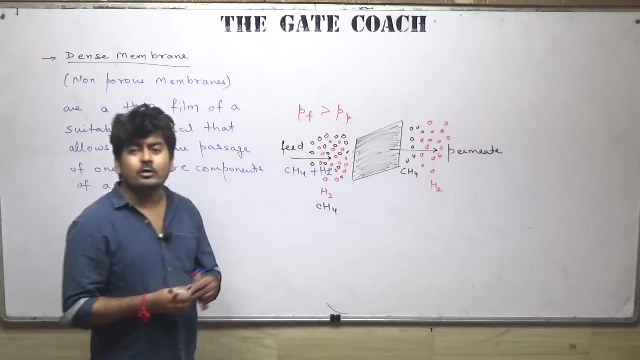 membrane. they are diffusing inside the membrane and leaving the membrane on the opposing surface, on the permeate side, like this. okay, and obviously hundred percent separation is not possible. so some of them methane molecules may also come along with this, hydrogen atoms, hydrogen molecules. so that's how this dense membrane will be disengaged. then the nextング Partners of Mup: когда 있습니다 Igncam keeper談. Ad complement Gram. 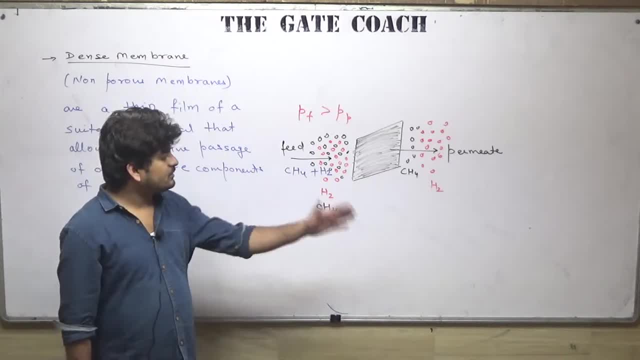 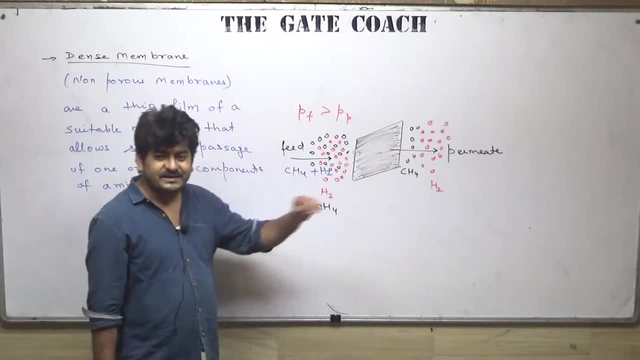 These hydrogen molecules are separated, so some of the methane molecules may also ilcome along with this. hydrogen atoms, hydrogen molecules- so that That's how this dense membrane works- Means whatever mixture you have, You pass it through this membrane. Passed through dense membrane, So the selective component in it. 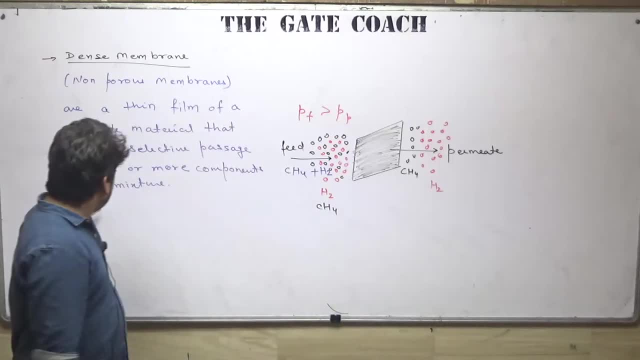 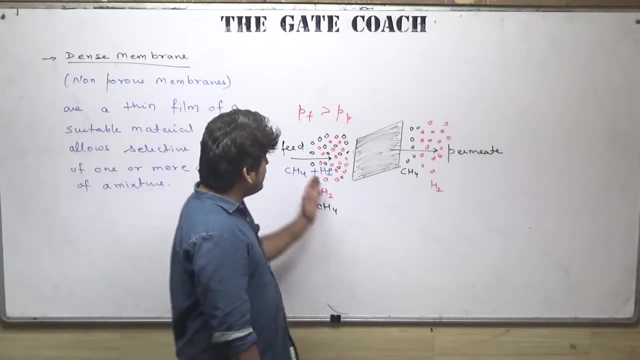 Which we have to separate, For which we have to Keep your selective passage, Which you want to select. You want to separate So that molecule on the surface of this membrane, Which is on the feed side, On that side surface, For example, this is the membrane Molecule on this side. 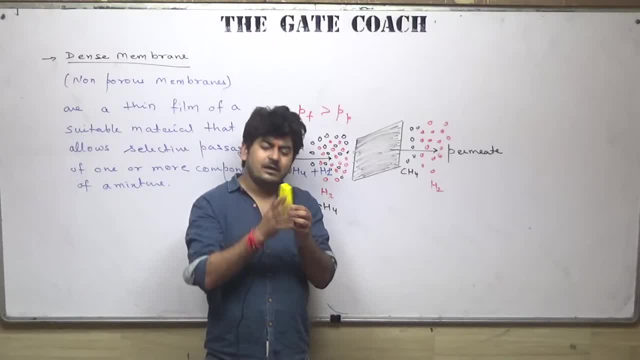 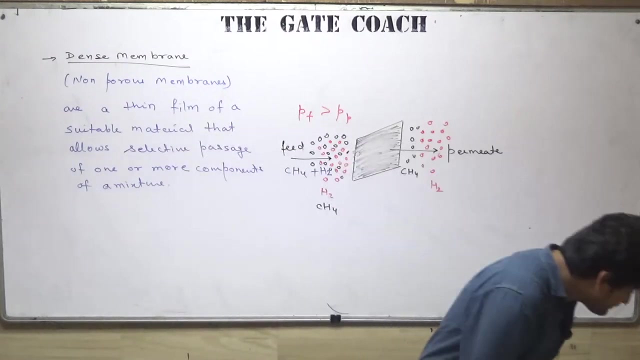 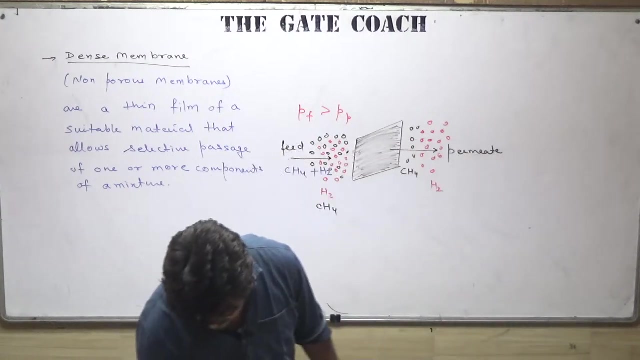 Will be absorbed, dissolved, Diffused And, on the other side, It will leave this membrane. That's how the dense membrane works. Okay, So this is something about the dense membrane Which you should know. Any example of dense membrane: Yes, Dense membranes are used, Actually, in the reverse osmosis processes. 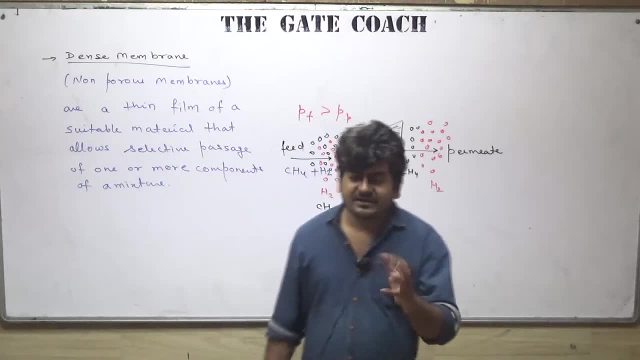 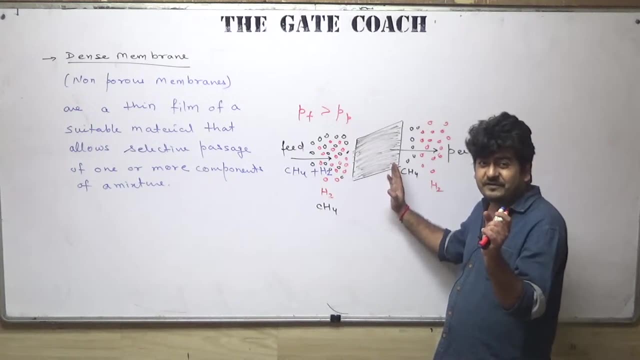 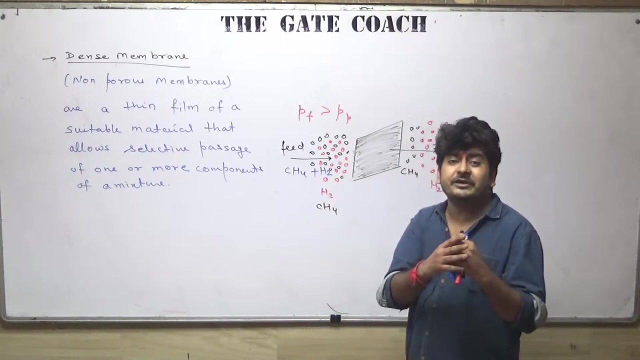 In those operations, Like you can understand What is happening: Molecule is getting dissolved, Diffusing through the thick solid surface And then leaving. So what kind of molecules Can diffuse Across the solid Through the solids? Mostly the gaseous molecules can do that. Okay, so For the gas separation operations. 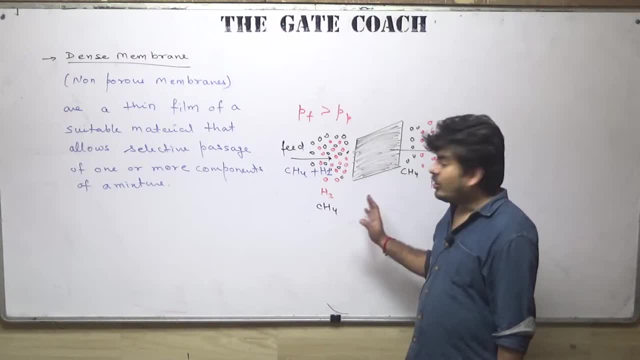 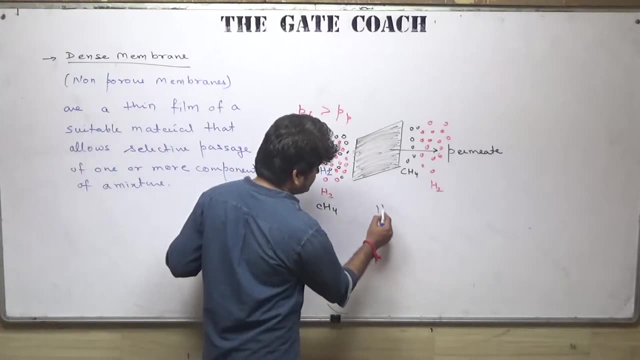 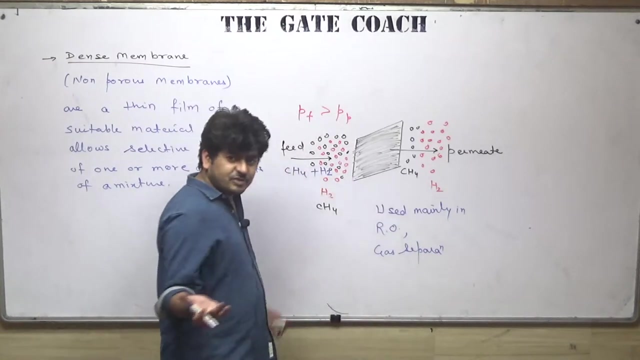 For the reverse osmosis operations Or otherwise The pervaporation operations Which we have discussed. Okay, let me write this. It is used mainly In Reverse osmosis, Gas separation operations, Where you want to separate Any gas from the mixture. Okay, just like gas absorption In gas absorption. 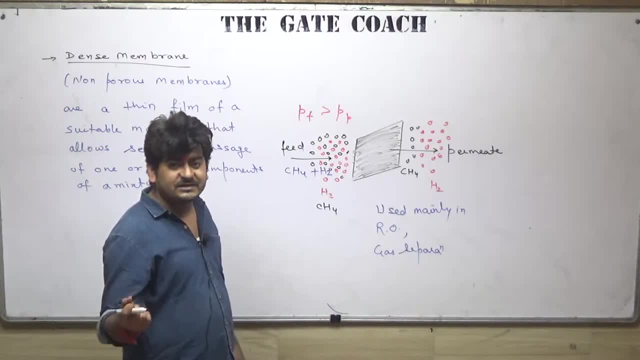 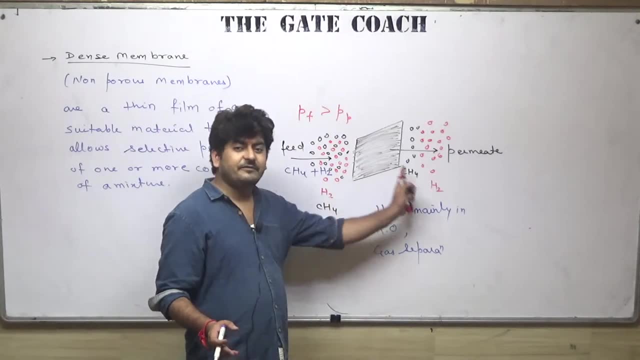 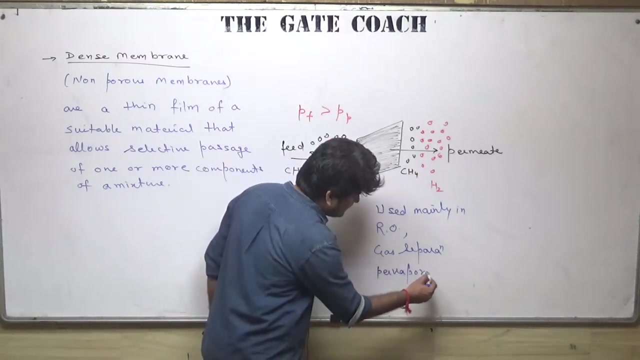 We use a liquid solvent To separate the solute. But here we don't Use that solvent. The solute will be dissolved In the membrane and diffuse and leave, Or otherwise you can say The pervaporation. That is one other way. Other techniques of the membrane separation process. 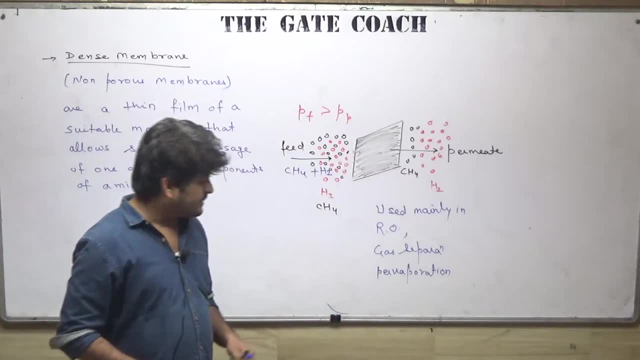 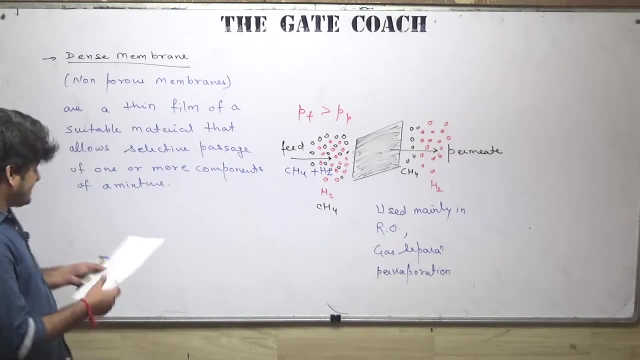 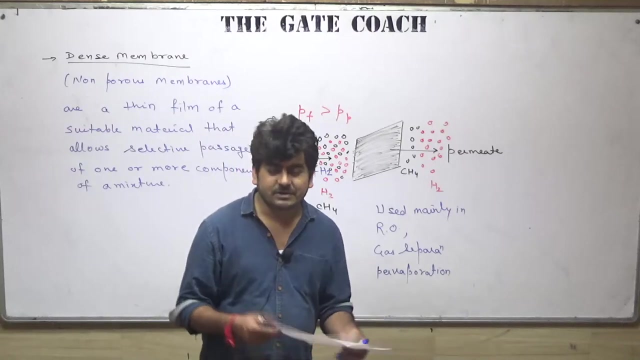 Unfortunately, we will not talk about All these pervaporation techniques, As that is not in your syllabus. Okay, so the point: If you want to write, Then you can write it, as I am using the bookish language only. Okay, that's why I am Have these notes. 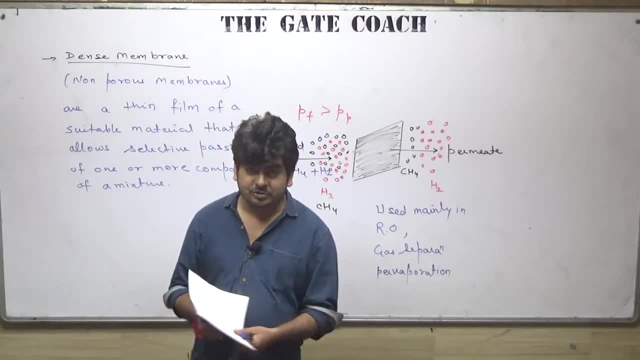 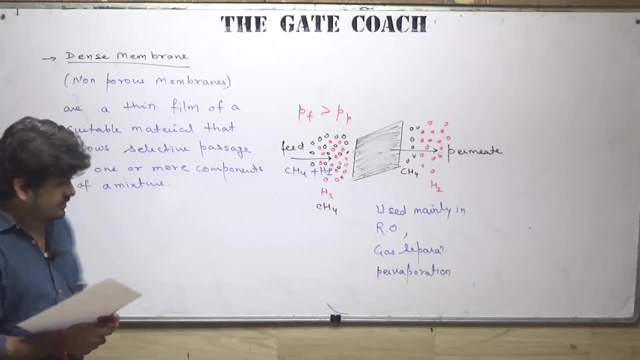 Because in GATE exam- I don't know- Maybe filling the blanks type questions may come Or multiple select questions are there. So you have to be Careful with all those things. Okay, the meaning I have I have explained to you. You can explain this dense membrane thing. 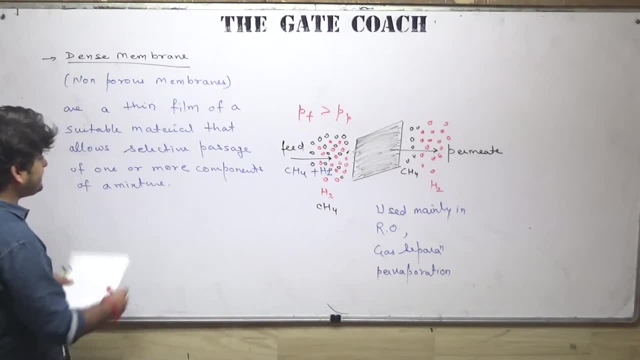 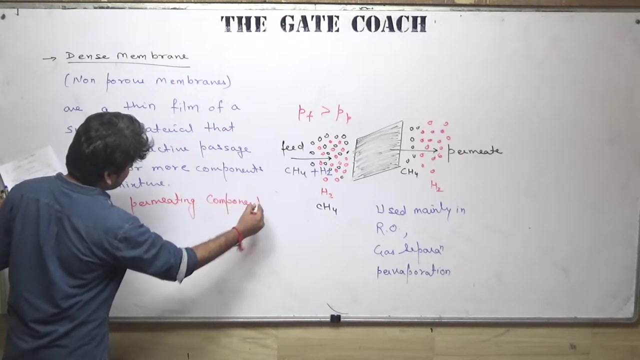 In your own words, But the bookish language. if you want to write For this entire working, Then you can write it as The permeating component. The permeating component Means the selective component Which you want to separate. Dissolves At the surface Of the membrane, Diffuses. 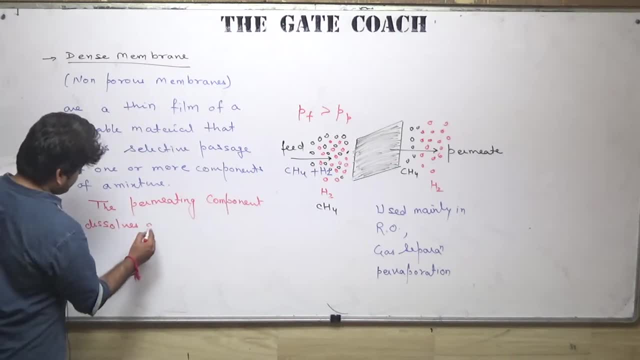 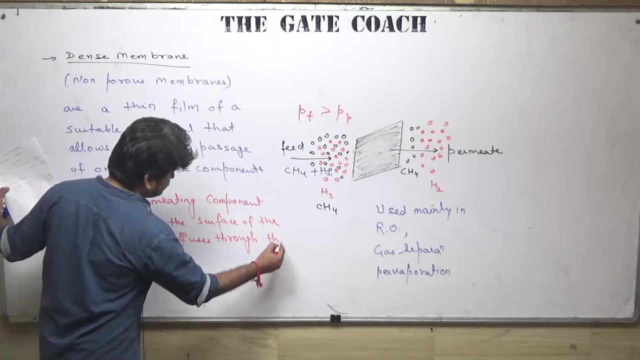 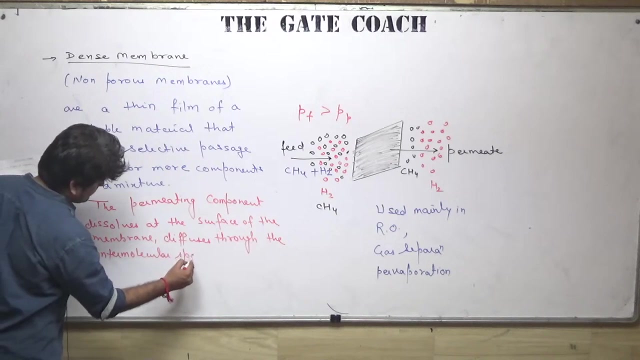 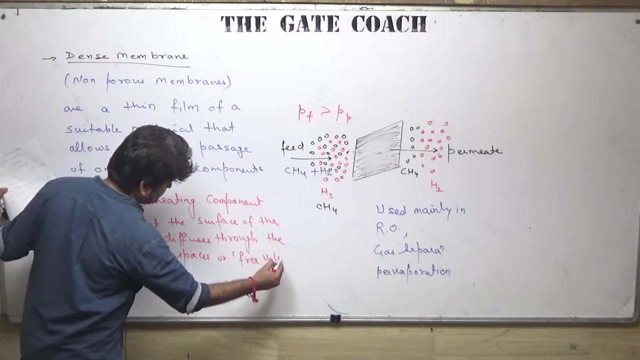 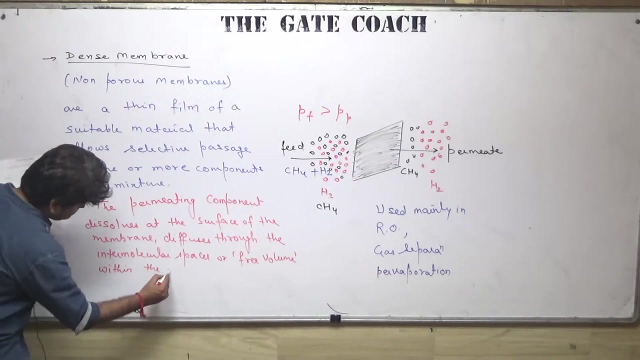 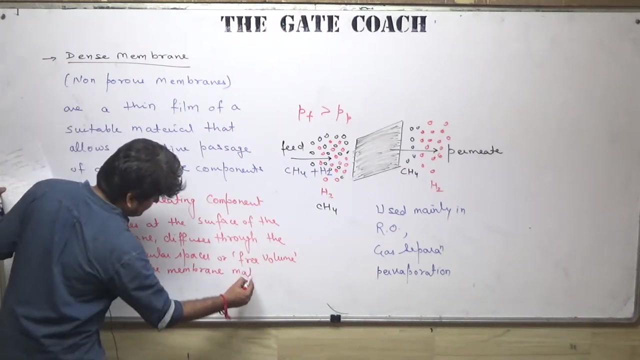 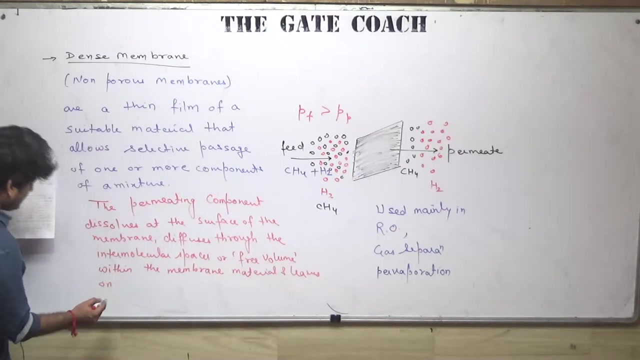 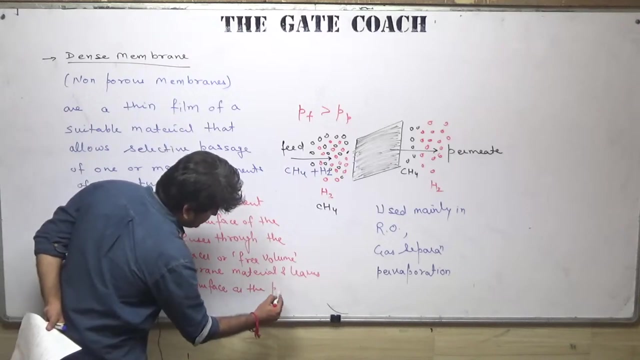 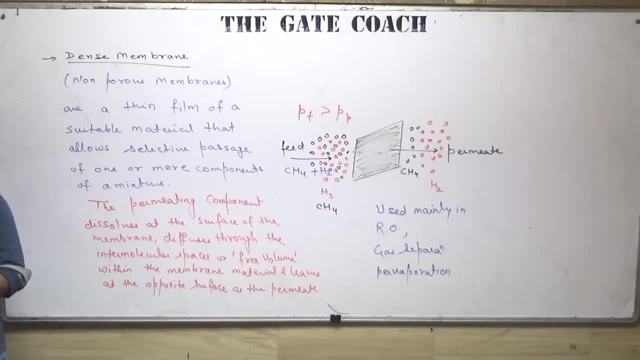 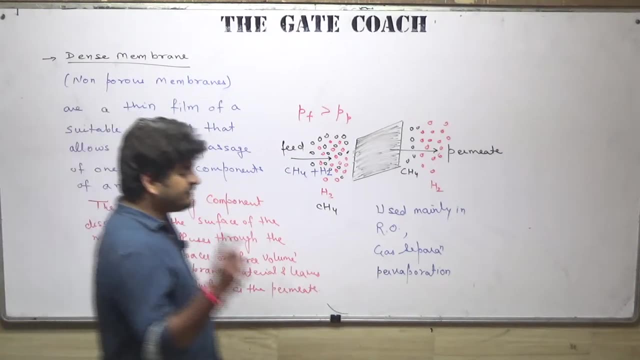 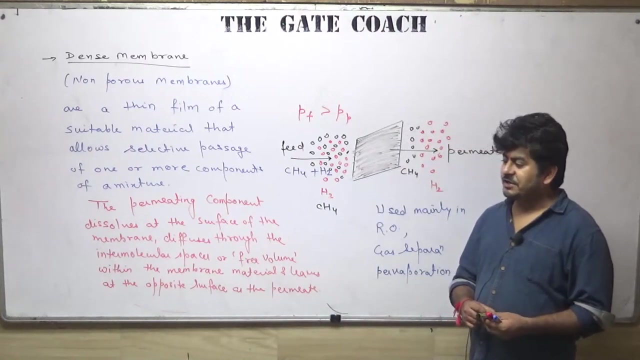 Okay, guys, so this is something about the dense membrane. There is one fun fact about the membrane separation which you should know. Okay, now I have decided that in each lecture, I will share one or two fun facts about the membrane separation- part Okay, which you should know. the key points: 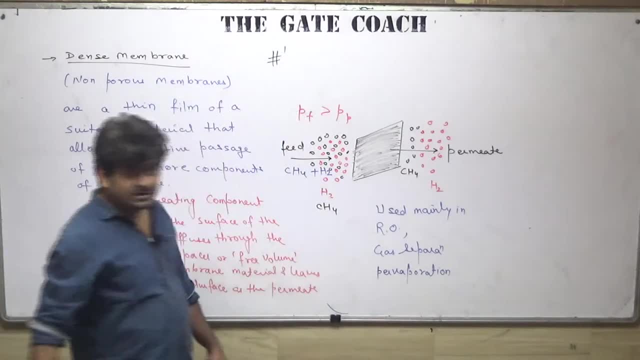 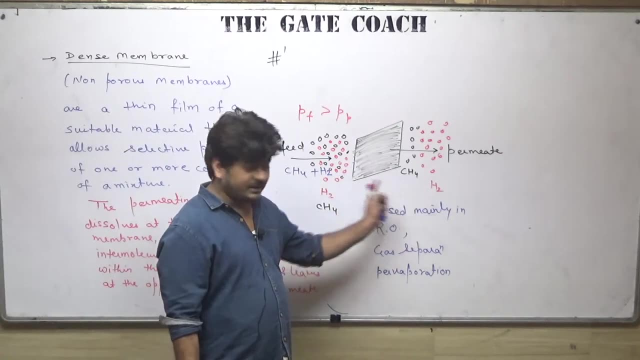 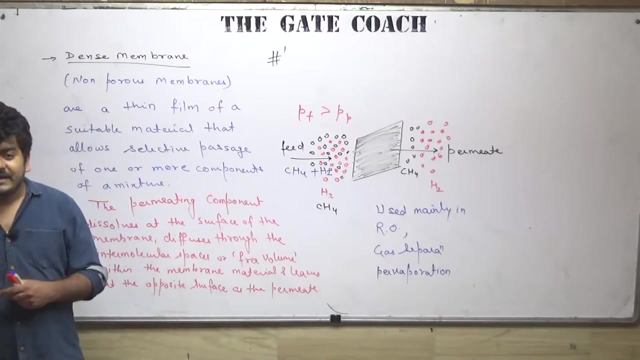 So fun fact number one about the membrane separation, That in this membrane separation molecules are moving through the membrane in the permeate phase. So transportation of the selective molecules from feed to permeate phase basically can be defined in terms of flux. Okay, what is that flux? 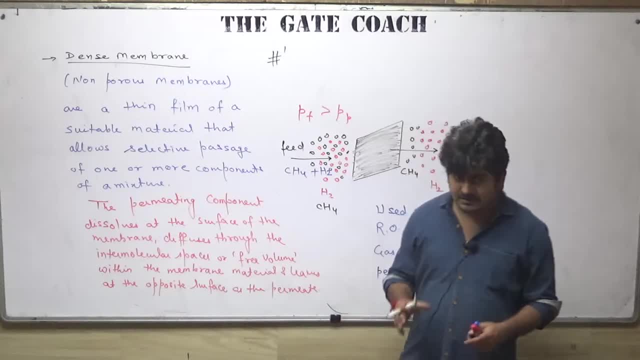 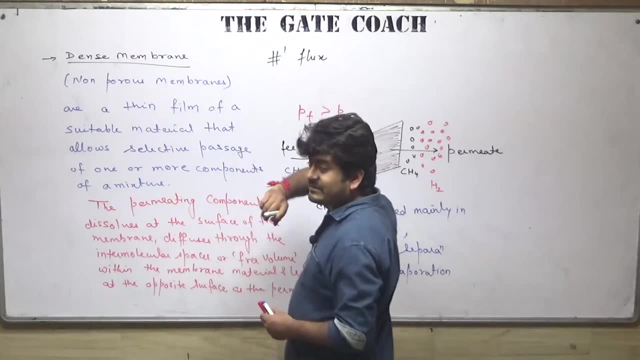 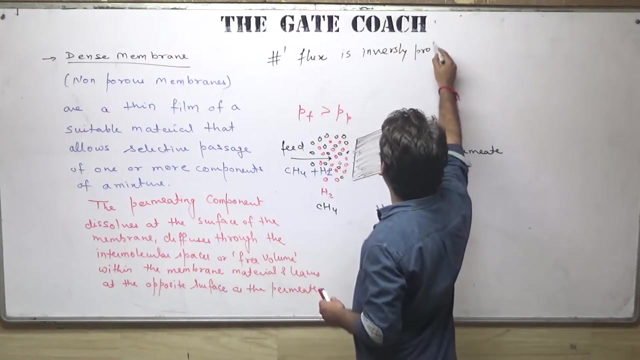 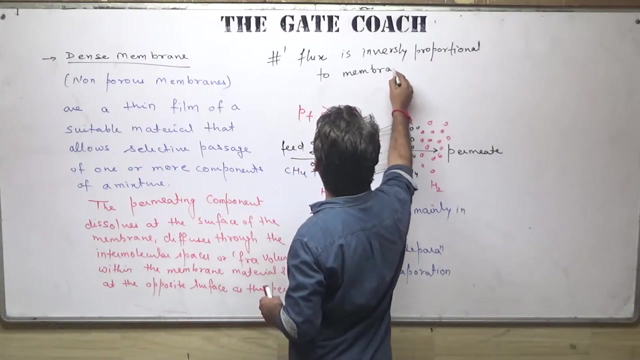 How can we define that flux? That we will discuss in other lectures, Okay, or maybe in this lecture if we get the time. But you can note the fun fact that flux is inversely divided, Inversely proportional to the membrane thickness. 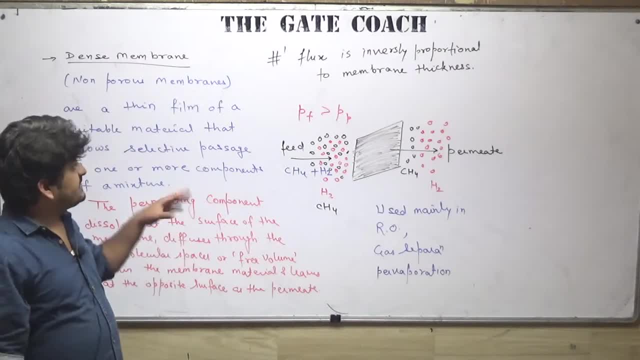 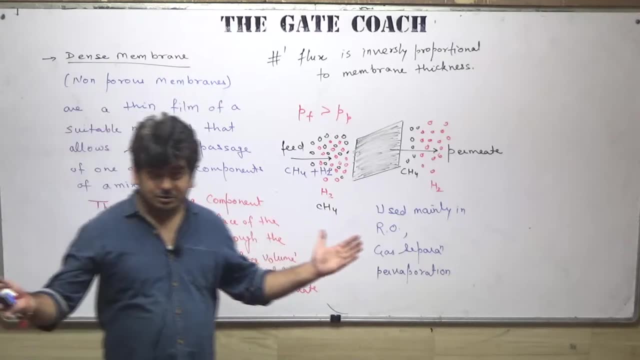 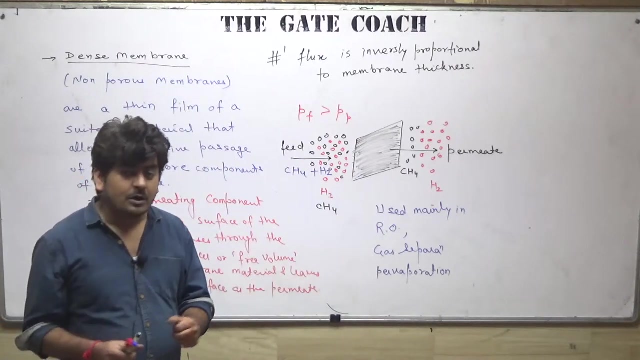 The flux of the permeate molecules is inversely proportional to the membrane thickness. Okay, so you can understand if membrane thickness is large. If membrane is very thick, Okay, its thickness is large. Then the flux will be low, So only small molecules will pass. 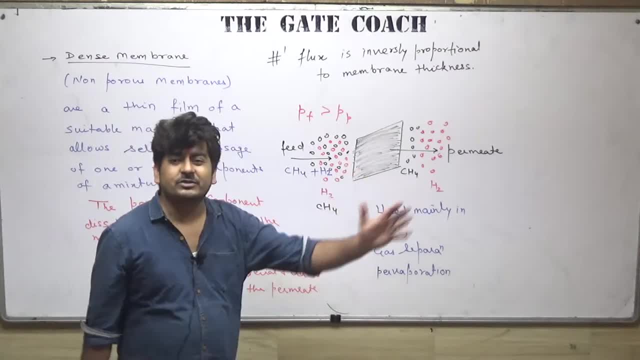 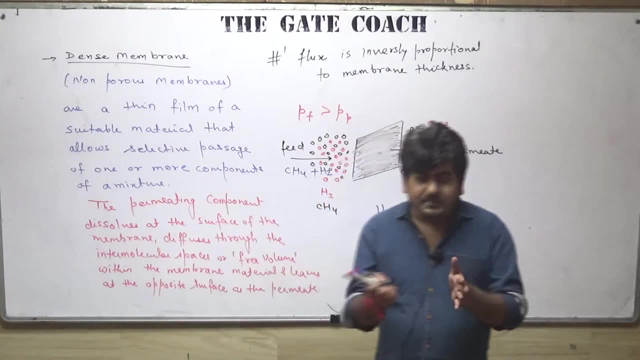 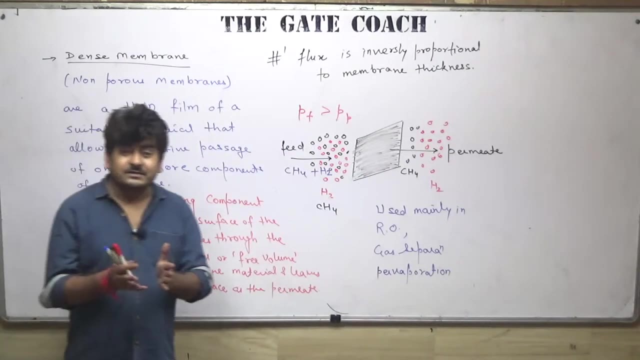 Small amount of molecules will be able to pass through the membrane. That's why in industries, in the commercial operations, we try to keep the membrane thickness as thin as possible. Okay, if the membrane is thin. Thin, Okay, means very slim, Very small thickness is there. 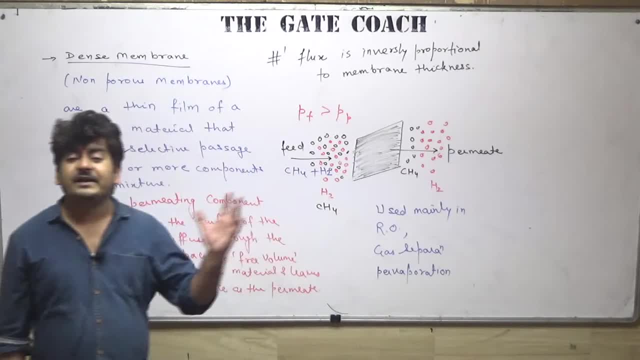 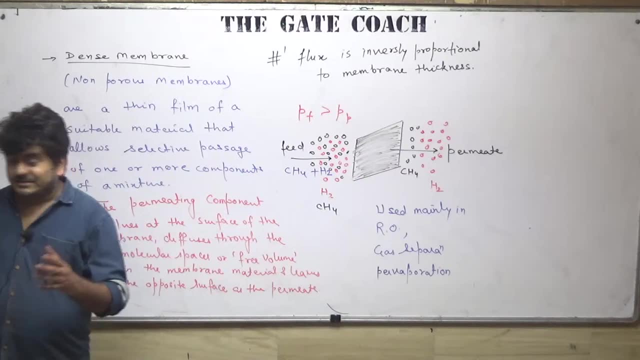 Then obviously the flux will be large And the high amount of molecules, large amount of permeate molecules, will pass through it. Okay, guys. so that's why we try to keep the thin materials, Thin membranes, Okay. next is the symmetric membrane. 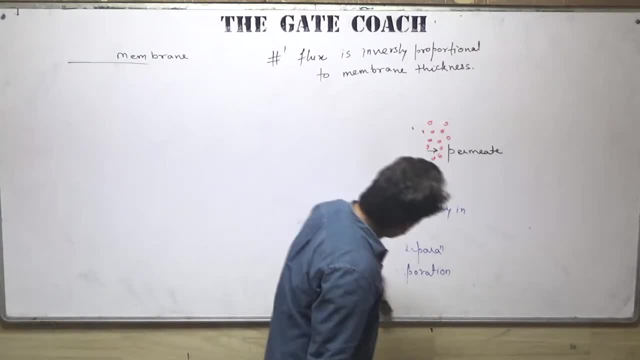 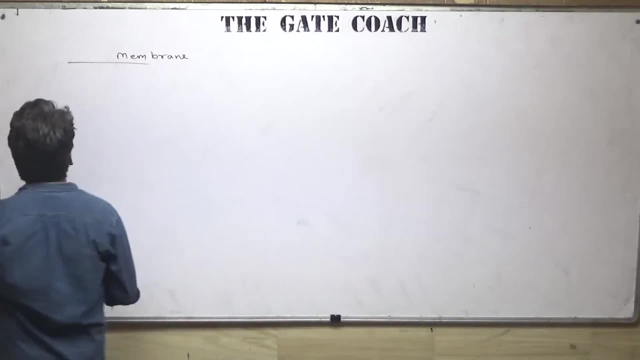 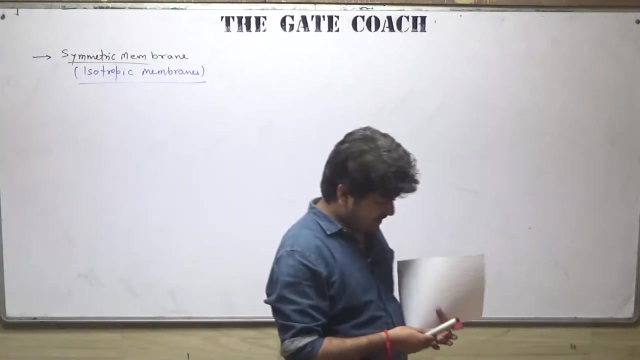 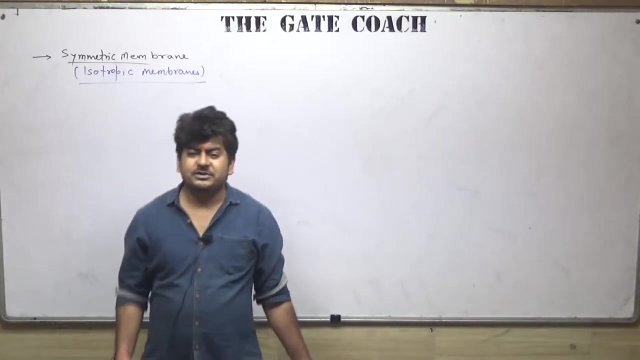 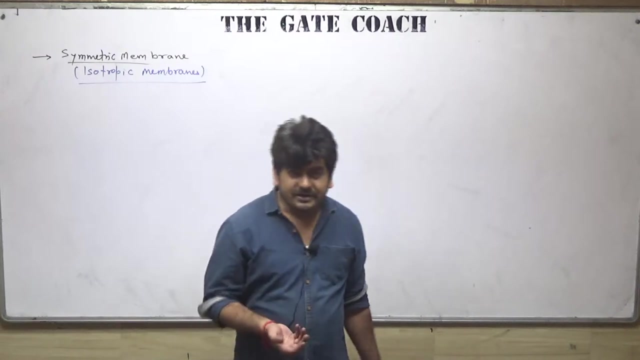 Symmetric membranes, Also known as isotropic membranes. Okay, I hope all of you understand the method we use. discuss in mechanical operation The solid-liquid separation part In mechanical operation we use to separate undissolved solid particles present in any liquid mixture. 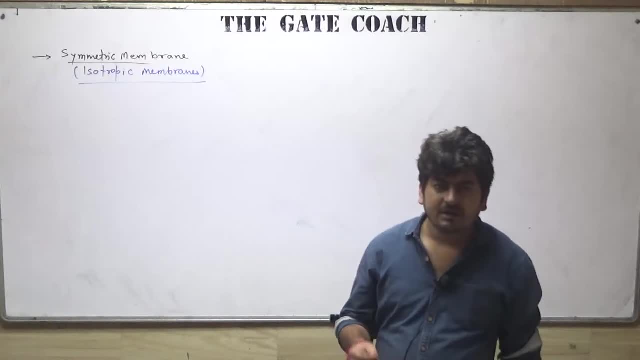 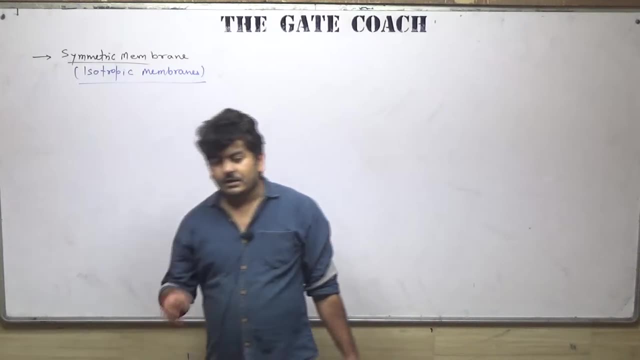 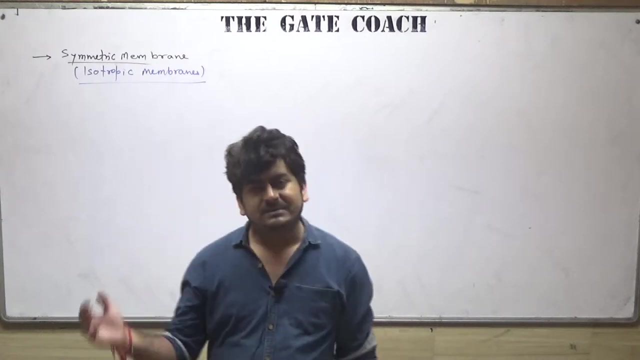 For example sand and water. Okay, Sand particles are undissolved, So that is a suspended suspension or the suspended mixture. Okay, So in those kind of mixtures we use mainly two techniques: Filtration and sedimentation. Sedimentation is used for the coarse, fine size particles. 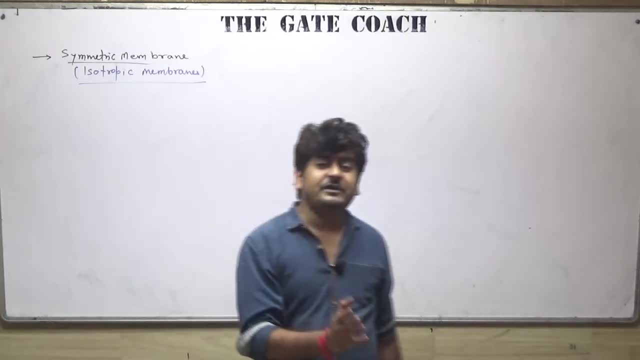 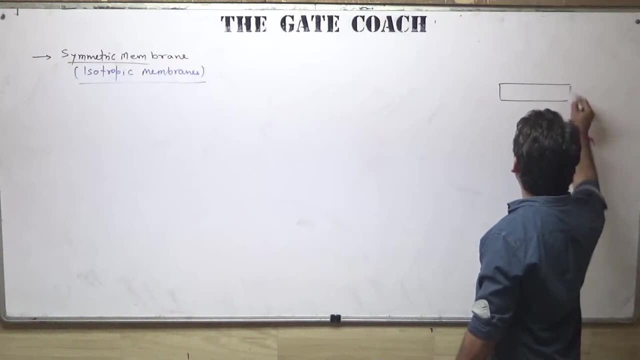 So separation of fine size particles, that is a different story, And filtration is used for the separation of coarse size particles. So what happened in the filtration? This is some filter medium, The porous medium also known as septum. We supply the solid-liquid mixture from the one side. 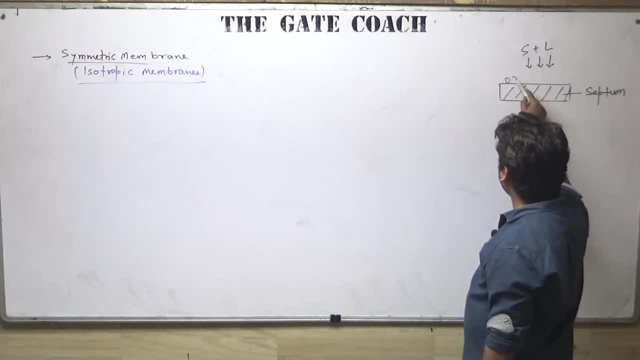 The size of the solid particles is greater than the pore size of the septum, So they will get retained. And liquid molecules have size smaller than the pores, So they will pass through this, Okay, as the filtrate. So this is conventional. 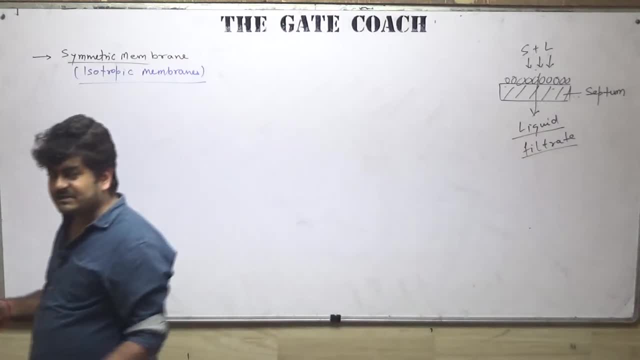 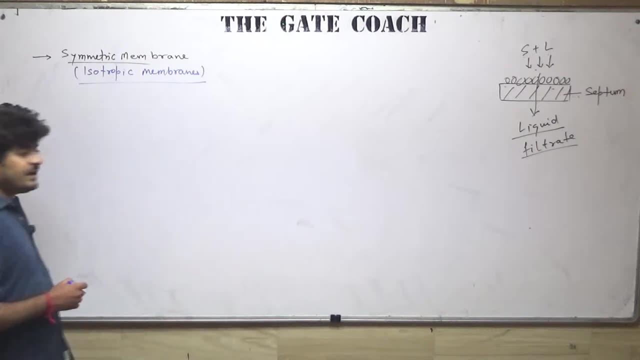 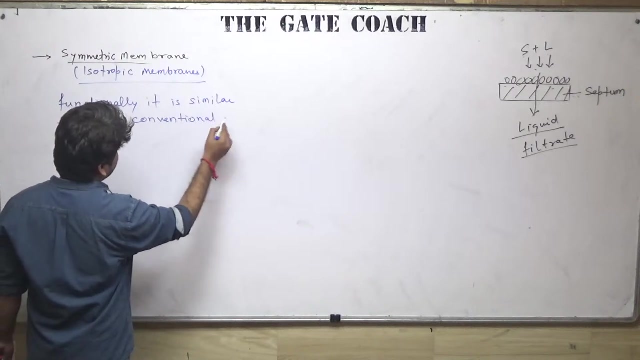 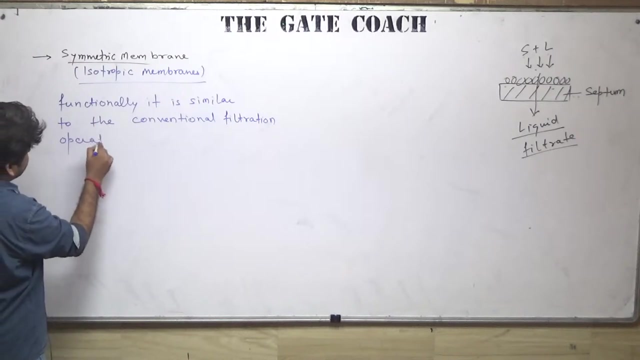 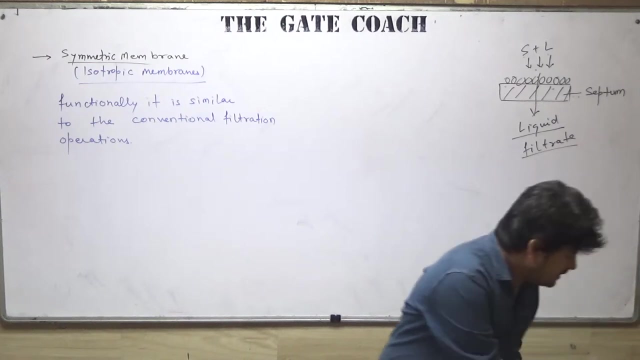 Conventional separation method which we use for the separation of undissolved solid particles from the liquid mixture. Okay, So if I talk about the symmetric membrane, So functionally It is similar to The conventional filters. We filter the leaves and素 Seb. 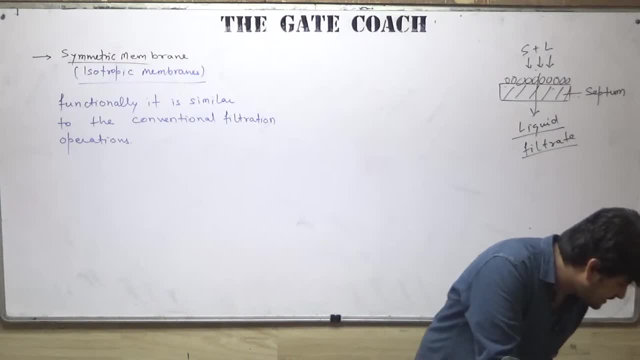 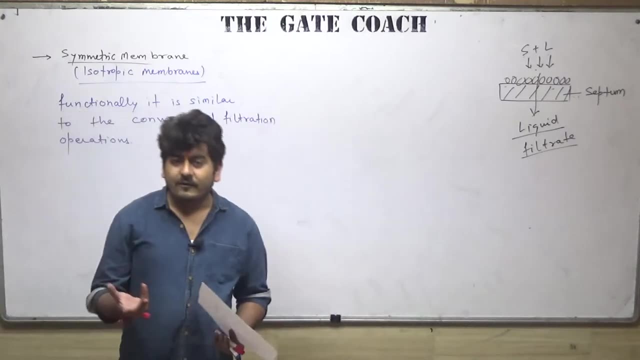 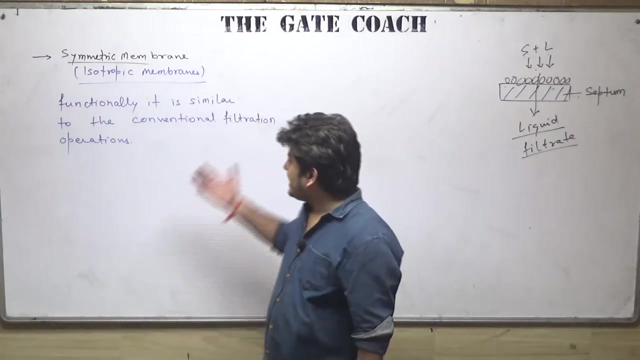 These filters are used for filtering undissolved solid particles. Sir, here resistance will continuously increase across the membrane or remains constant. See, here it's obvious that, as membrane is what Membrane is, just kind of a barrier, okay, which we are using to separate some components from the existing mixture, from the feed. 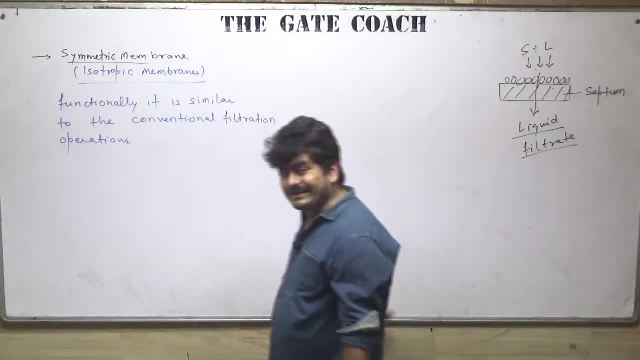 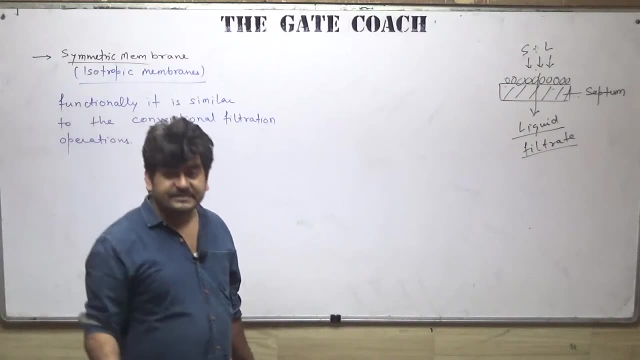 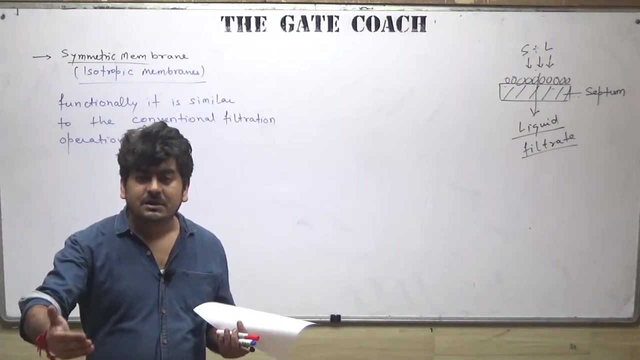 Okay, it is a barrier. So if you increase the thickness of this barrier means the membrane thickness. if you increase, so obviously the resistance will increase. okay, As you can understand, if the thickness is large, then molecules, the molecules which are passing through this membrane, 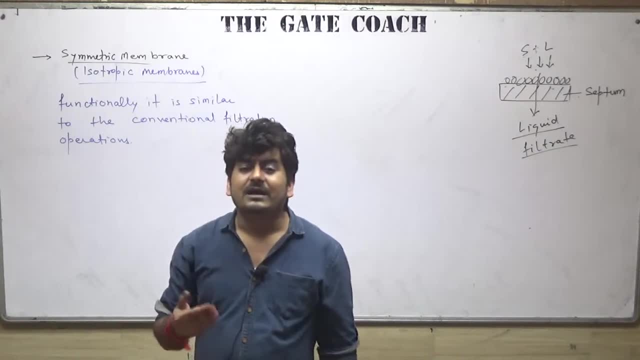 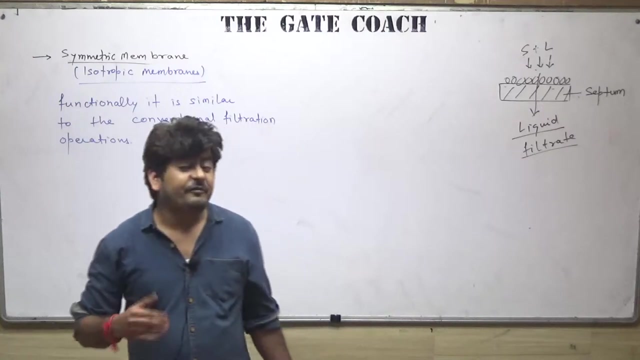 they have to consume a larger amount of energy And as their energy consumption increases, so you can understand that resistance increases. For example, if you have to run for 100 meters, you can run as fast as you possible, but if you have to run for 20 kilometer, 10 kilometer, 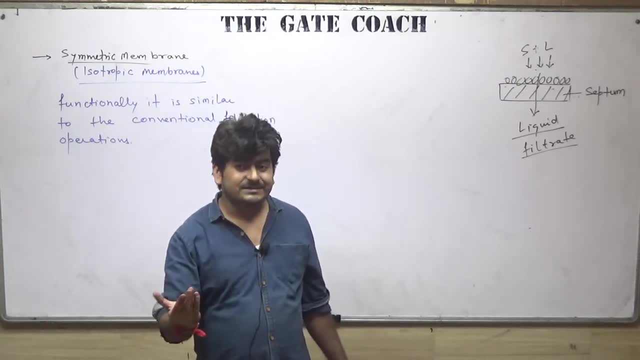 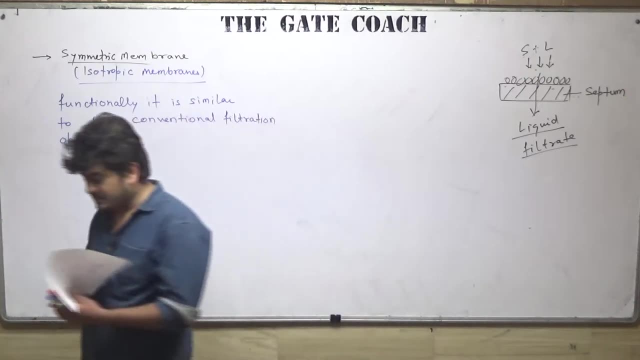 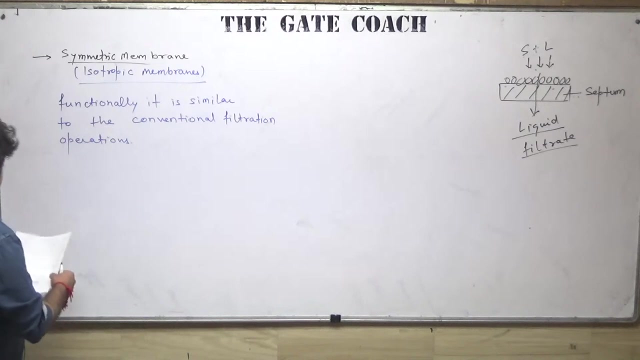 then obviously the resistance- energy consumption- will increase. the resistance is high because you have to travel a larger distance, so that's a thing okay in a every situation. So let's talk about the symmetric membrane. so write down, guys. 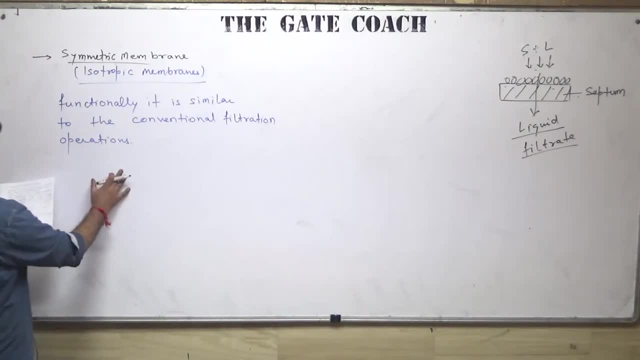 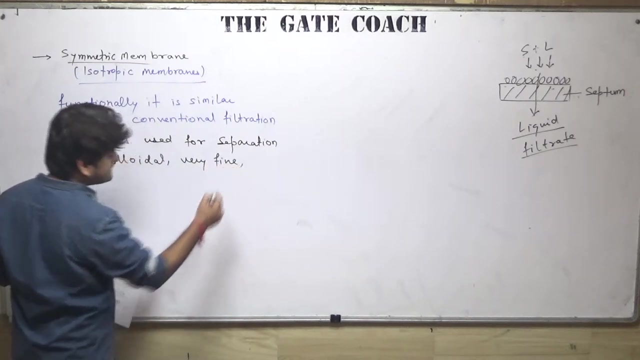 Here, Here, Here, Here, If I want to write about the symmetric membranes. So, first thing, while filtration method is used for the separation of coarse particles, these symmetric membranes are used for separation of colloidal particles, very fine sized particles. 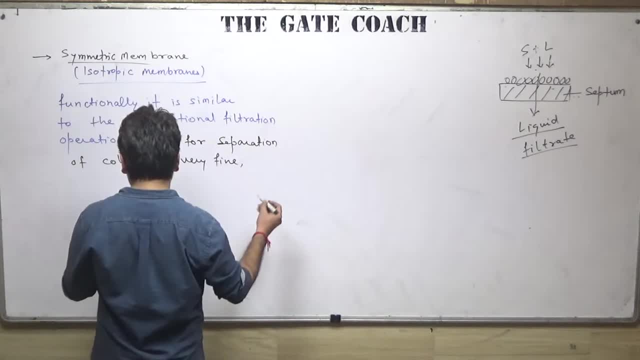 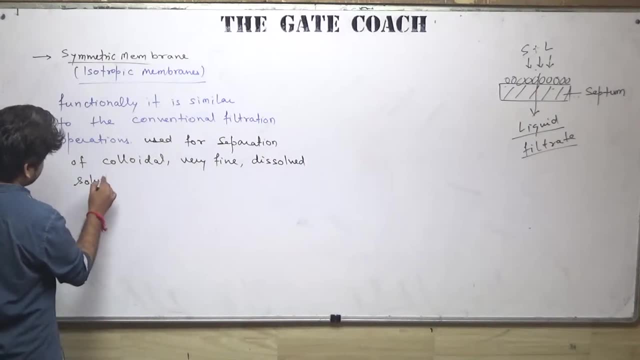 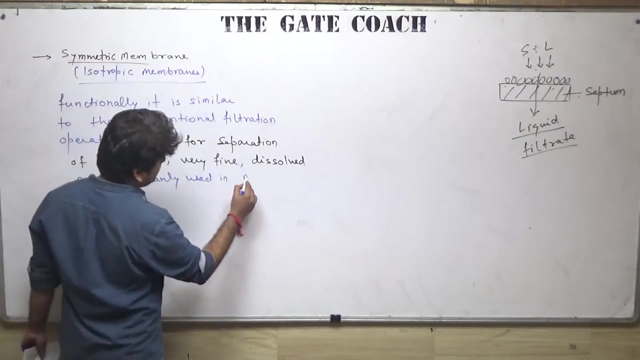 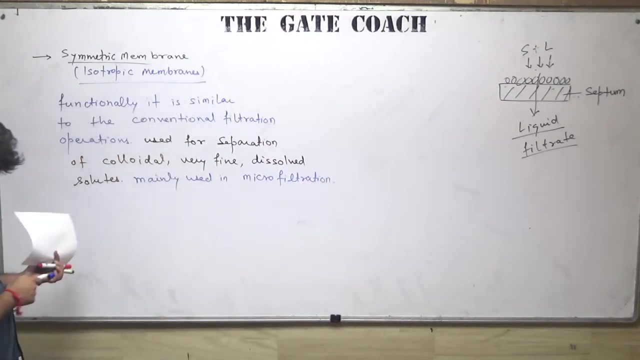 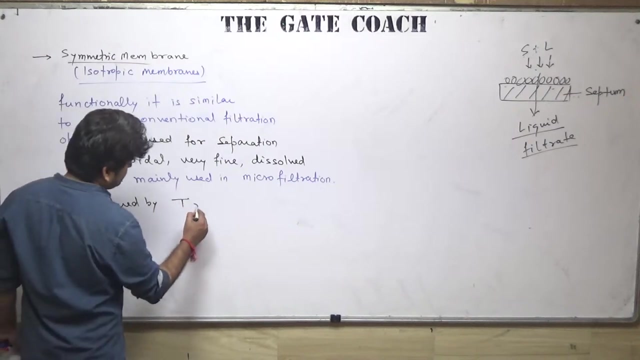 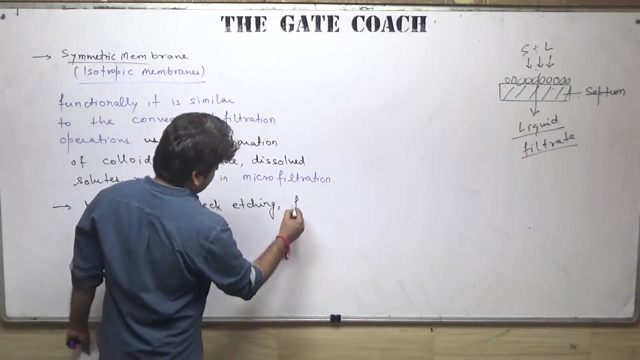 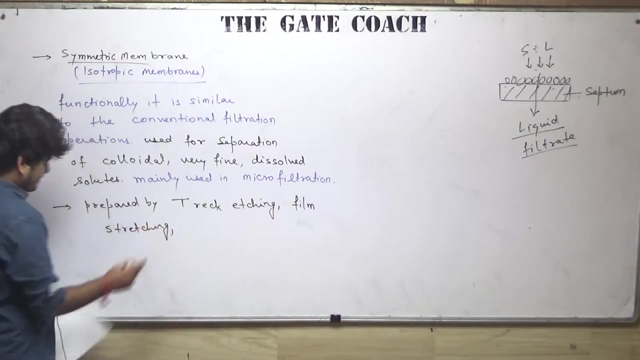 okay. Or you can say that dissolved solutes and normally used in microfiltration, Okay. and if I talk about the preparation method, how can we prepare the isotropic membranes, the symmetric membranes? so these membranes can be prepared by track etching method, film stretching method and solution precipitation techniques. 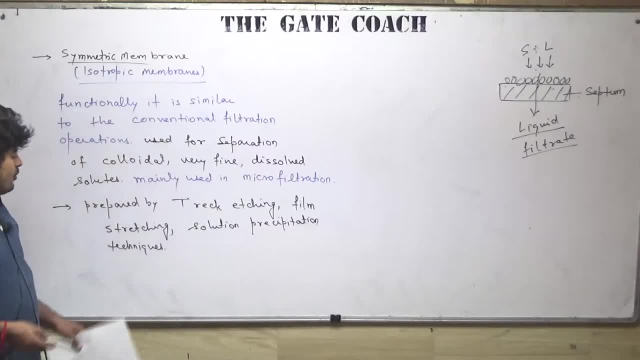 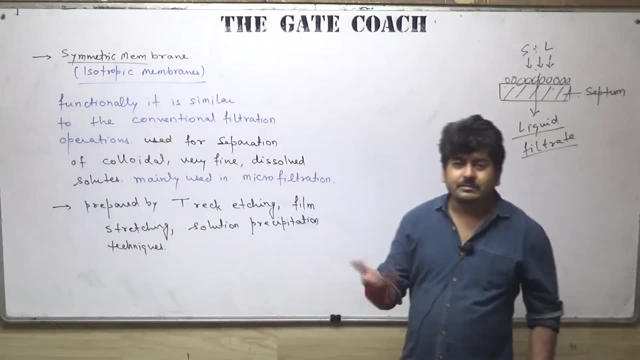 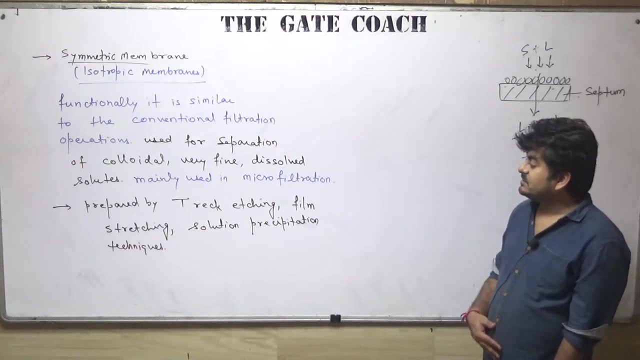 okay, what are these methods? see, I don't know we have to do discuss all these things or not, because only membrane separation is there in your syllabus, but in literature it is available. okay, so what will I do? I will share the handout of all these three methods with you. 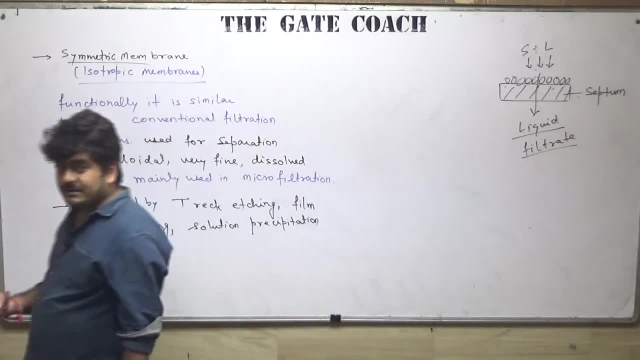 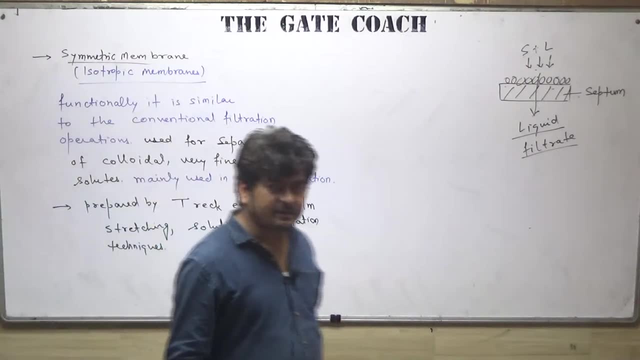 in the telegram group so you can. if you get some, if you have some extra time, then you can read about all these three methods. these are very simple methods. you can read about all these three methods and I will share the handout of all these three, and all the theory is there. that's why I am not discussing all these things. 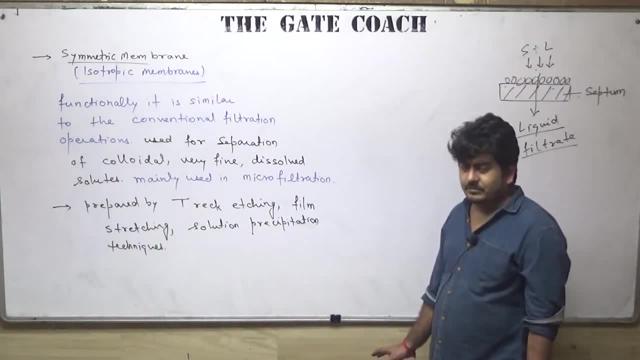 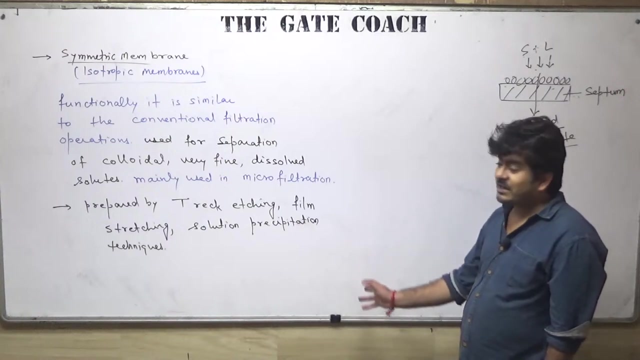 because we will discuss the only important points. I hope all of you know that membrane separation is a theoretical subject, so we cannot discuss the entire theory only. so I am just discussing the important parts so that you can revise this part in a shorter span. so if you have some extra time you can read. 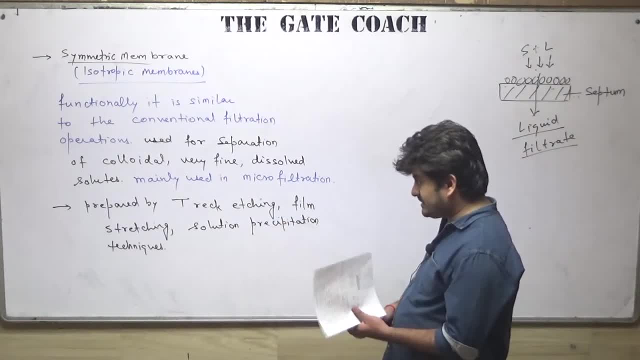 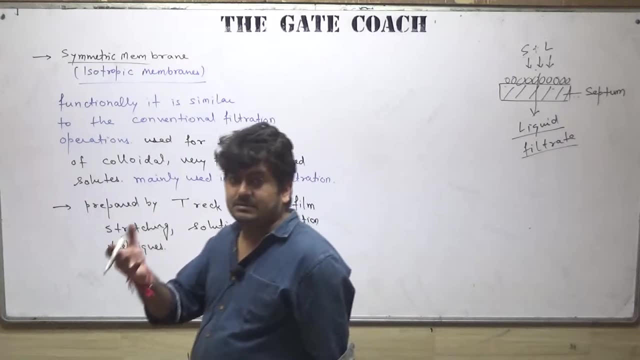 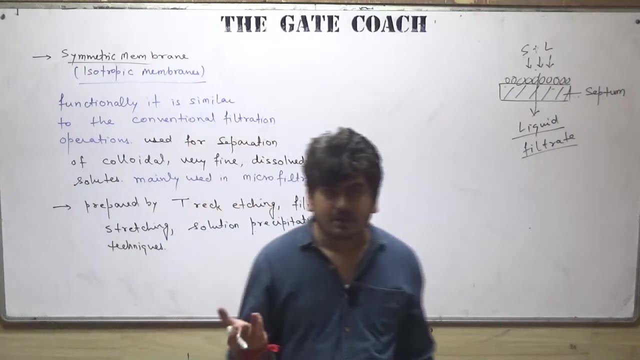 about all these three methods and if I talk about the symmetric membranes, so as the name says, symmetric means some pattern, similar pattern is there. so what is the similar pattern? what similarity can be there? where will that similarity be in the membrane? what will be there in the membrane which we can keep similar? 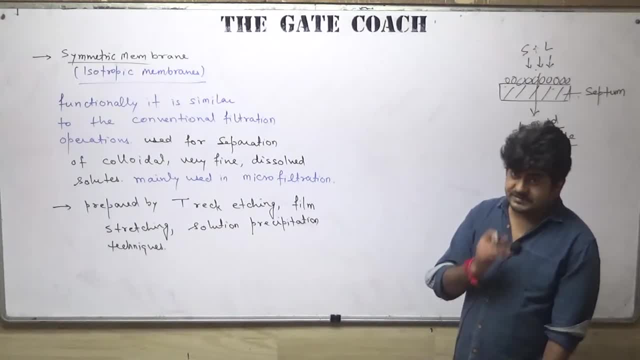 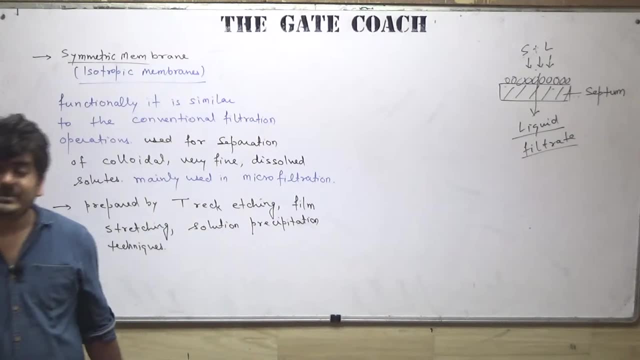 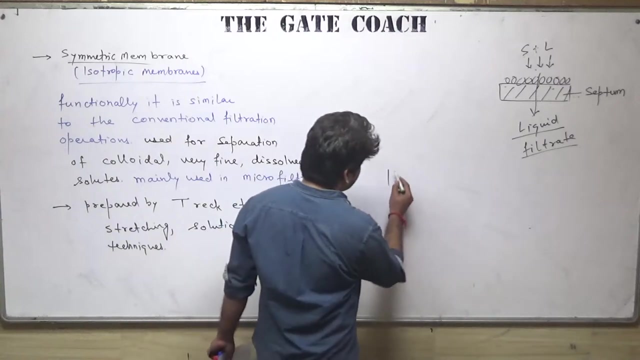 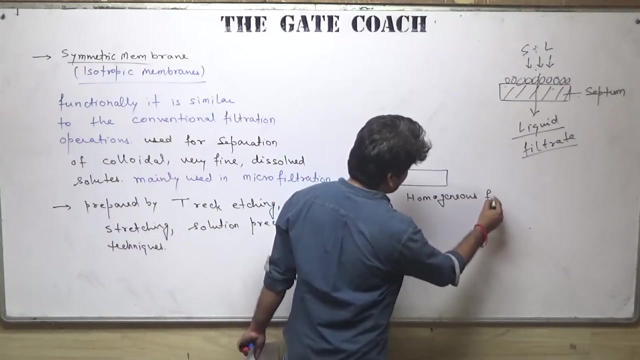 or not, so that is called pores. in any membrane there are pores which can be similar or non. similar means symmetric or asymmetric. so for the symmetric membranes, the membranes, it can be a homogenous membrane, or you can say the homogenous film means, just like a dense membrane, a thick, solid. 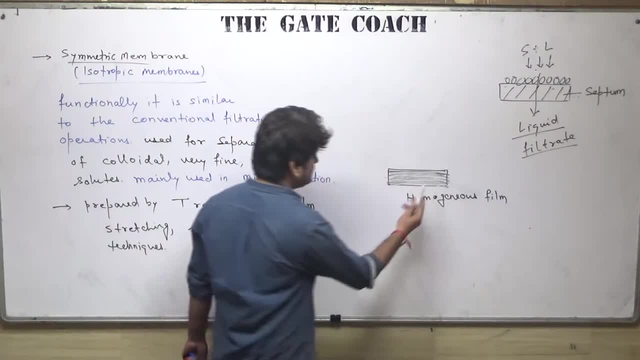 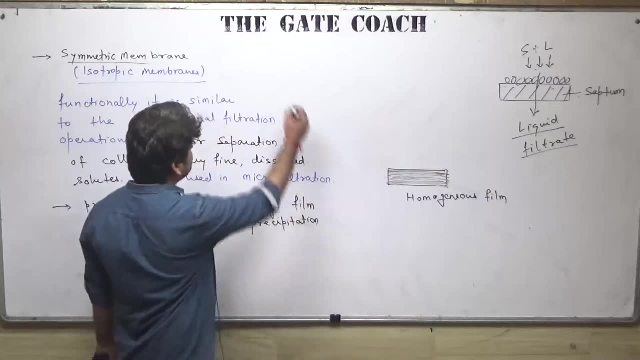 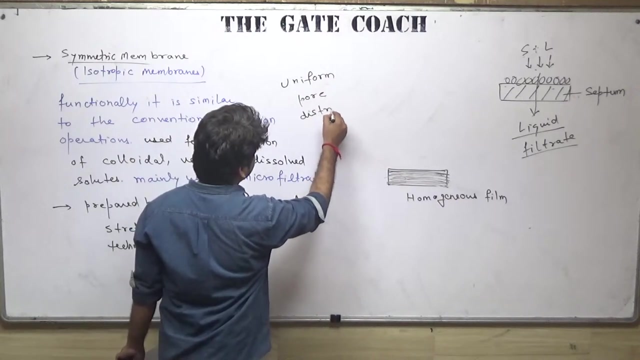 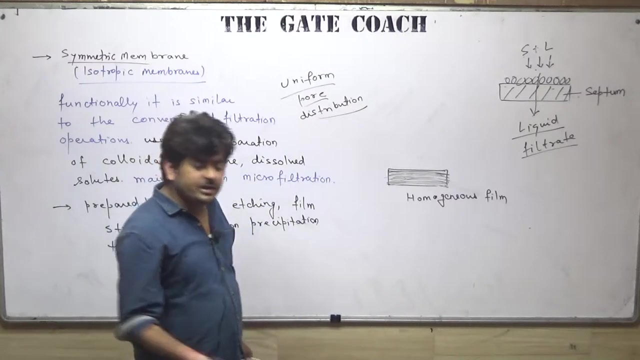 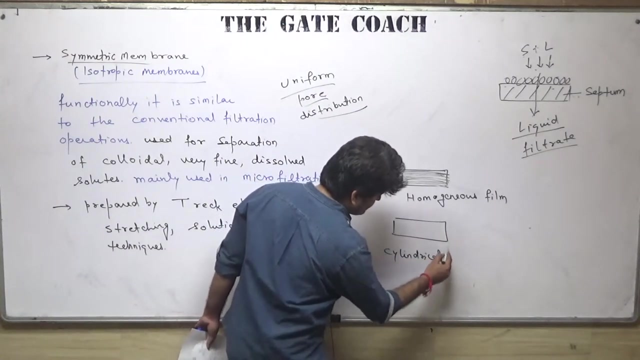 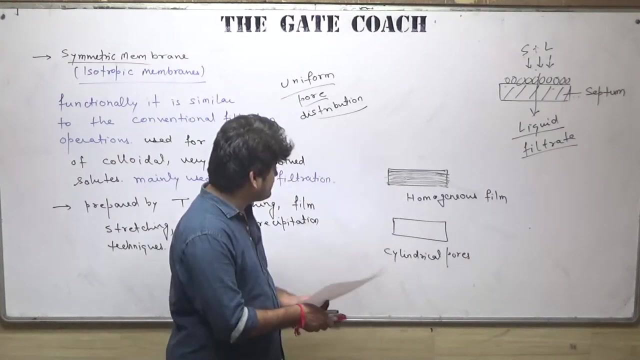 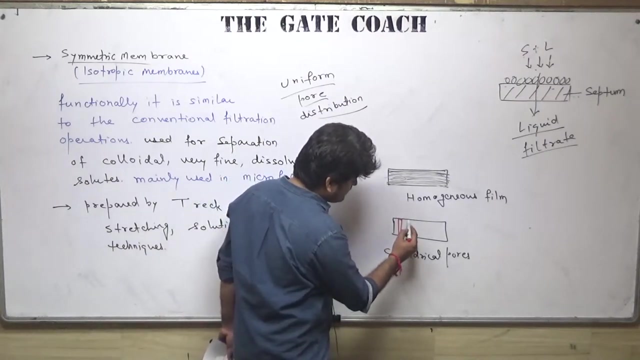 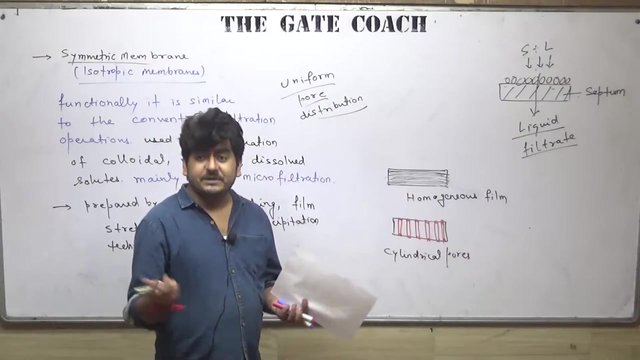 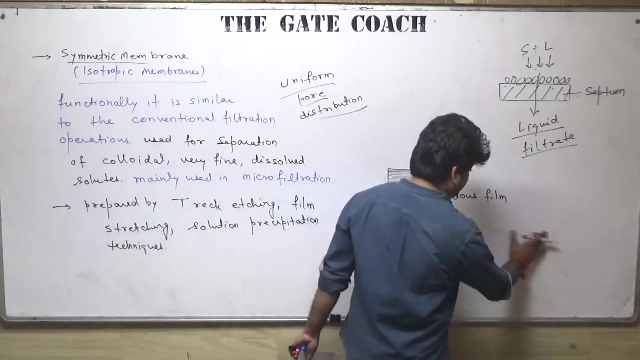 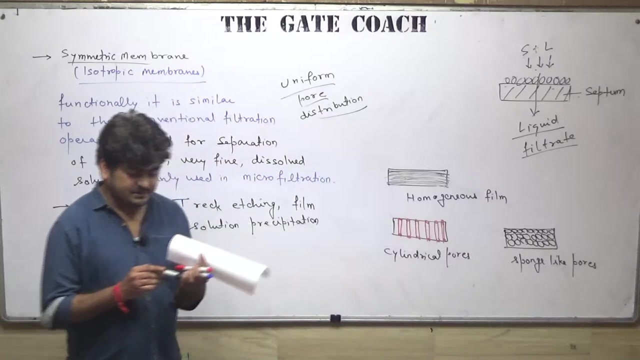 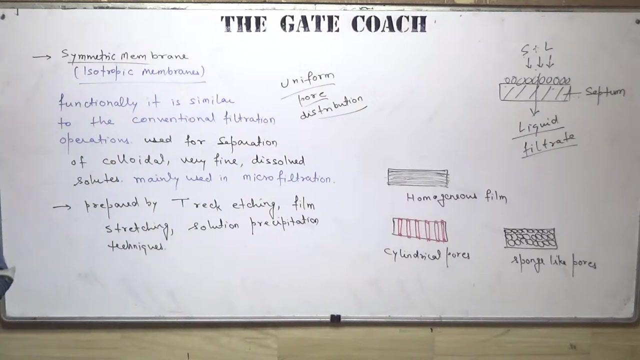 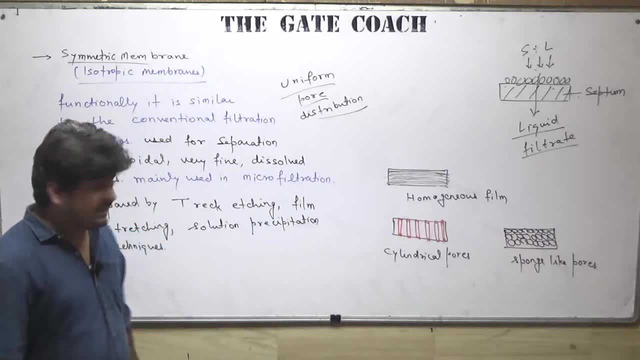 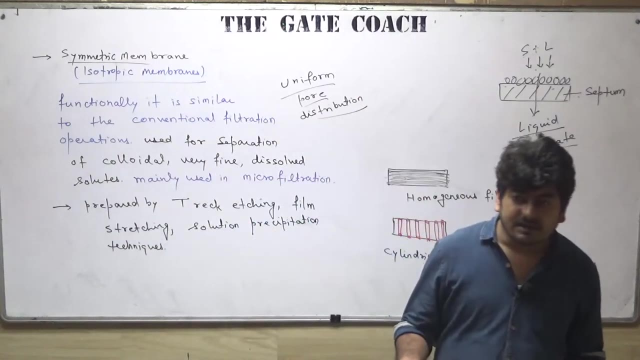 ok, ok, ok. And microfiltration we do mainly for the. as we discussed in last class as well. microfiltration we do for the separation of bacterias, yeast kind of things means the microbial entities. to separate those microbial entities from the mixture. 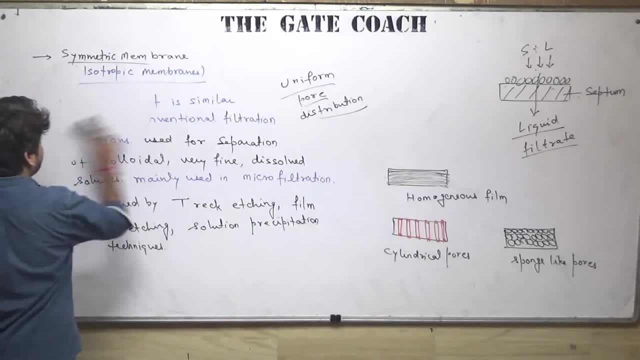 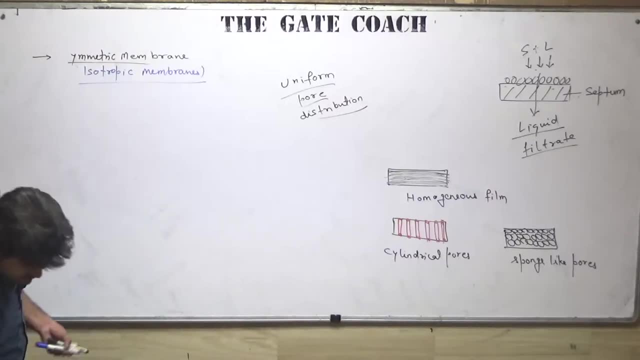 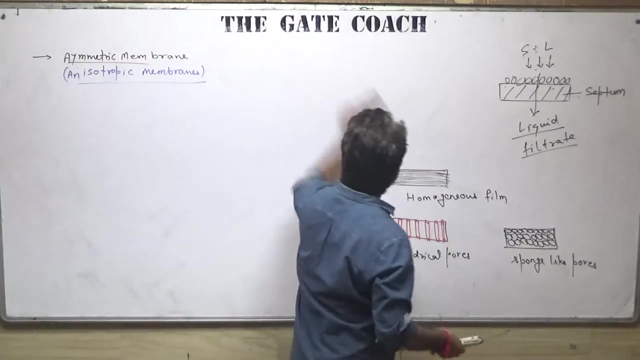 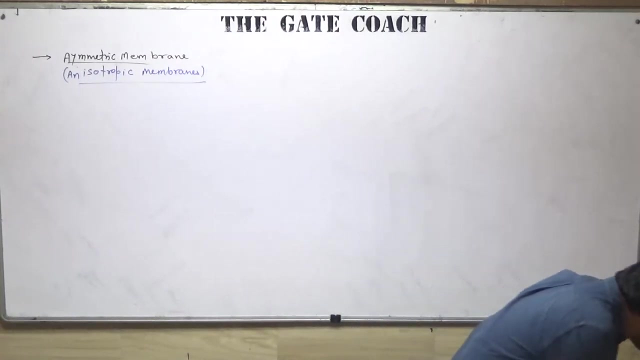 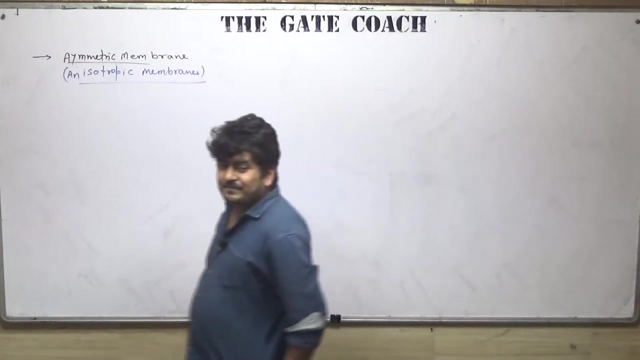 Next is guys, asymmetric membrane, Also known as anisotropic membranes. Just, we will discuss all those things. okay, What are the one thing? we have discussed about that in the last lecture? that desired attributes of any membrane. Okay, what are the attributes are required to select a membrane. 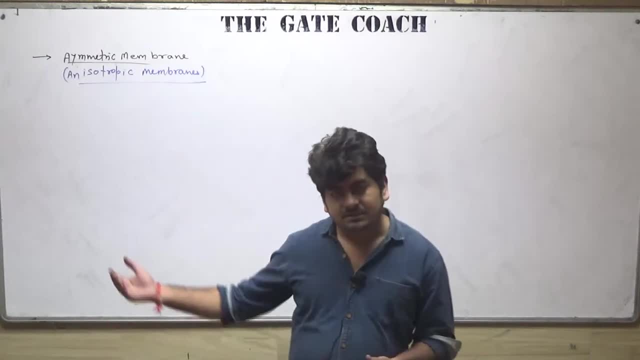 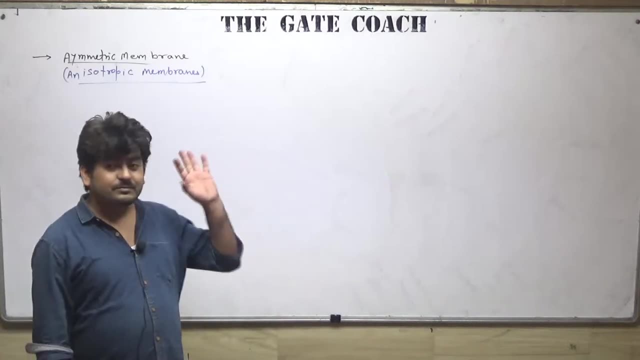 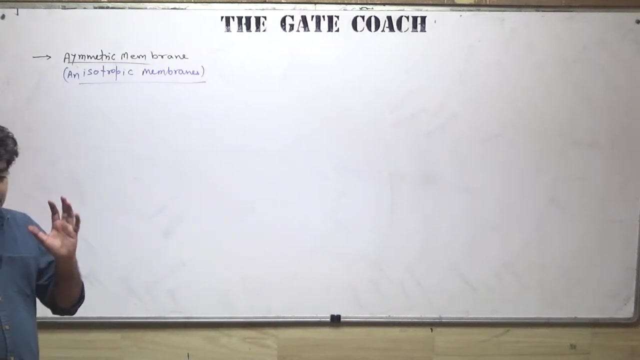 for the desired operation. Otherwise, we will discuss that in the coming part after this. membrane classification in membrane modules itself: Okay. membrane module is the biggest topic in this. membrane separation subject: Okay means we will discuss all these things, how the transportation is taking place, their methods and all. 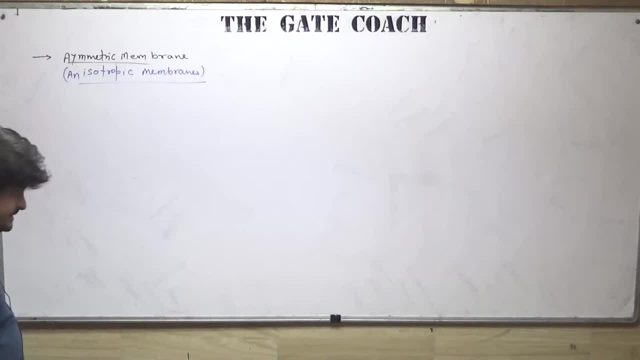 And what the characterization of membranes. Next is asymmetric membrane, Also known as anisotropic membranes. Okay, so what are the asymmetric membranes? So, guys, that is that you need to understand. okay, Asymmetric membrane has a thin film of 0.1 to 1 micrometer. That is a thin film of 0.1 to 1 micrometer. So that is a thin film of 0.1 to 1 micrometer, Also known as anisotropic membrane. So the way it is 🎵. 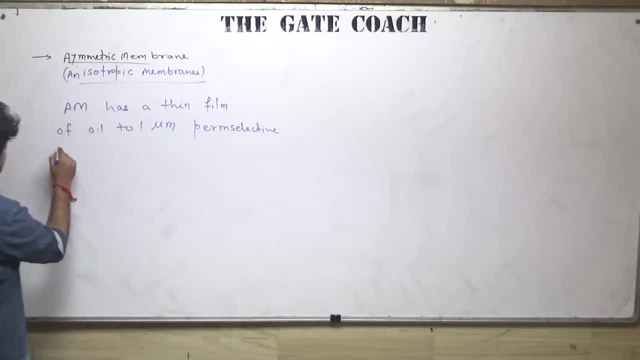 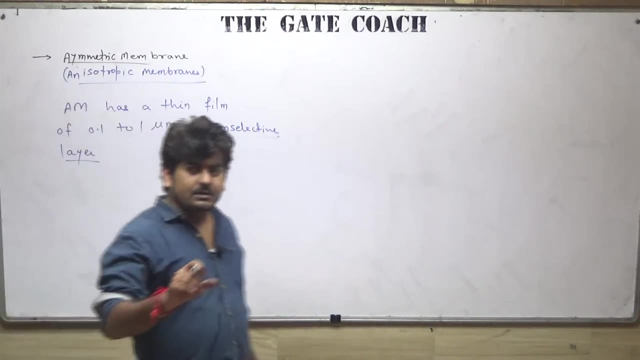 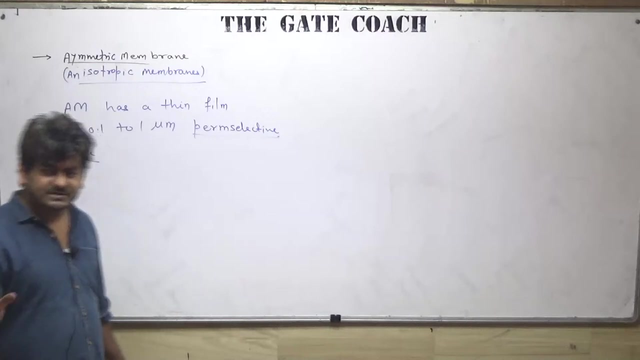 Perme selective layer. Perme selective layer. I hope you understood the meaning of Perme selective layer. Perme selective layer means the selective passage. okay, In any mixture, only the selective components will be able to pass through it. That is Perme selective. 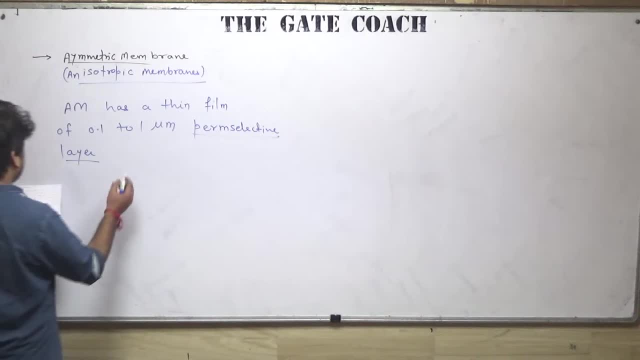 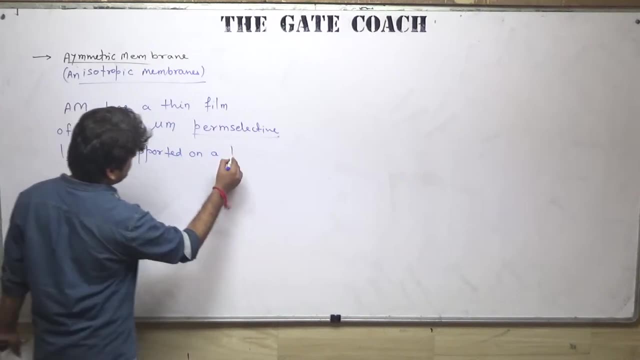 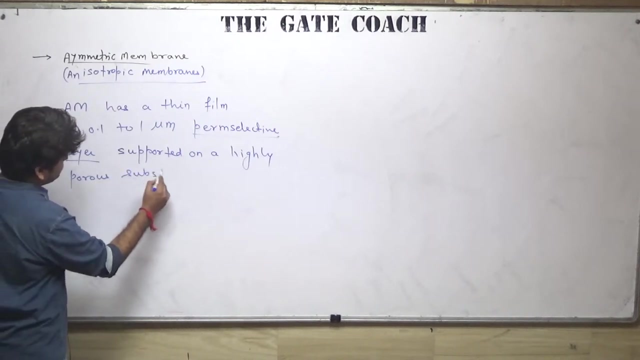 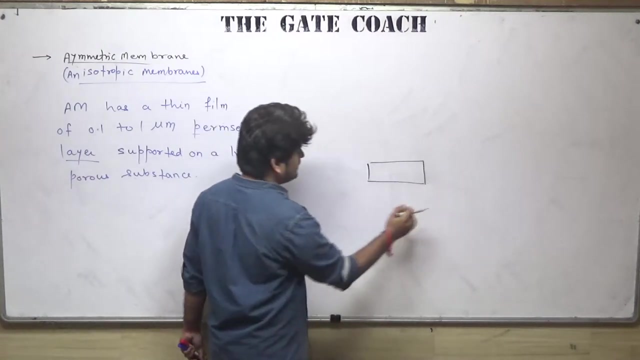 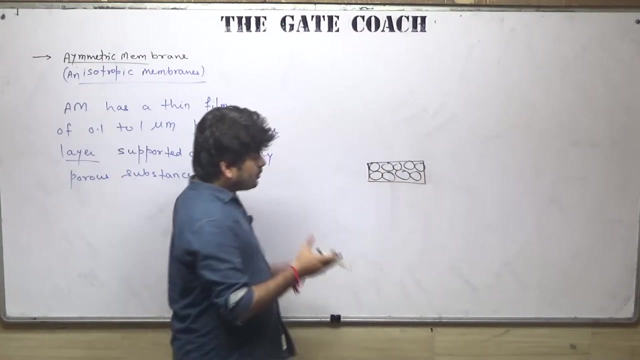 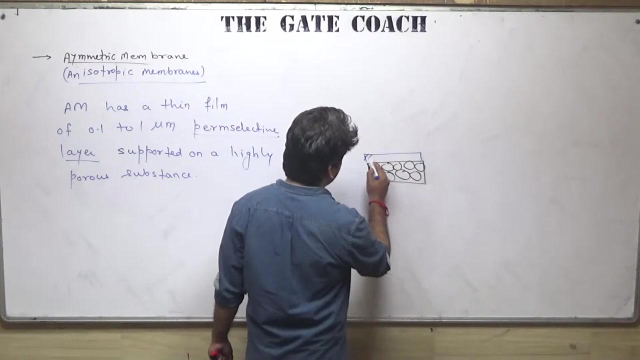 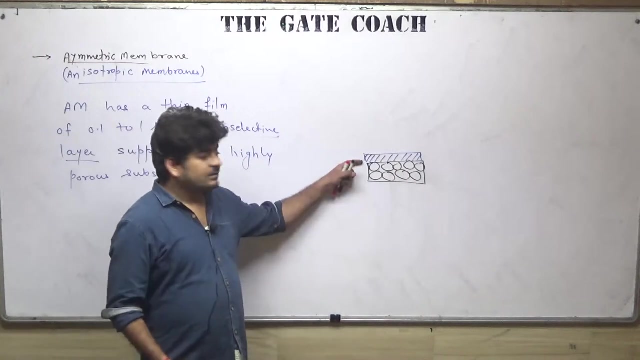 Or you can say semi-selective Okay. layer supported on a highly porous substance means- suppose this is some support which is highly porous. okay means a very large size pores are there. so on this support we place a thin layer, that is, the asymmetric membrane, where a thin layer okay, which allow the passes. 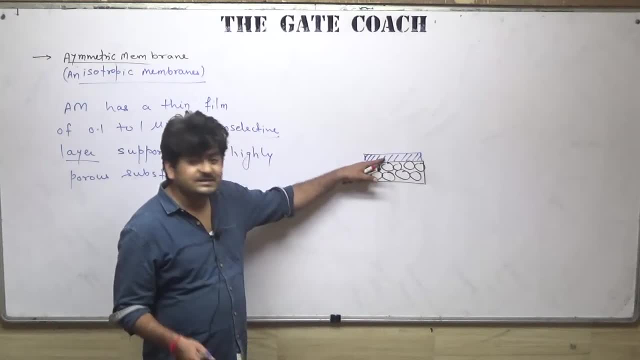 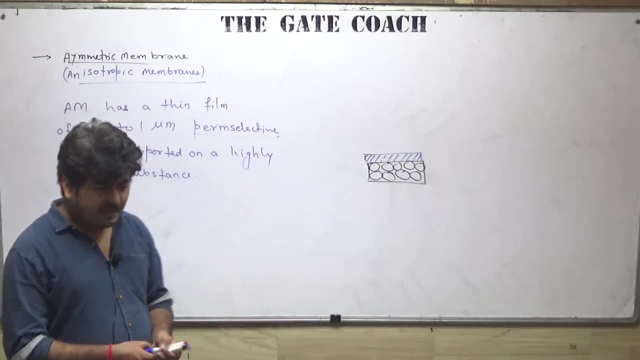 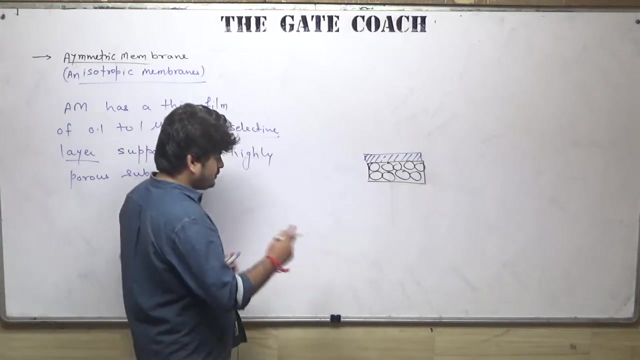 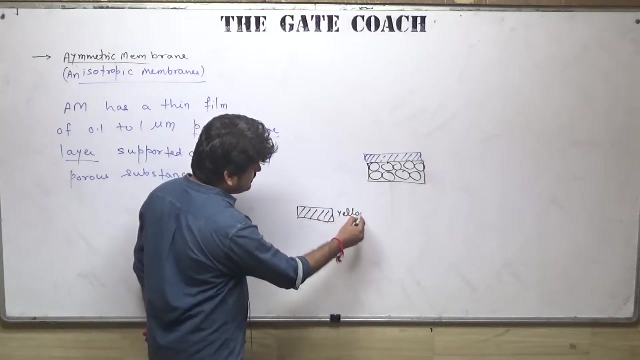 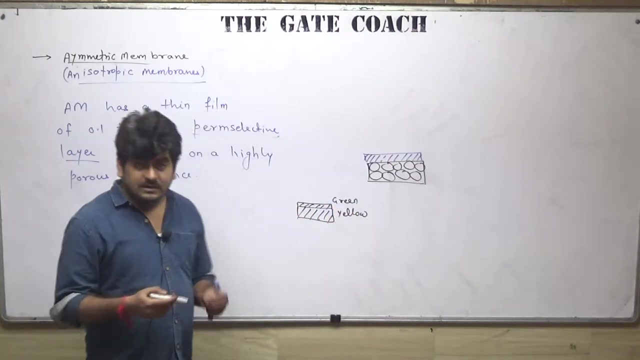 to the selective components only, and this layer is supported by this porous module, porous substance. okay, for example, if you see the sponge which we use in the kitchen for dishwashing, the bottom part is yellow, yellow in color and above this, a green color, green color layer. okay, a film of green color means what we call it, a scratch bright. 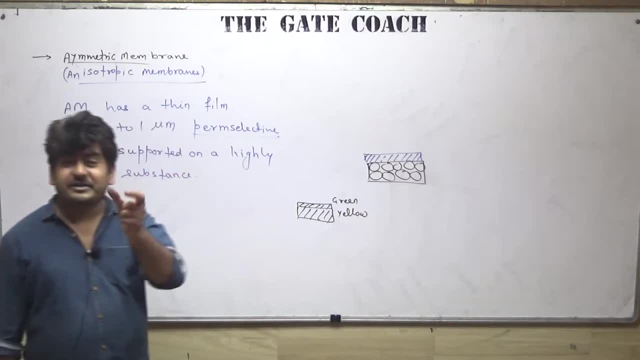 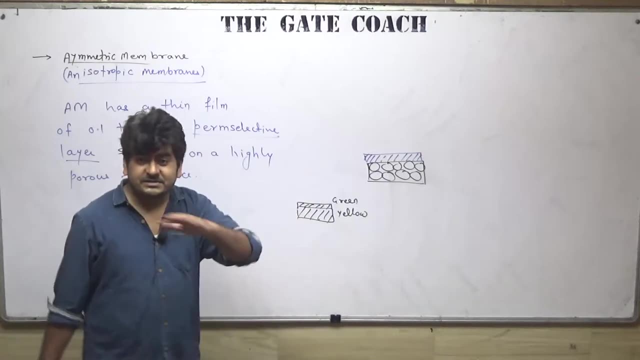 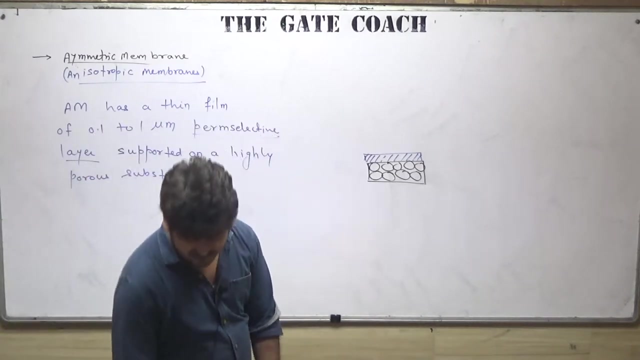 that is a brand. that green color layer is there, green and yellow combination. so, just like that, yellow part is the support, green part is the thin layer which, anyways, i think you must have understood those who go to the kitchen, they must have understood the general dishwashing. there is no problem, okay, so asymmetric membranes. 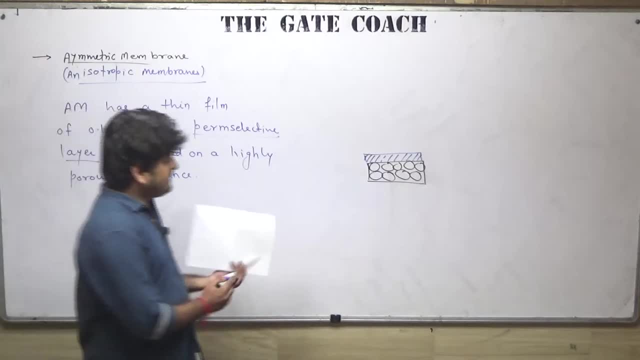 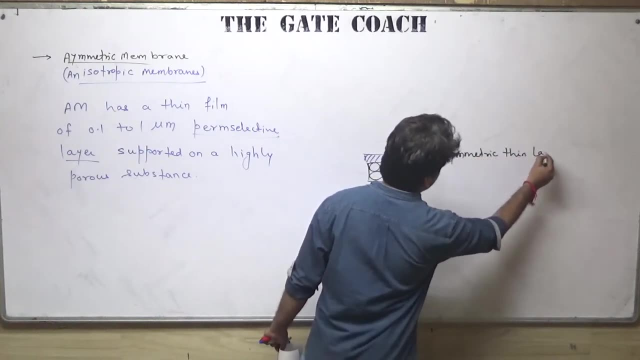 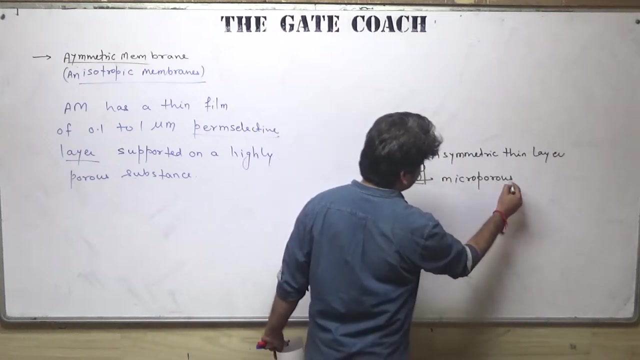 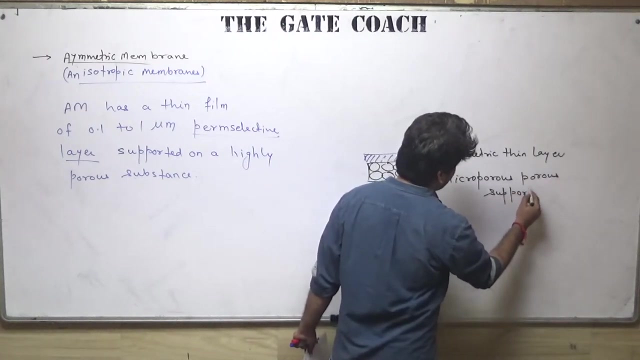 we have several types of asymmetric membranes. okay, and if i talk about this, so this is the asymmetric membrane, this is the thin layer and this is the porous support and most of the, in most of the cases, this support is microporous- means the pore size in microns. 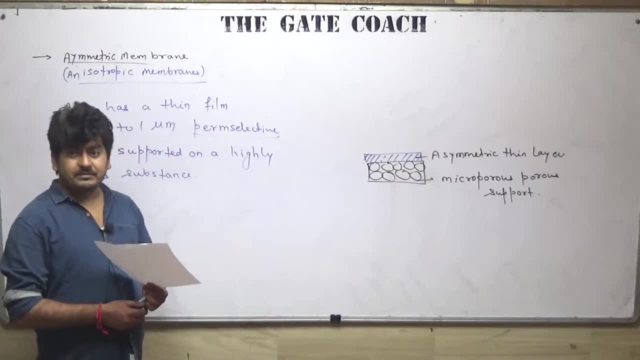 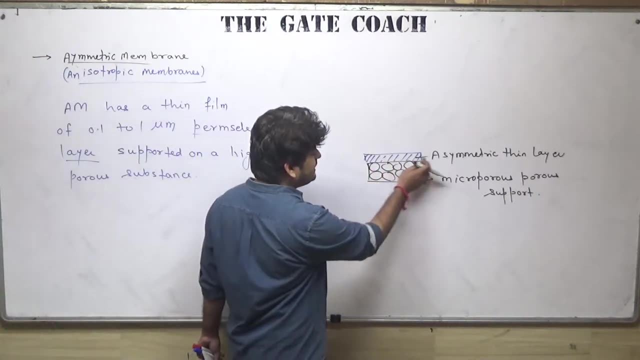 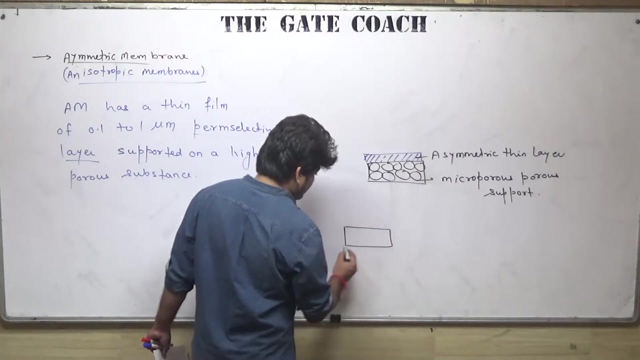 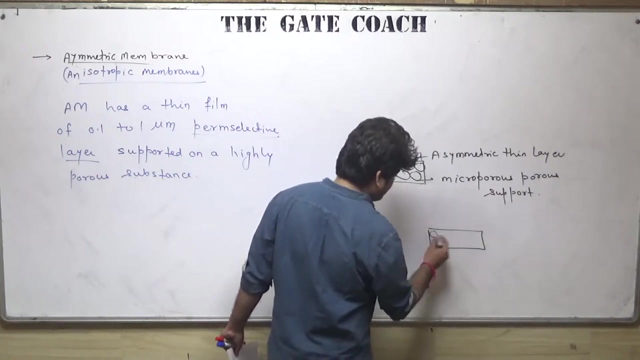 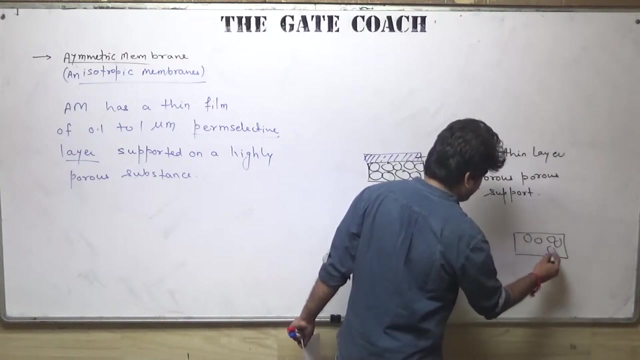 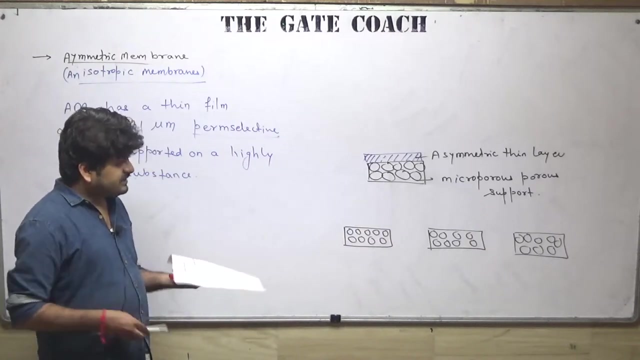 in asymmetric in in asymmetric membranes. we have three types of structures. okay, based on the quality of this thin layer, we have three possible arrangements. first, let me draw the support to, this is the micro porous support and if i talk about the thin layer, okay, so that thin layer can. 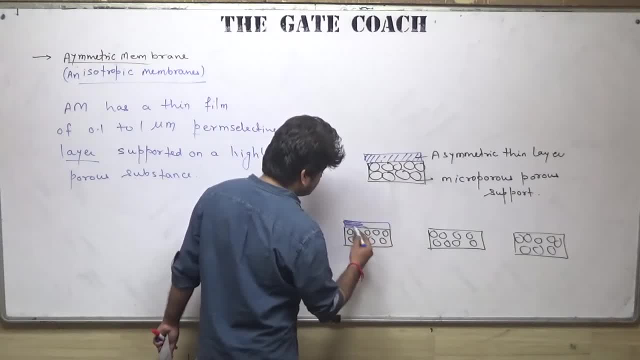 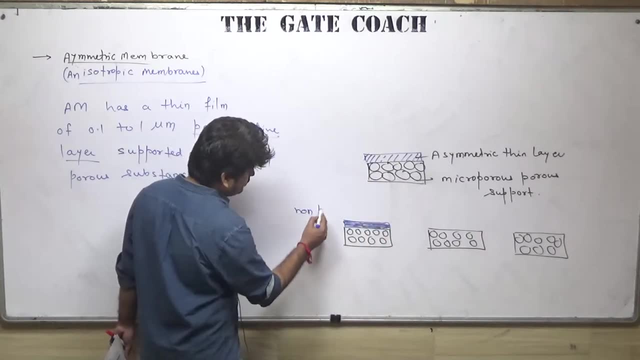 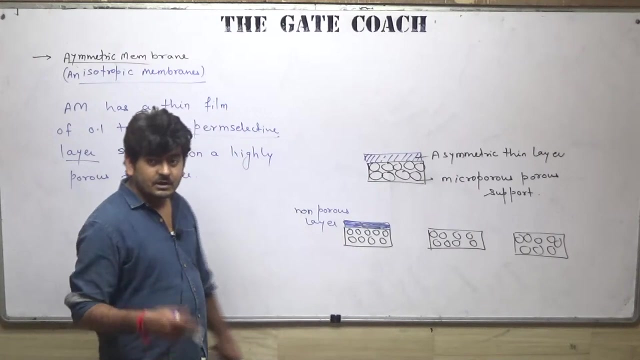 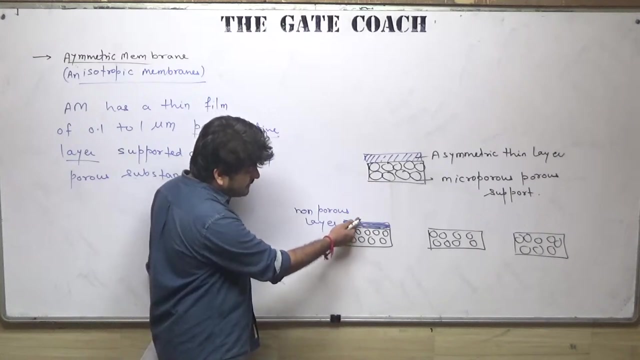 be a thick solid, basically the non-porous layer or the dense layer, non-porous layer on a porous support. so what will happen? selective component feed will go from this side. selective components will absorb in this layer, will diffuse and they will leave in this porous side and 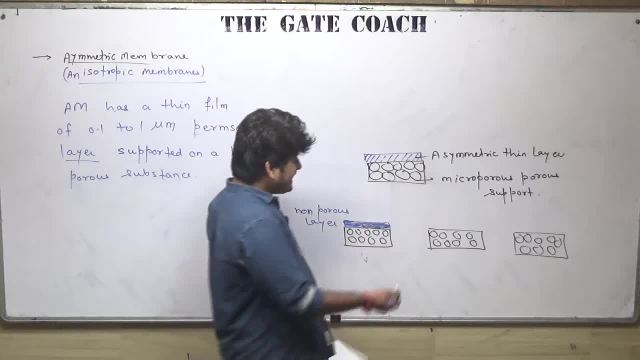 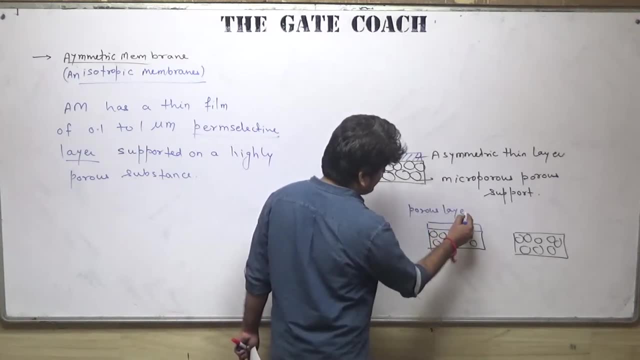 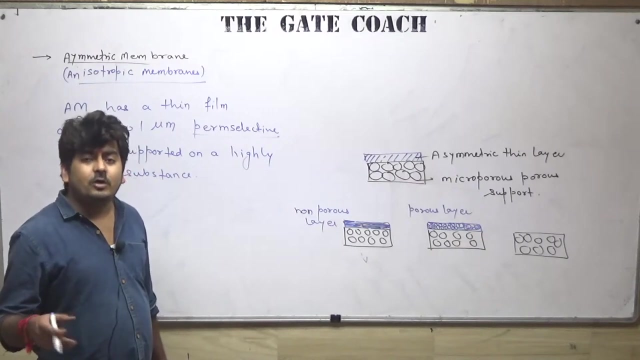 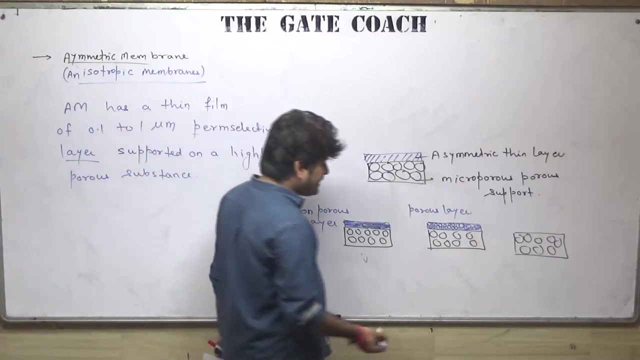 and then here we will get the permeate. second is the porous layer. okay, means this thin layer has some pores in this and the pore size may be uniform or non-uniform. in this thin layer the pore size may be uniform or non-uniform, that depends. okay, otherwise, if you combinely see in the micro porous support, the pore size is: 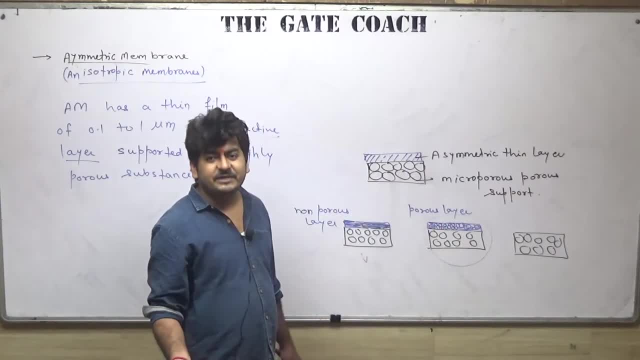 large and in the thin layer pore size is small. so that is asymmetric membrane for your guys. okay, and in this thin layer, if i talk about these pores, it could be uniform or non-uniform. similarly, in this porous part, this pore size can be uniform or non-uniform. that is that depends. 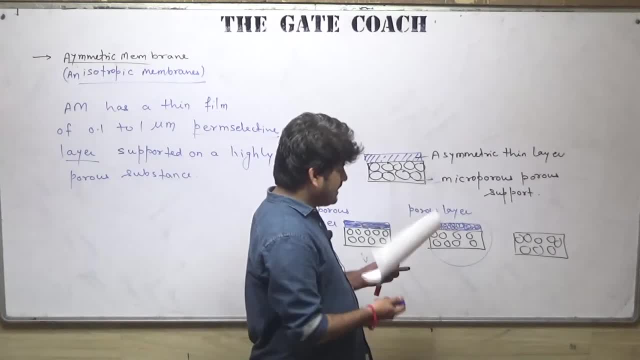 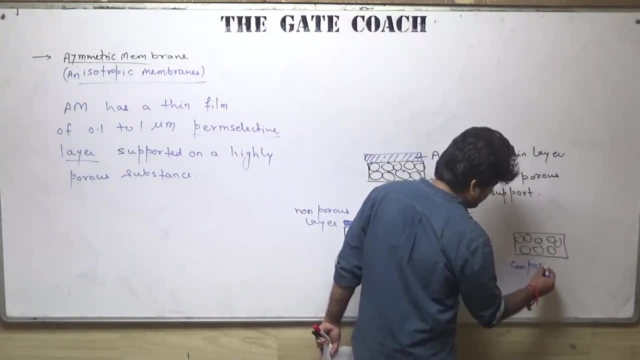 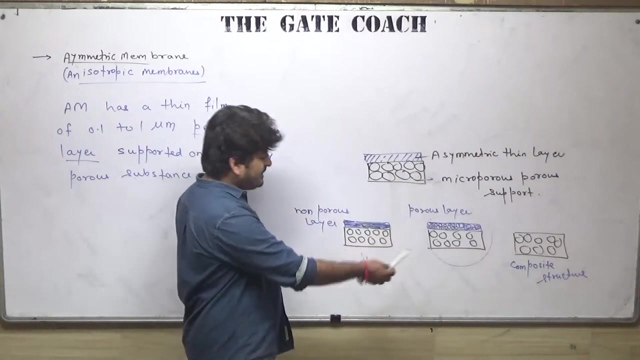 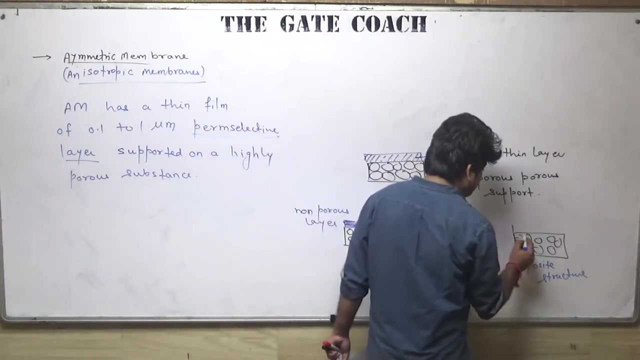 and the third category is composite structure. the composite structure, what is composite structure? that is the combination of these two. for non porous and porous layer. okay means in this thin layer, in first half, that will be non porous, or you can say dense layer is there, and in the second part of this thin layer that will be porous, non porous. 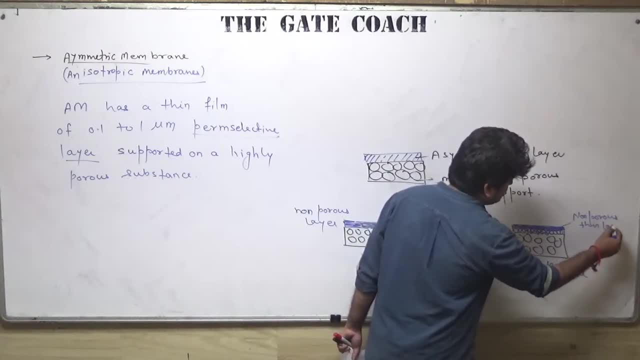 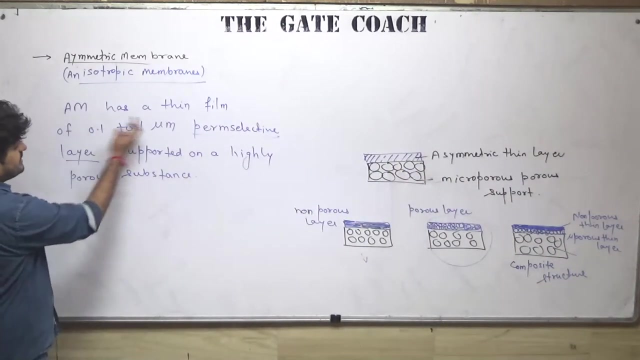 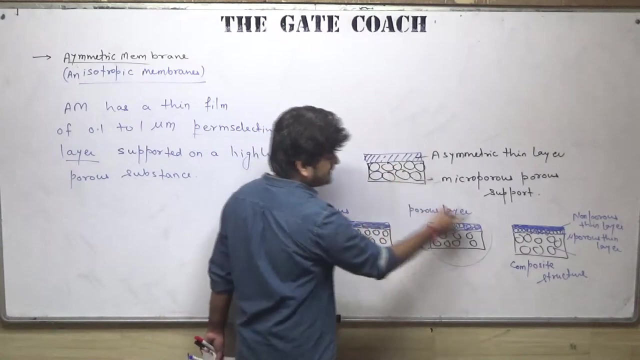 thin layer and this is porous thin layer, basically the micro porous thin layer, and this is the support which we have. okay, so this is a asymmetric membrane, guys, which has a thin film of 0.1 to 1 micrometer permselective. the size of this, the thickness of this thin layer is about. 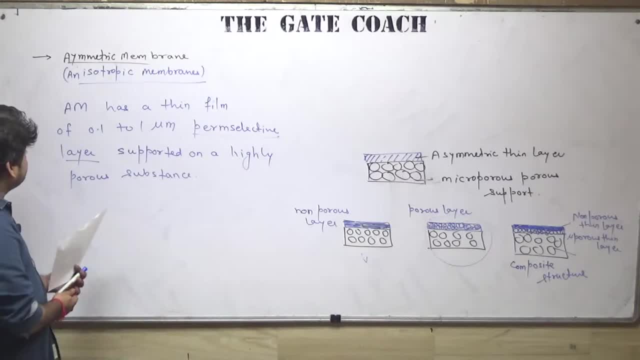 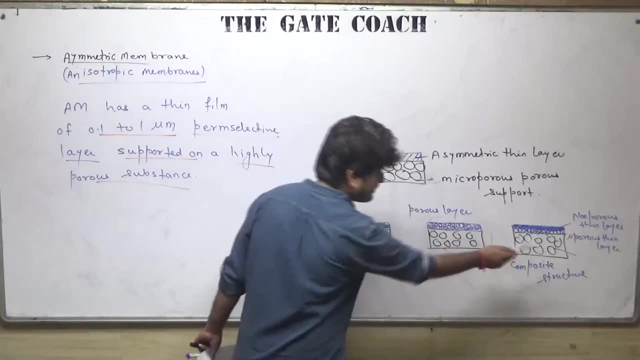 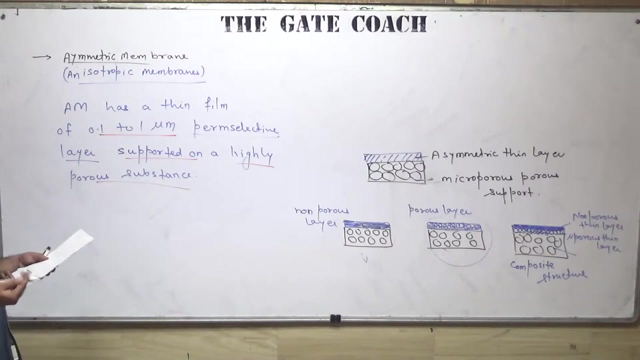 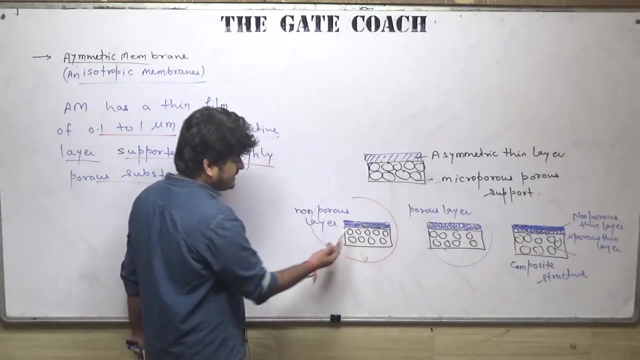 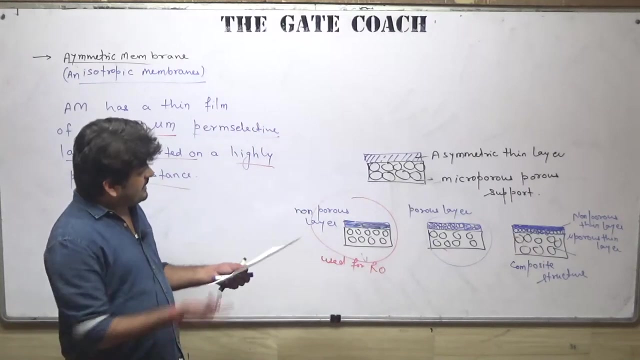 0.1 to 1 micrometer, okay, supported on a highly porous substance. that is asymmetric membrane for you guys. and if I talk about the uses, so this asymmetric membrane can be used. if that thin layer is non porous, then it can be used for reverse osmosis operations. if this thin layer is porous, then it can be used in. 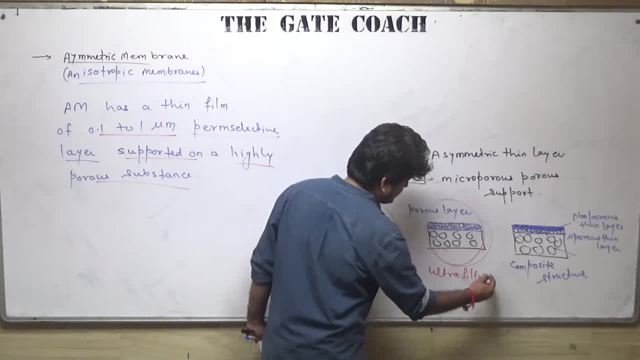 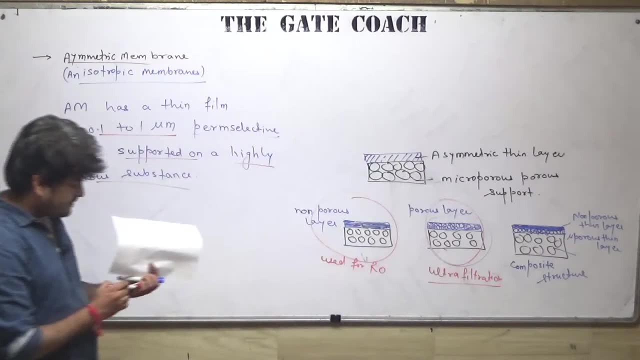 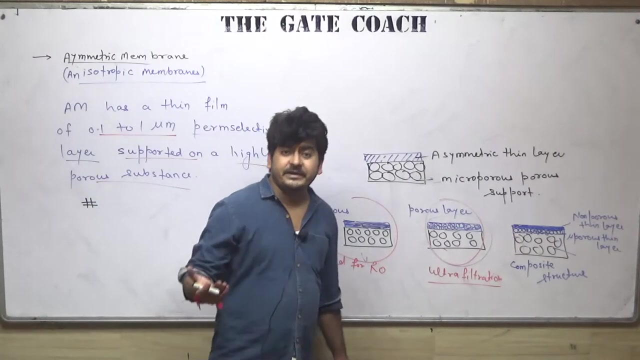 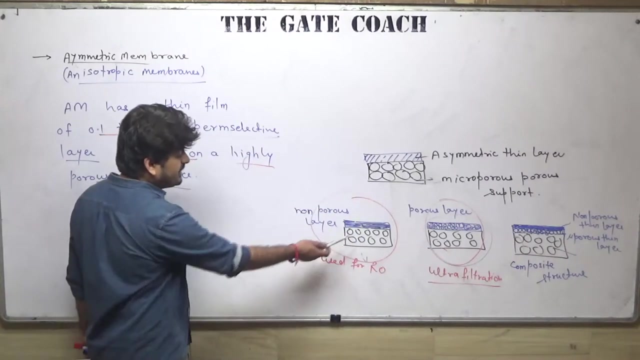 ultra filtration operations. okay, guys, so this is asymmetric membrane flame this or, in extr Portugal, this can be used in Myur injured أي lwo eless. asymmetric membrane for you. I talk about the bookish language. then these two terms, articles, and if you have to define asymmetric membrane to any one, 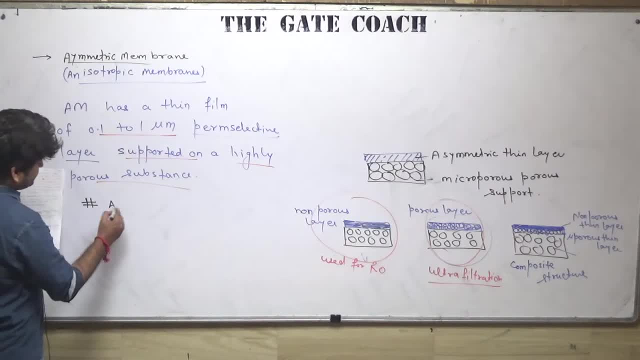 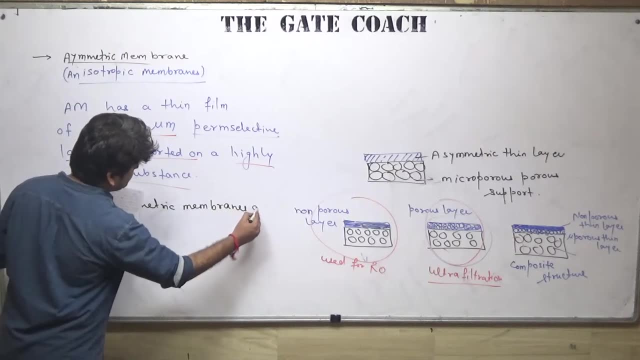 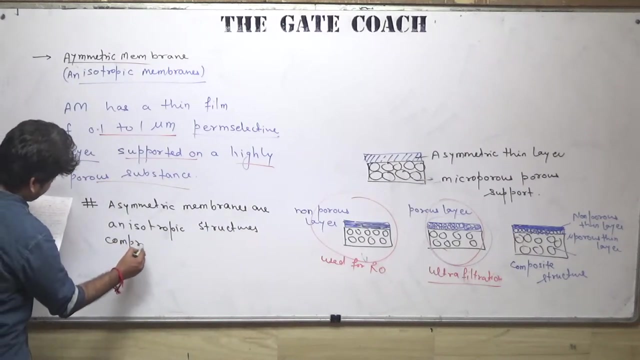 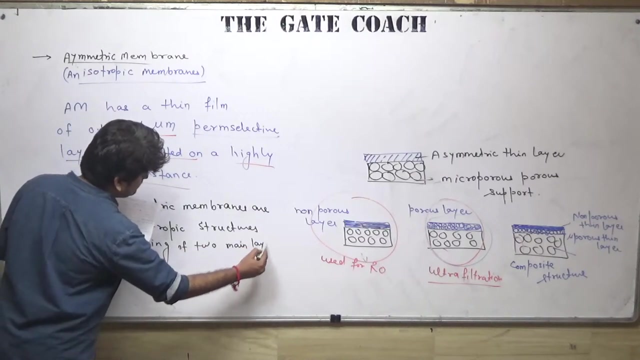 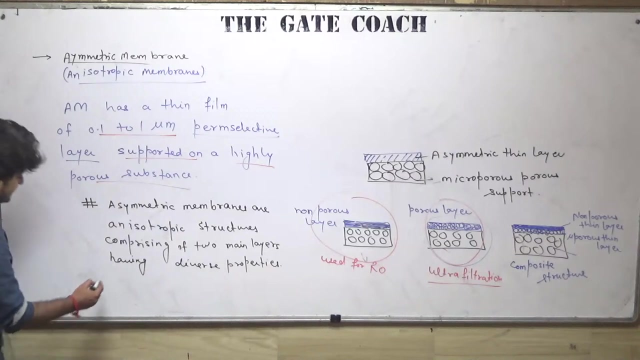 then you can define asymmetric membrane as the combination of two layers. okay, having different. asymmetric membranes are anisotropic structures comprising of two main layers having diverse properties. this means various type of properties are there, such as morphology, that is, the upper layer, the thin layer known as morphology. 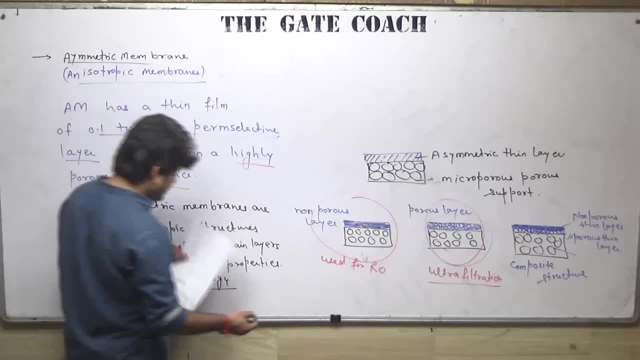 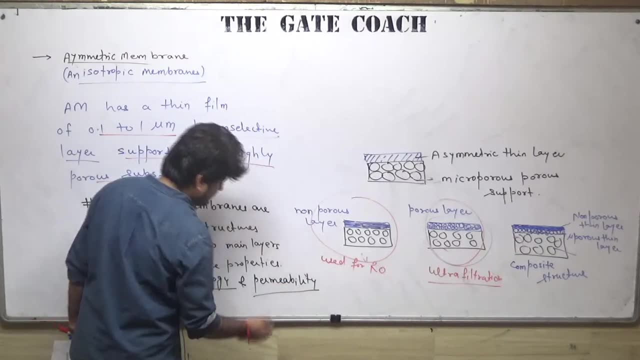 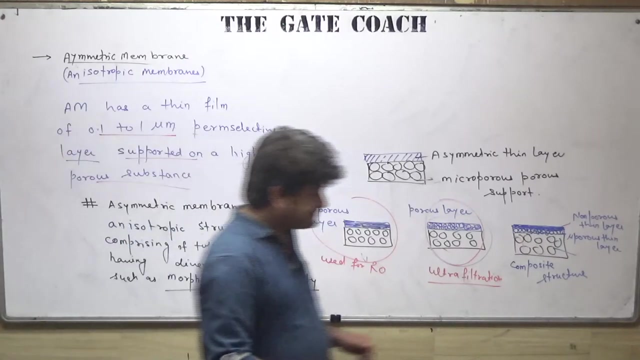 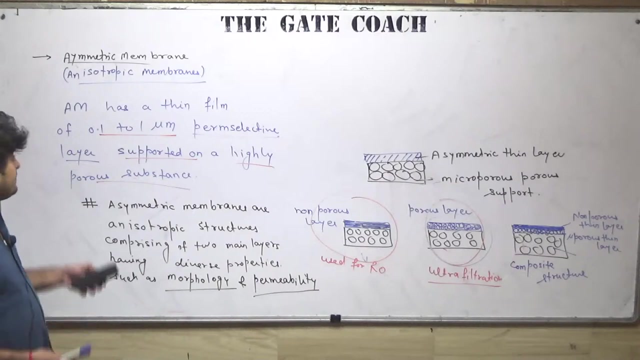 and the bottom layer And the support is known as permeability. So this is a symmetric membrane for you guys. Okay, next we will talk about the composite membranes. So if I talk about the composite membranes, So composite membranes are basically the combination of: 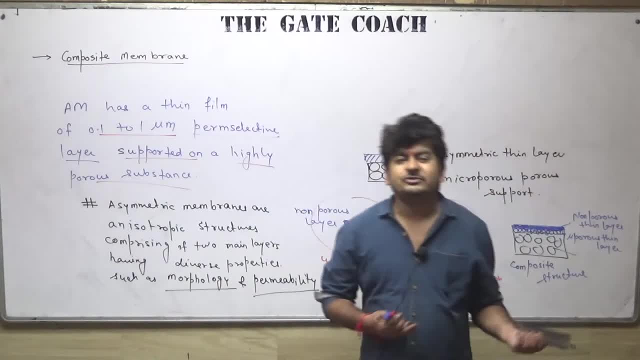 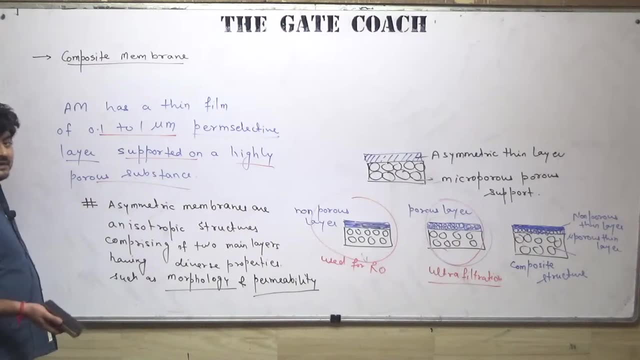 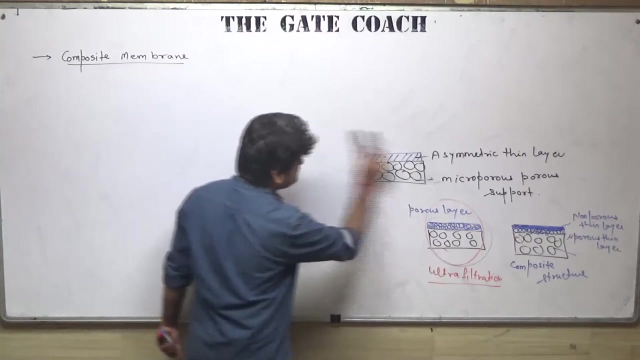 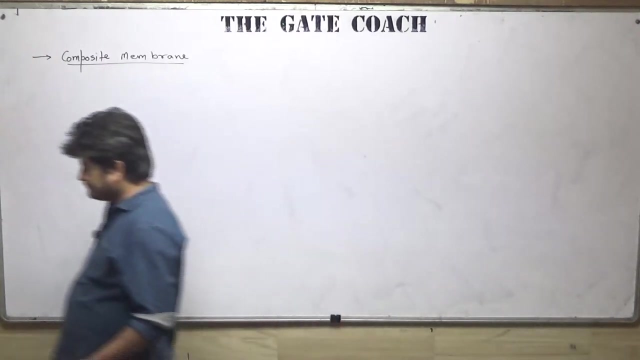 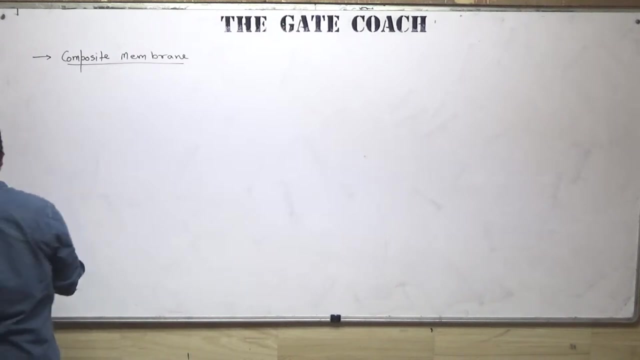 symmetric and asymmetric membranes, isotropic and anisotropic membranes. Okay, what are those? How can we define the composite membrane? What is the applications and all these things? Let's try to understand this. Functionally, these are similar to asymmetric membranes. 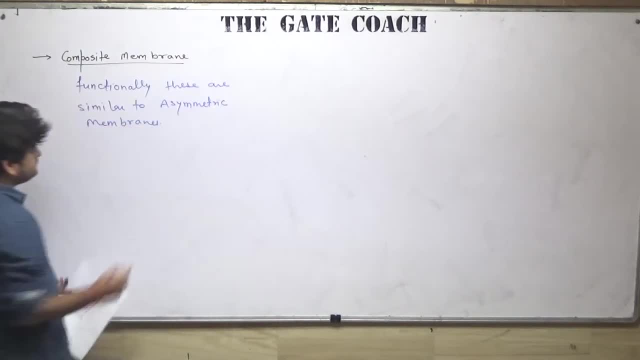 Okay, so how can we define the composite membranes? That is a point, So that you can define like a composite membrane. See, if you see any book or any literature, you will not find the points, relevant points, about the composite membrane as such. 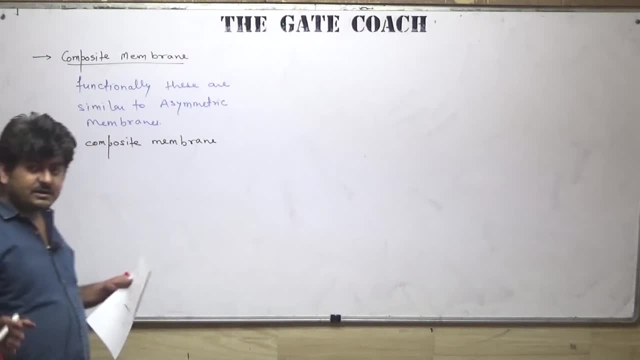 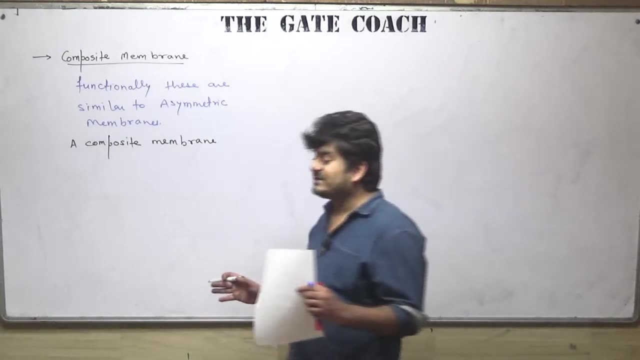 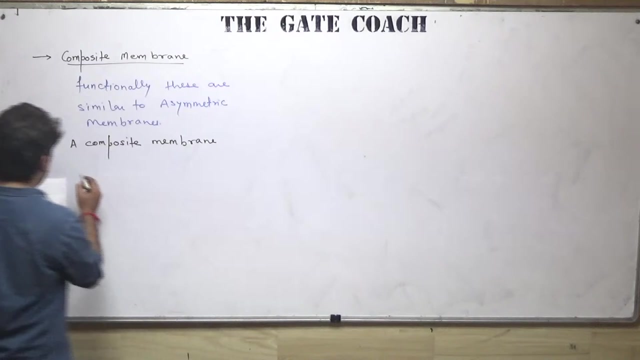 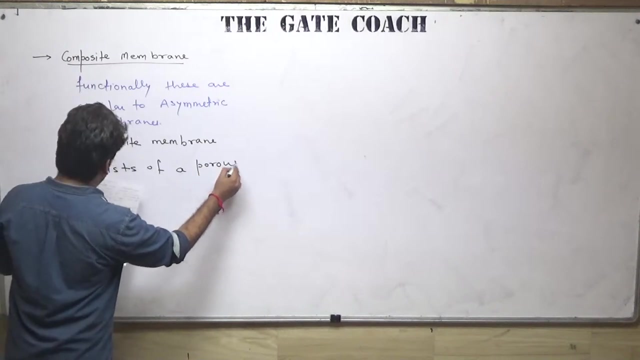 Okay. In every book which I have seen composite membrane, they have explained this only in 3-4 lines. That's it Okay. So there are some points which you should understand. A composite membrane consists of a porous or dense, thin membrane. 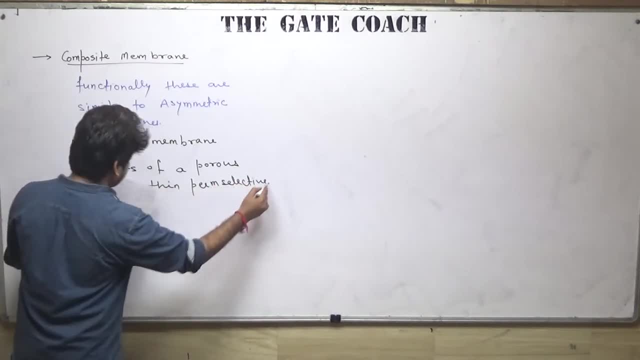 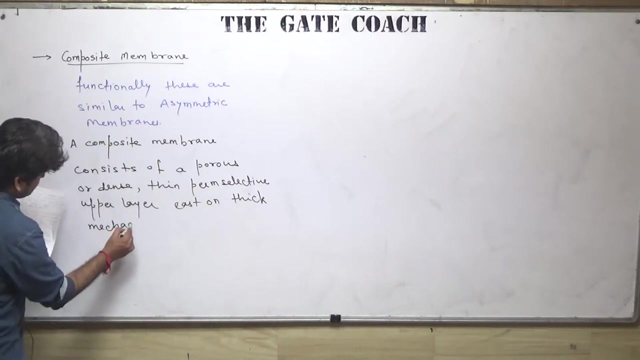 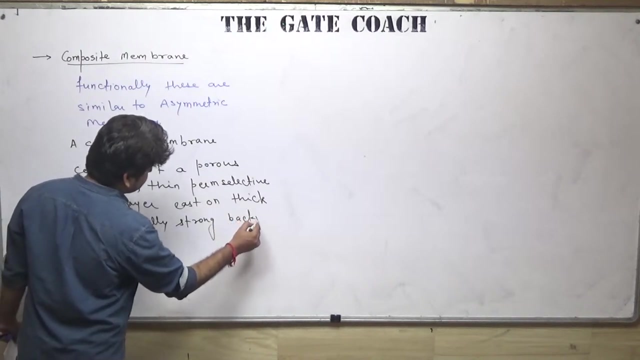 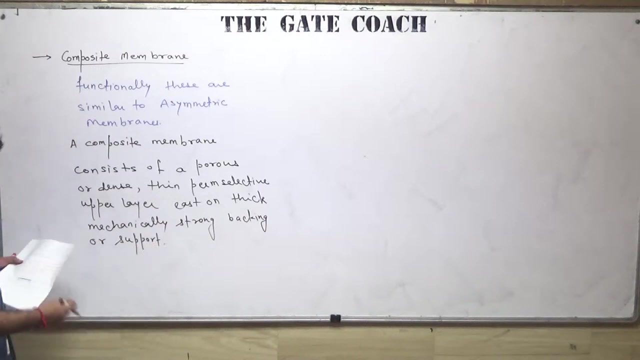 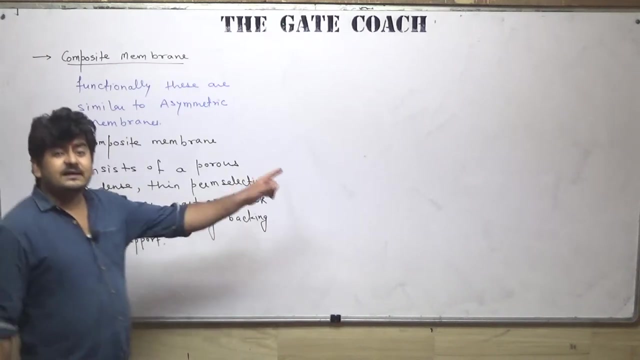 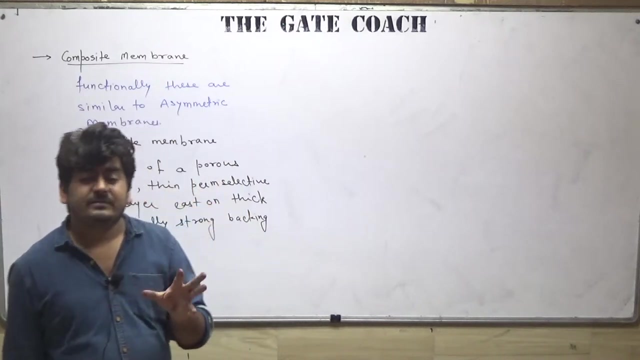 Perm-selective upper layer cast on a thick, mechanically strong backing, or you can say support. Okay, In asymmetric membrane, the thin layer and the bottom support they most of the time they have. they are made up of same material, Okay. 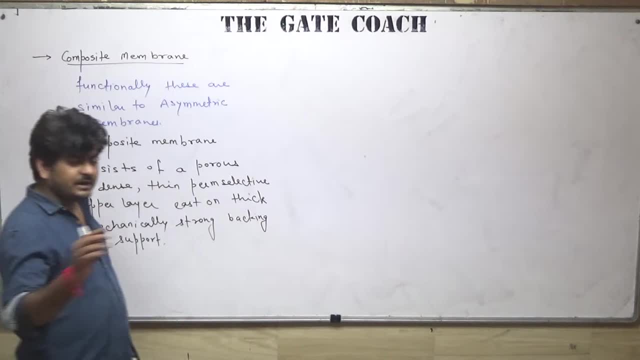 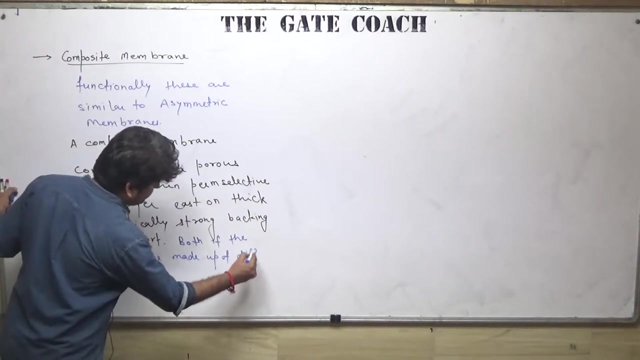 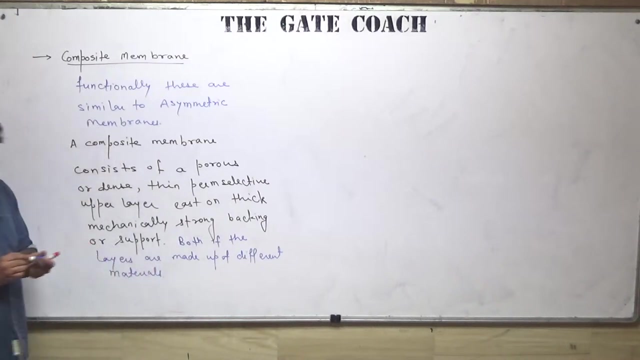 Only there are few examples where, in asymmetric membrane, the thin layer and the porous support is made up of different material, But when we talk about the composite materials, then both of the layers are made up of different materials. Okay, So what is the composite membrane look like? 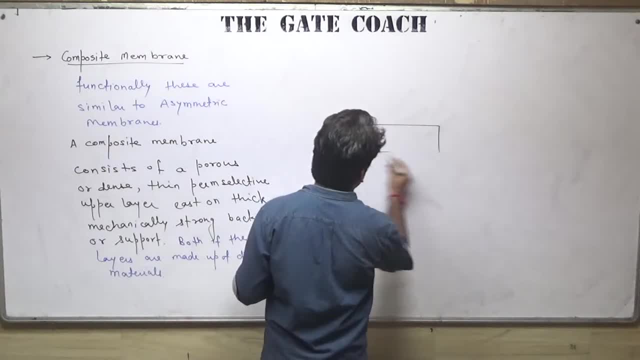 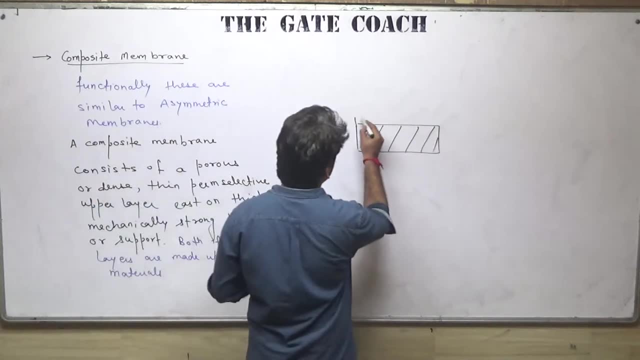 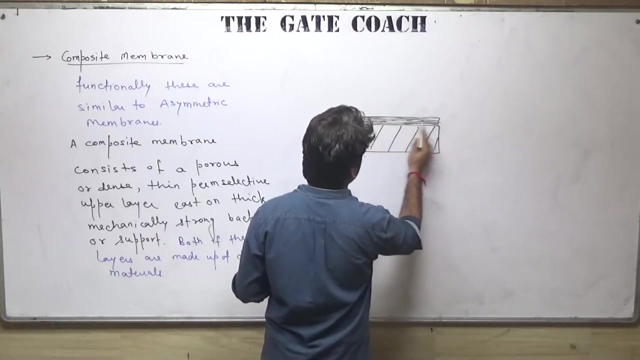 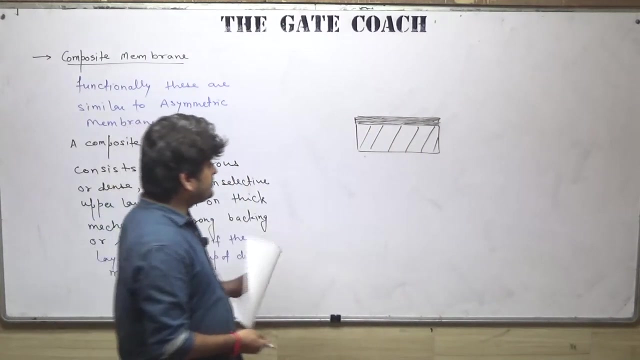 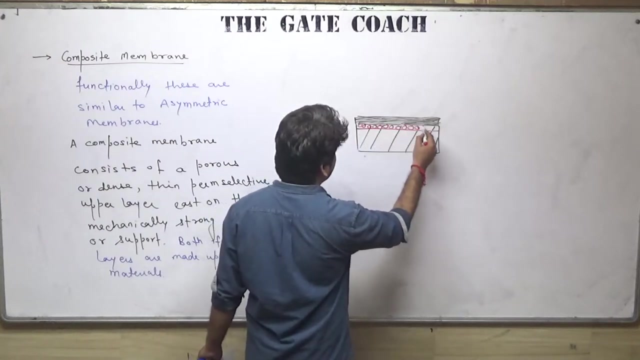 So composite membrane. you can see, this is the support which we were talking about On this. there is a membrane, a thin, non-porous layer, And just below this thin, non-porous layer, there is a porous structure. Okay, 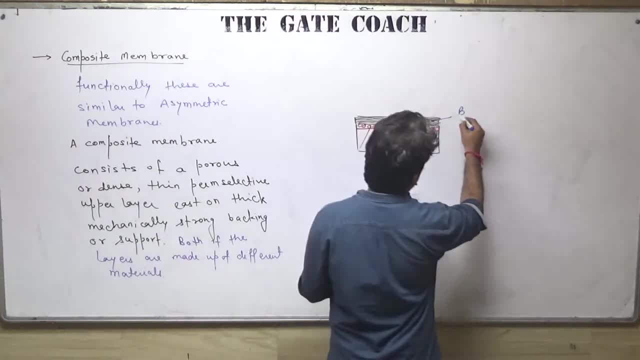 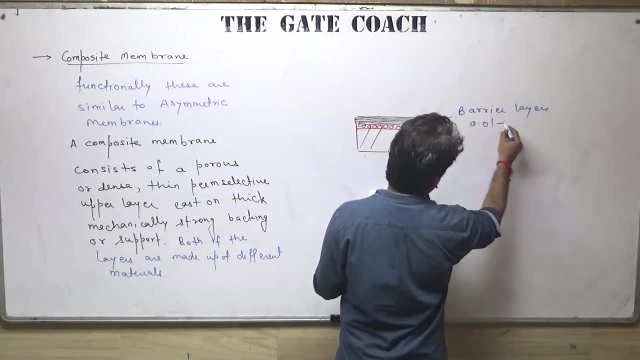 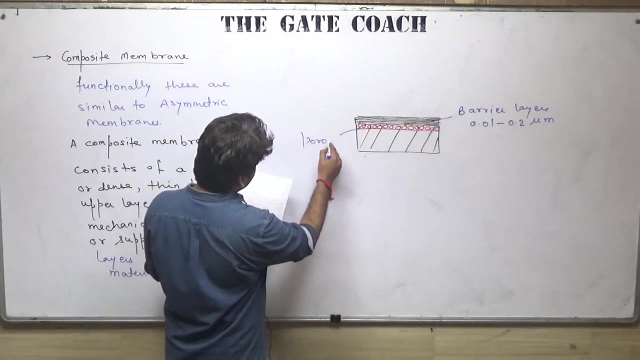 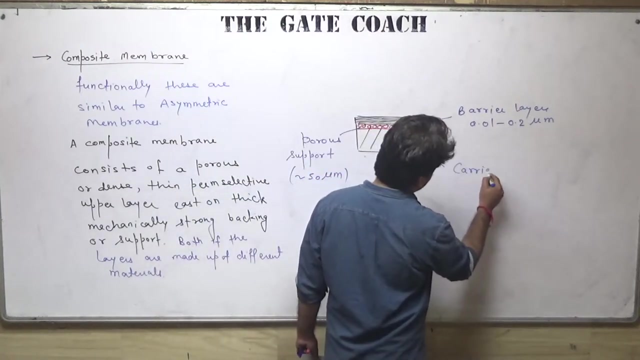 Where this non-porous layer is also known as barrier layer. The size of this layer is approximately 0.01 to 0.2 micrometer. This is the porous support. The size of this porous support is about 50 micron And this is the carrier material. 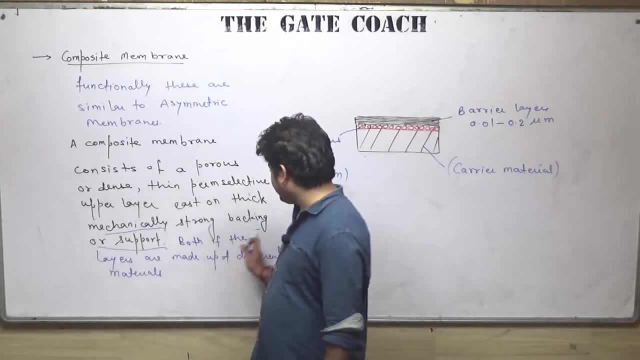 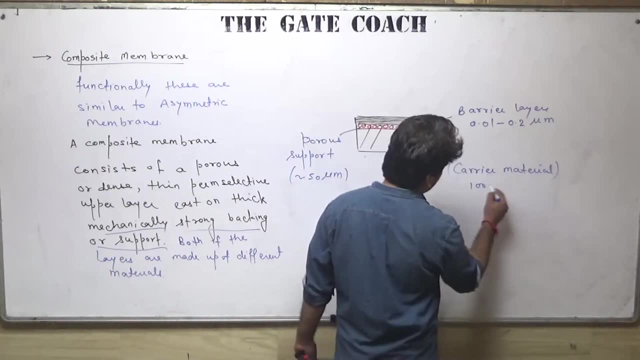 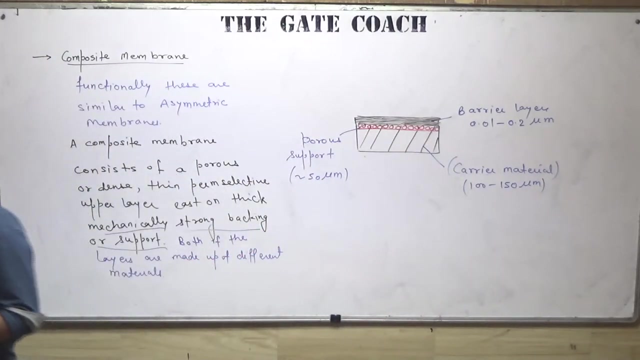 The mechanical support which we were talking about, And the size of this, the size of the pores in this carrier material, is about 100 to 150 micrometer. Okay, So functionally you can see, this is same as the asymmetric membrane. Asymmetric membrane is also a combination of two layers. Composite membrane is also a combination of two layers. But what is the difference? The difference is if I talk about the membranes. in case of thin film, composite membrane, you can say TFC. Membrane flux is higher than that of an integrally asymmetric membrane. Asymmetric membranes Okay. So if I talk about the flux, So in composite membranes flux is higher than that of an asymmetric membrane. Second point: The pore structure. The structure of these pores in the layers. 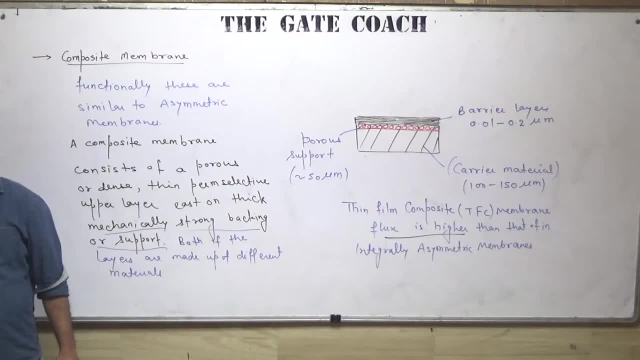 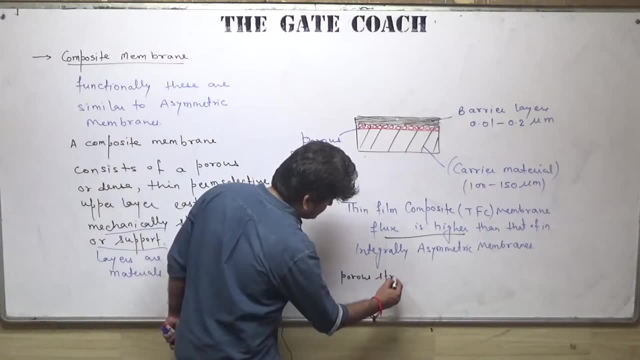 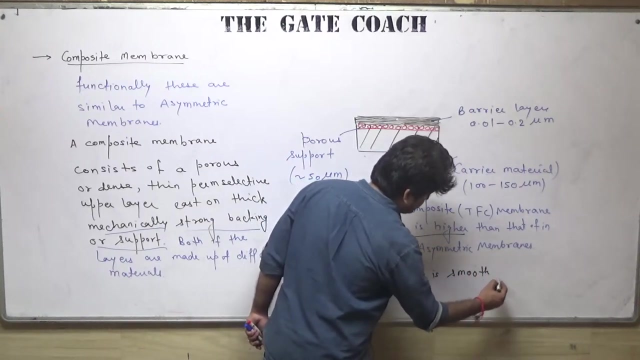 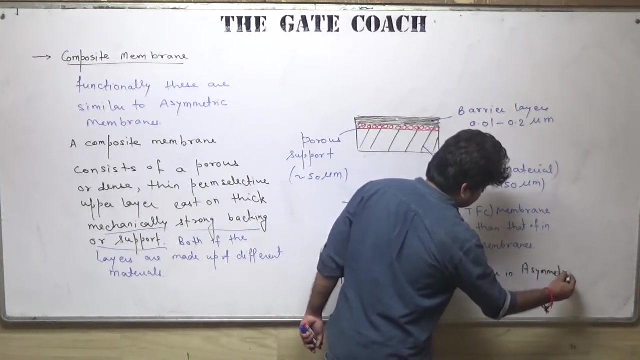 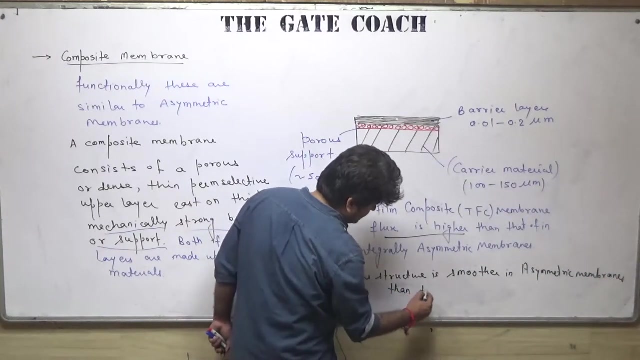 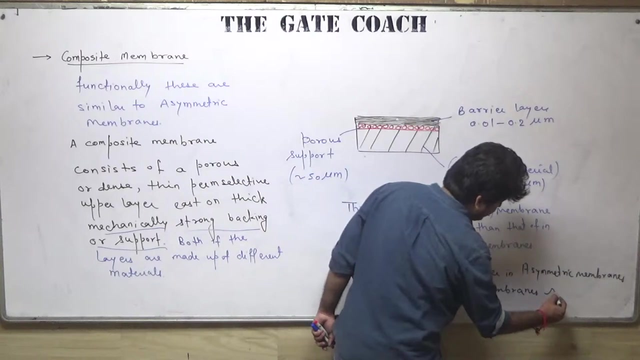 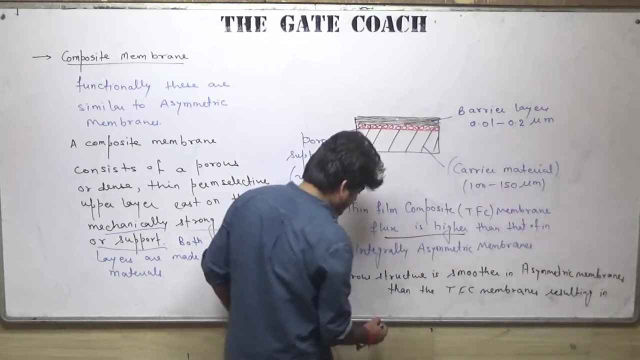 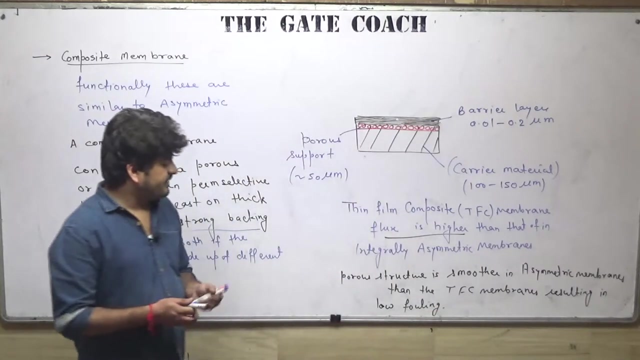 If I talk about that, The porous structure is smoother in asymmetric membranes Then the thin film composite membranes, Resulting in low fouling. We discussed that fouling in the second lecture. Okay, So this is basically the deposition of physical particles, solids, on the membrane surface. 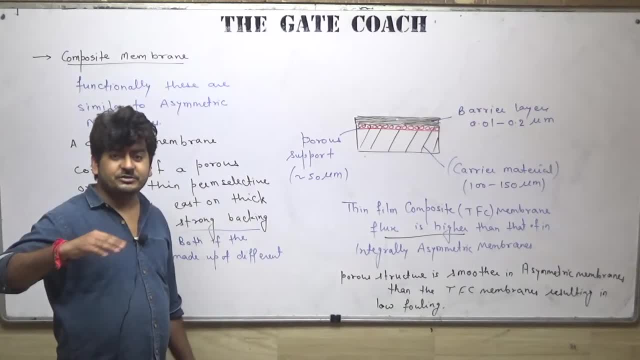 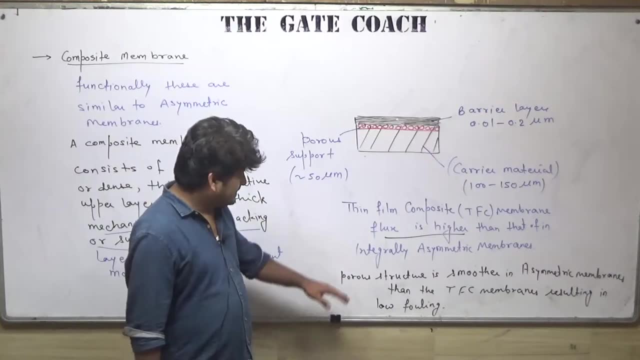 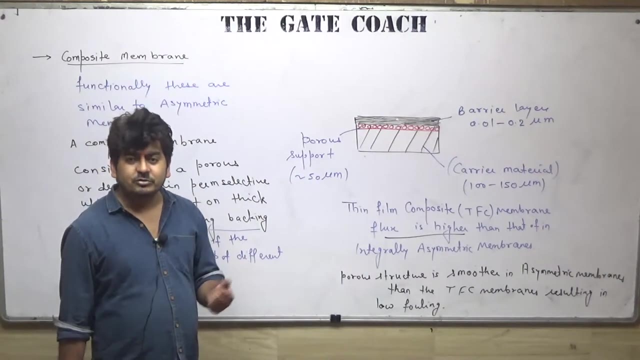 Like dust, particles get deposited on your vehicle when they are in the parking for a longer time. So deposition of the solid particles in the membrane. That is called fouling. So in case of asymmetric membranes the pore structure is more smooth than the composite membranes. 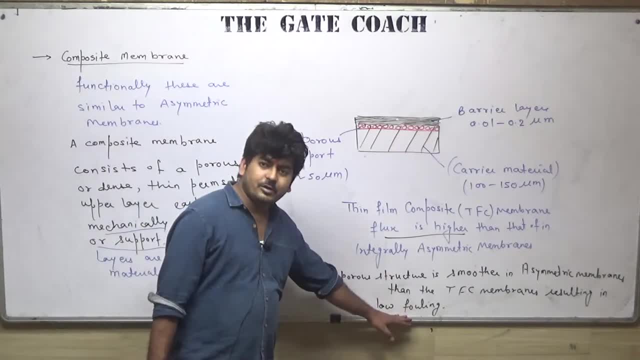 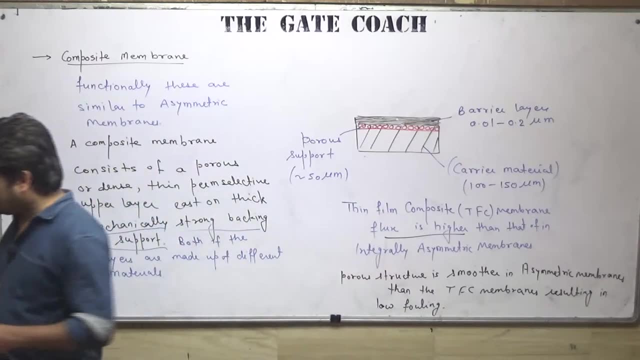 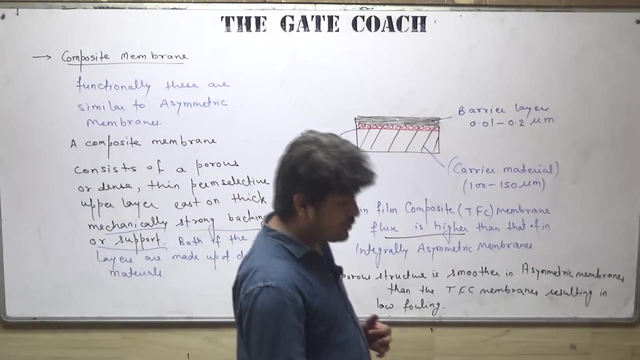 So that's why the fouling problem, The fouling problem in asymmetric membrane is less As compared to that of in composite membranes. Okay, So both of them have their different advantages and disadvantages. Okay, So this is something about the composite membrane guys. 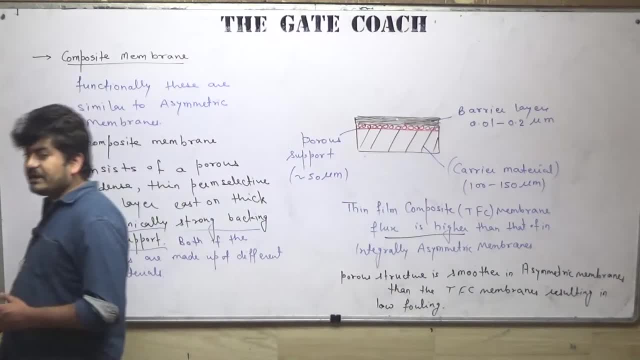 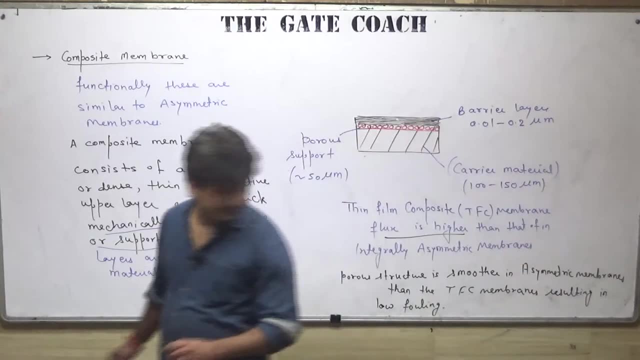 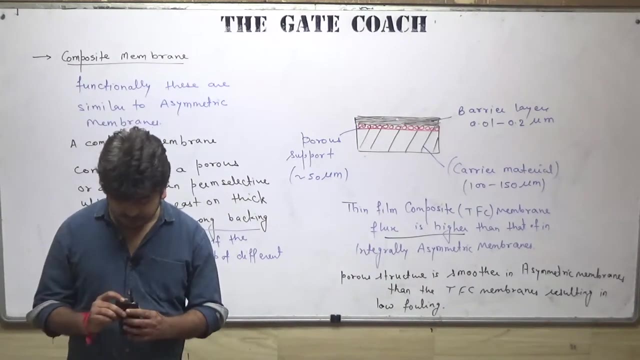 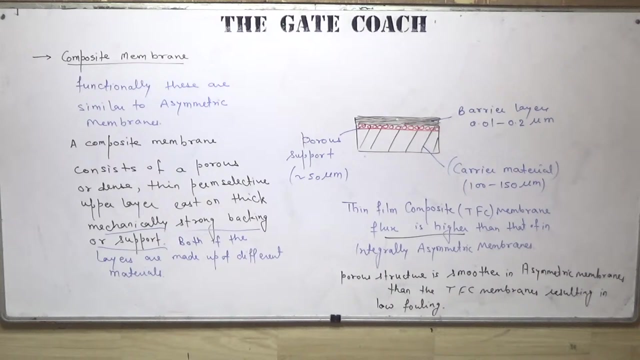 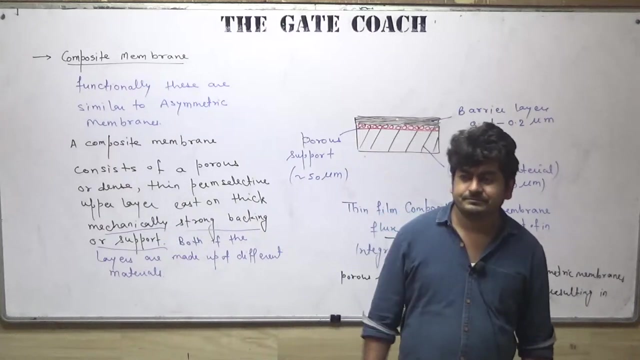 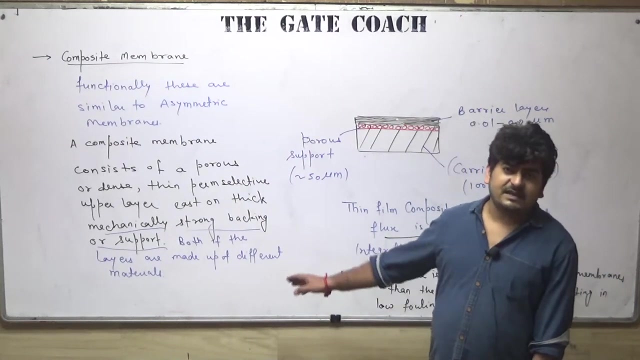 Next we will talk about the inorganic membranes and liquid membranes. Guys, I will share the handout about the liquid membranes in the next lecture. Okay, Thank you. We will talk about the liquid membranes and inorganic membranes to you in the telegram group. 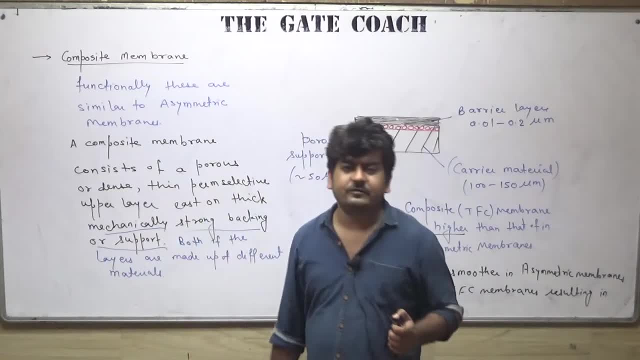 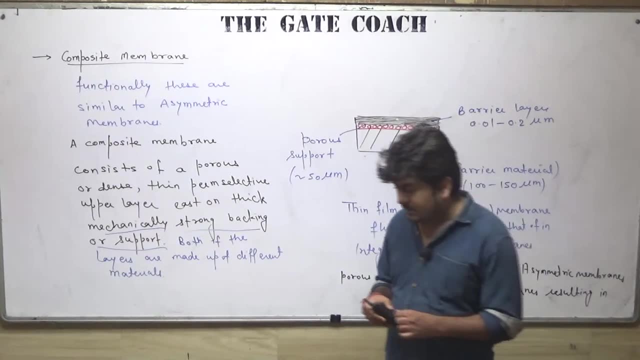 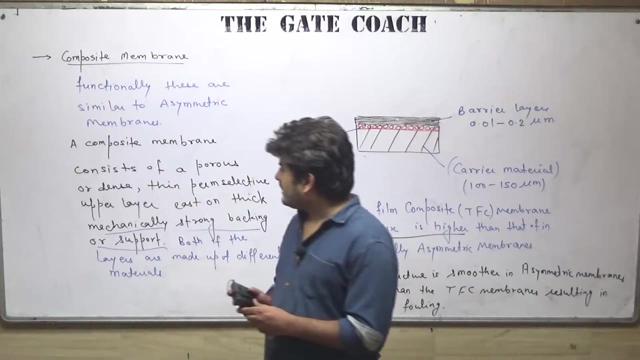 Unfortunately, we have to stop this class right now because we have some work to do. So see you in the next class. The timing will be shared to you till tomorrow, or maybe day after tomorrow, when we will have the next class, And then we will discuss about the characterization of membrane. 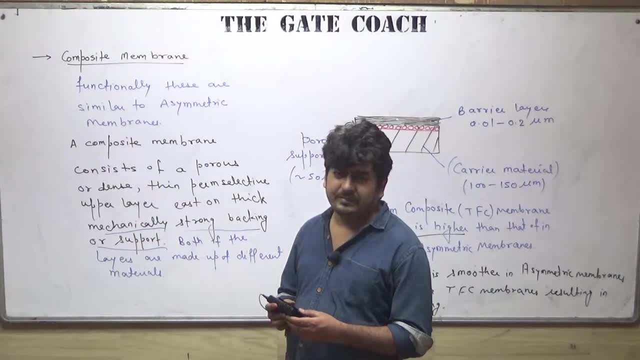 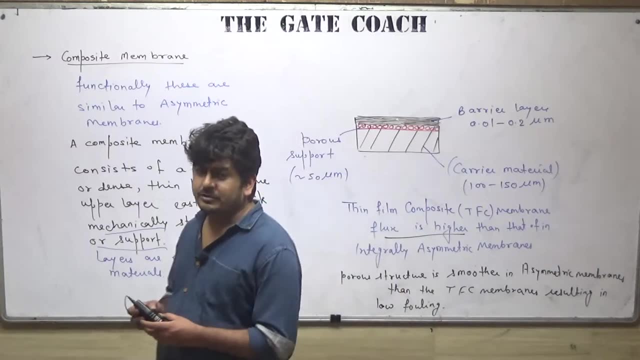 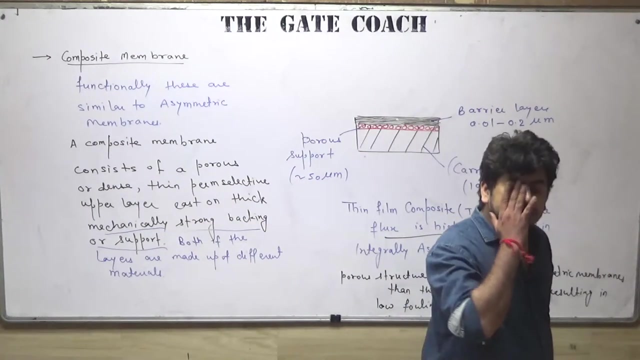 Transportation of membrane and the five main modules of the membrane: The spiral bound module, the cylindrical module and all that. Okay, See you guys. Thank you for the day, Bye, Bye.